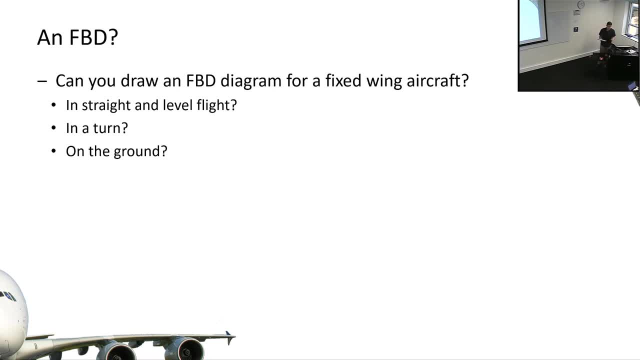 I want you to draw a free-body diagram for a fixed-wing aircraft in straight-level flight in a turn, in a sort of level bank turn, and on the ground. Now I'm not going to give you any more specifics than that. You can make whatever assumptions you like. 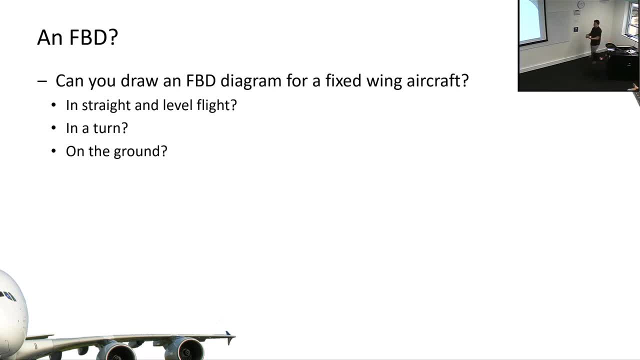 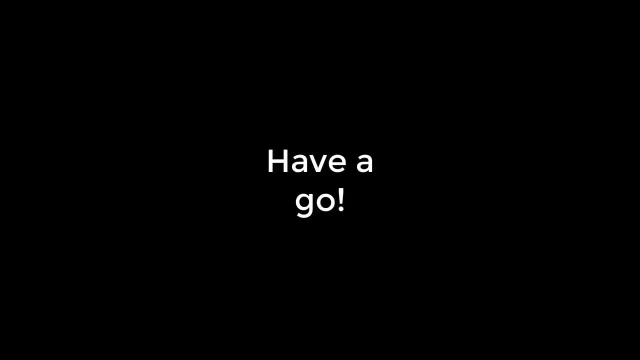 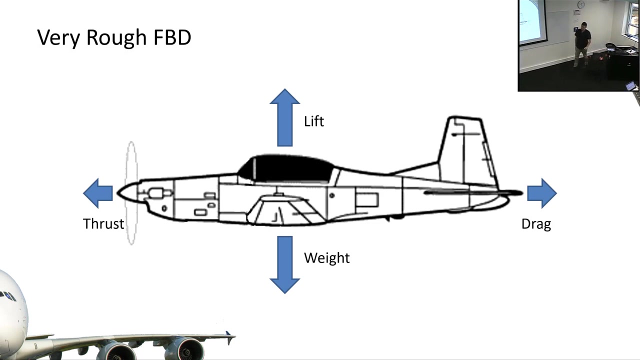 But Have a crack at drawing what you think I'm expecting you. Straight-level flight is something that you'll hear a lot for the next couple of years. Straight-level flight is the kind of go-to condition that we stick an aircraft in when we're trying to think about it and what it's doing in terms of performance and in terms of structures. 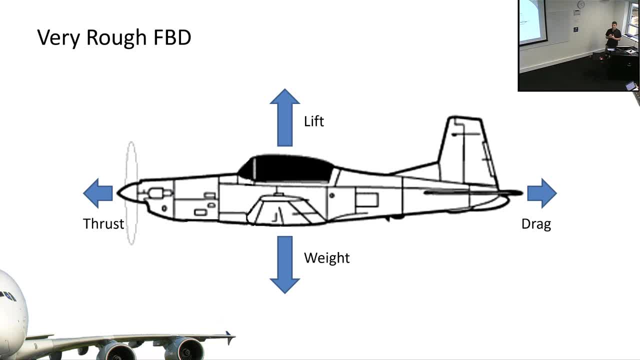 Because from straight-level flight, we can then impose other conditions on it as we see fit. But this is the sort of default state that a cruising aircraft lives in Now. this is obviously a very rough FPD. I've really treated the aircraft as a particle here. 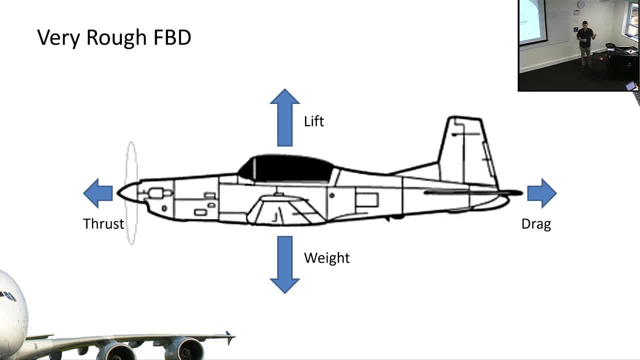 But we have a lift force which you all should be familiar with. We'll talk a bit more about how we generate lift, Primarily not in this course, in the aerodynamics course, But we'll talk about the interaction between lift and weight a lot in this course. 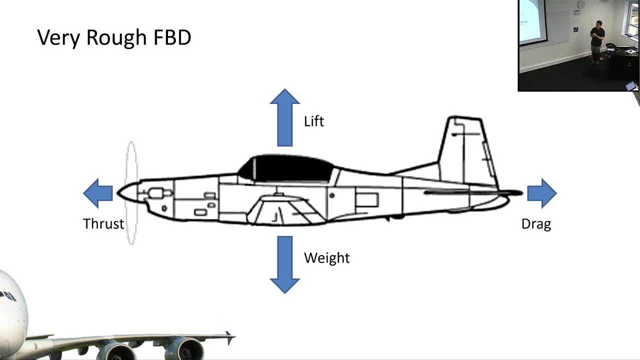 Thrust and drag are equal and opposite in straight-level flight, as are lift and weight. Now, thrust is not at all covered in this course. That's what you'd learn in the flight mechanics and propulsion course. And drag: we don't talk about much either. 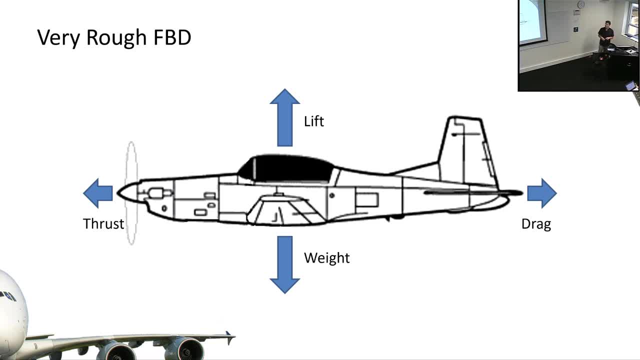 In general, thrust and drag are significantly smaller than lift and weight. So, in terms of the aircraft and the structures that we need, lift and weight have a much bigger impact on the structural design than thrust and drag do in terms of the amount of material we need to carry those loads. 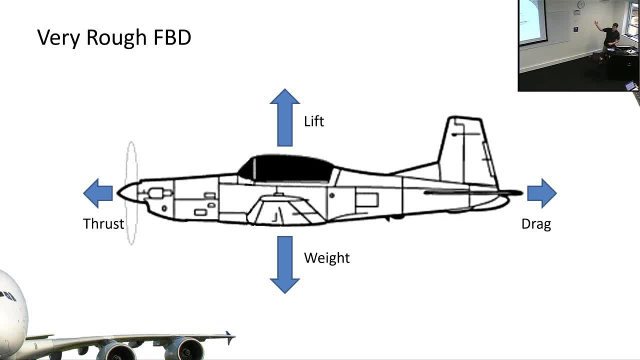 And in straight-level flight there's nothing really interesting happening out of the plane. here There's nothing happening on in and out of the page that's of interest. Now, this from a structure's perspective. how useful is it? This is not really telling us anything about the loads in the airframe, is it? 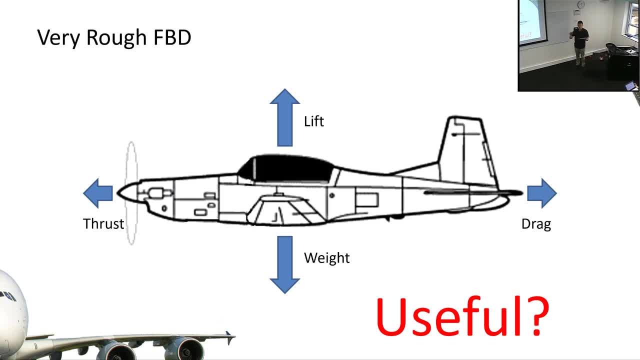 It's telling us a lot about what's happening as a whole to the airframe and to the aircraft, But there's nothing that's going to about this kind of diagram That's not going to going to tell us how much load is in the wing or how much load is in the tail. 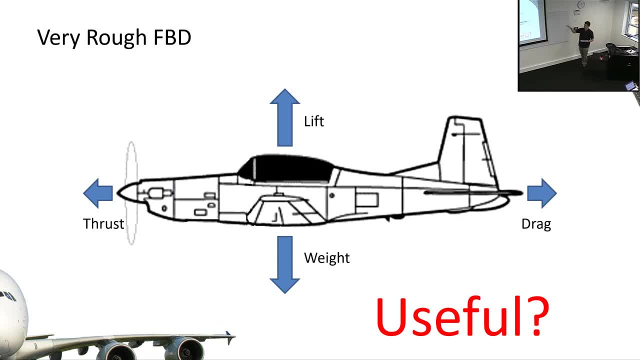 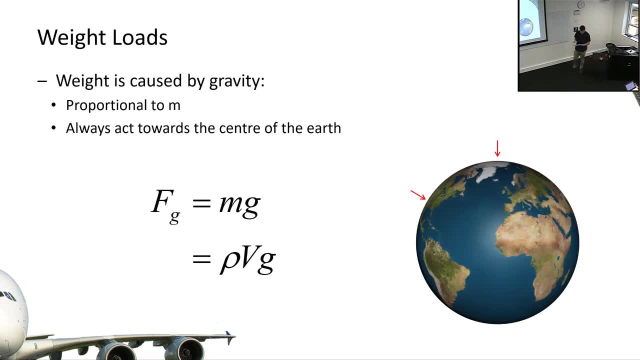 where we're relying on this. this can tell us how this kind of particle aircraft moves around, but it's not going to tell us anything about the structures. so I've got some pictures of the other conditions in a minute, but I won't. I want to take a bit of a side note and talk about these, the nature of some of 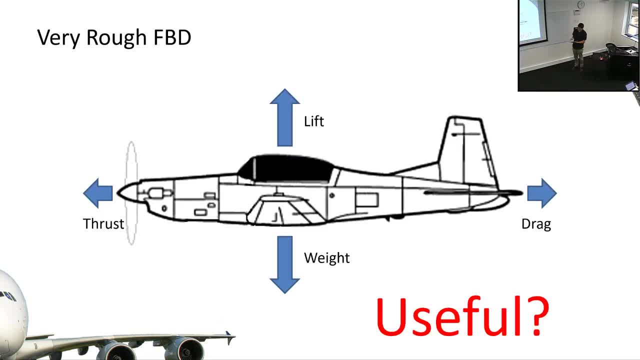 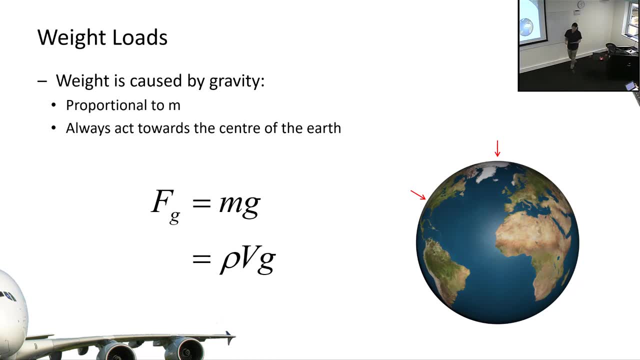 these loads. so if we look at these loads here, weight loads- when we talk about weight, weight is always acting towards the ground and precisely towards the center of the earth, and it's obviously proportional to the mass of the aircraft. and if we're flying around near the surface of the earth, which most of the 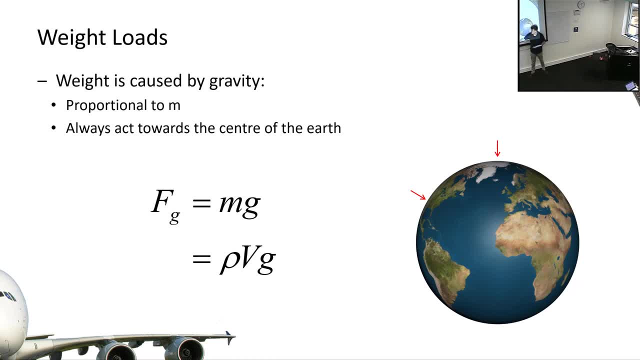 cases we consider: ah, then it's a very simple relationship to work out what the force due to gravity is, or the weight and of a point mass, or if some kind of difference between the mass and the weight of the aircraft. so if we look at a distributed mass like fuel, we just take its density, multiply it by the. 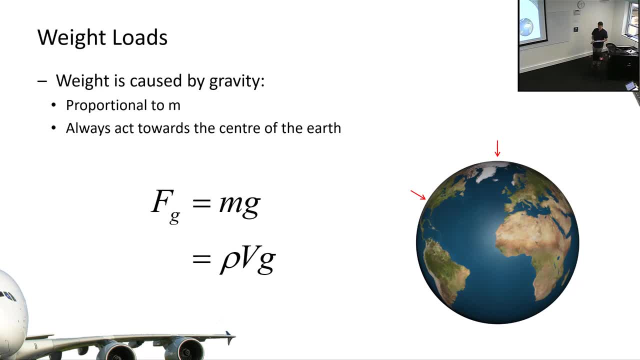 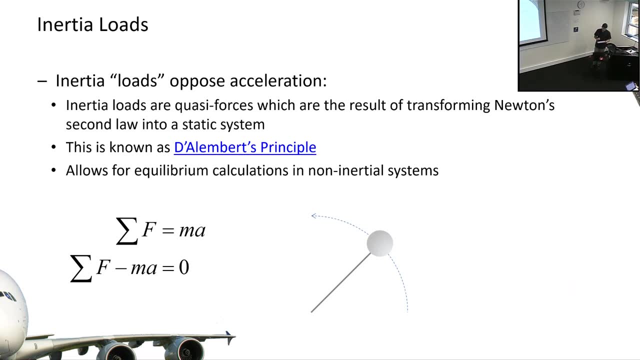 volume and then gravitational constant, and we have a force. now there's another type of load which we use a lot in this course for in accelerating systems, and it's what we call it an inertia load or an inertial load, and it's a pseudo force. it's not. 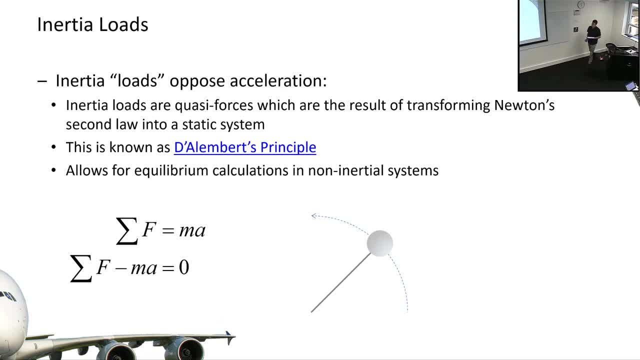 really a sort of linear time field, but it's a pseudo force. it's not really really a force and you'll get into arguments with first-year physics students about this that think they know a lot about how forces work, that we can cast our system into a non-inertial frame. 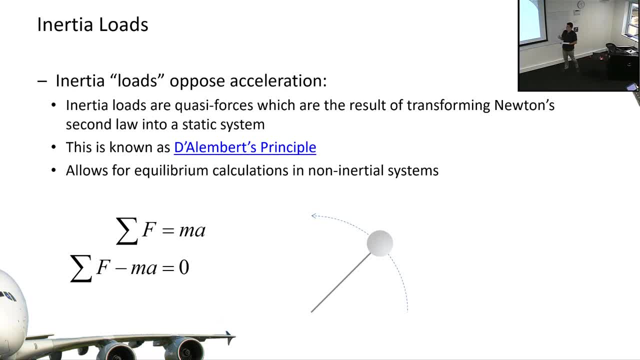 And it's using what's called D'Alembert's principle- and there's a nice link there. you can have a look- But Newton's second law. traditionally we take sum of forces on the left and we say that's equal to the mass times acceleration on the right. 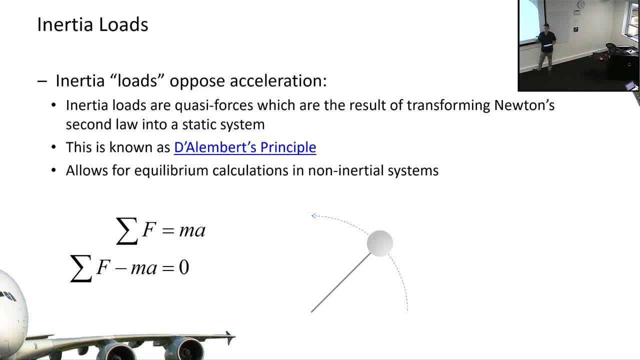 We don't really like dynamic systems very much. if we can avoid it, We like to do static equilibrium systems, And so what we can do is take the MA and stick it on the left-hand side of the equation and just cheat and pretend it's in equilibrium. 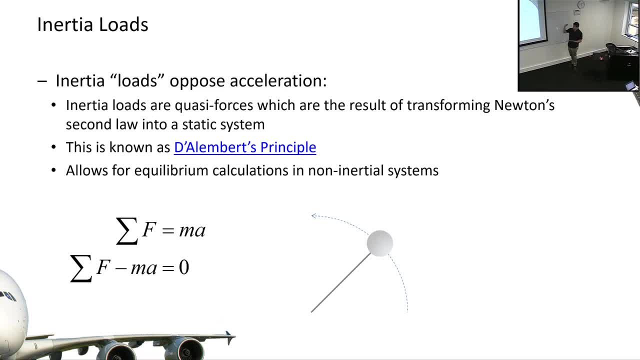 And so when we have an accelerating system like this ball on a string that's spinning around in a circle, the traditional kind of second-year mechanics way to look at that is: sum of forces equals MA. we work out what the acceleration is: V squared on R. 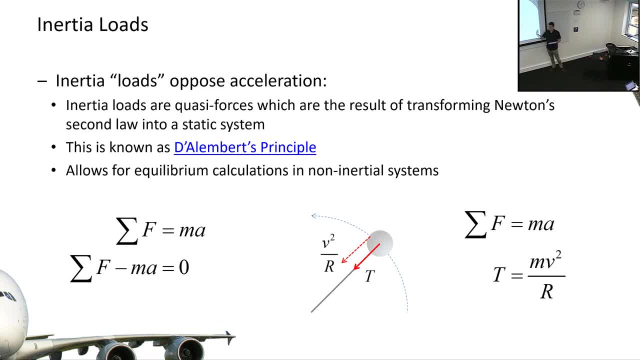 so we can work out the tension in the cable by equating: T equals V squared on R. That's the traditional way of doing things, The way that we like to do it in this course, which pays big dividends when you're talking about very complex systems. 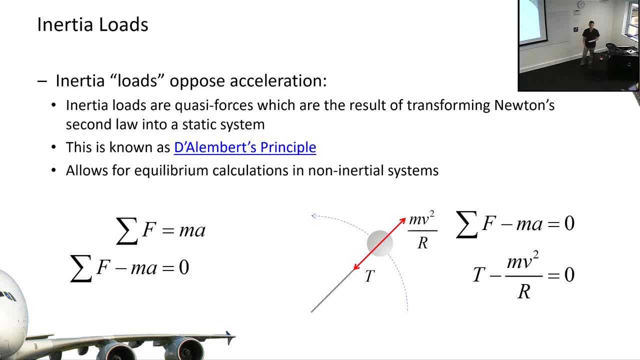 is to treat the acceleration as an inertia acting in the opposite direction. So you take any accelerations, you multiply, you multiply them by the mass. so what we've done here, and the minus sign just points them in the opposite direction and we can say we've now got this equilibrium equation to solve. 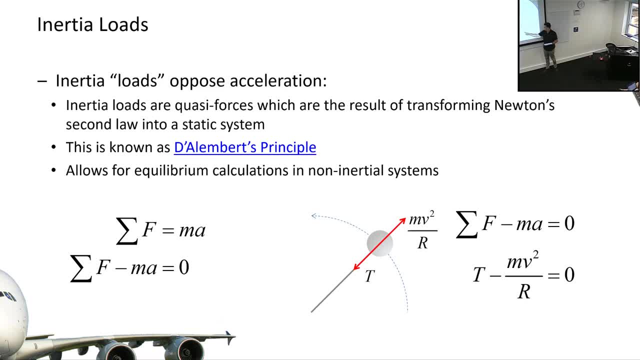 The tension on that side minus MA equals zero. T minus MV squared on R equals zero. It's the same equation. in this simple case, very easy to see the equivalence between those two things, but it's very helpful with complex systems. Now the reason. I talk about arguments with first-year physics students. 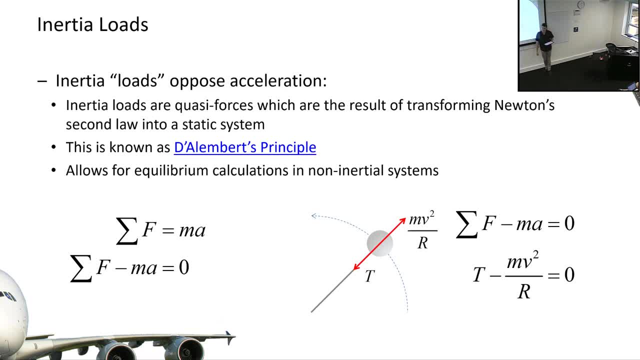 is. this is often called the centrifugal equation, centrifugal force, and if you talk to people who've just started learning some dynamics, they'll say there's no such thing as a centrifugal force. Ah, bullshit, there is a centrifugal force. 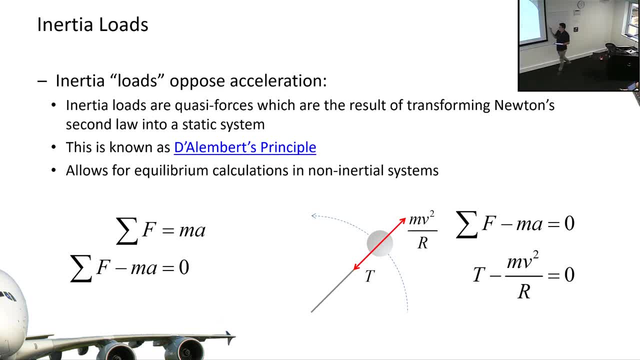 We can feel it, it's real and it's just about what reference frame we're looking in. So this way of thinking about inertia loads is very useful when we start talking about modes of motion for the aircraft where we're accelerating, And those accelerating motions are the ones 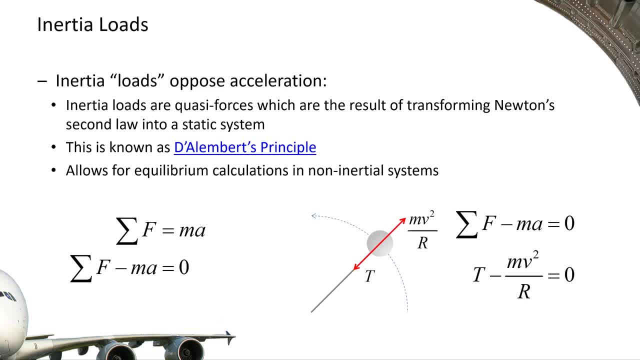 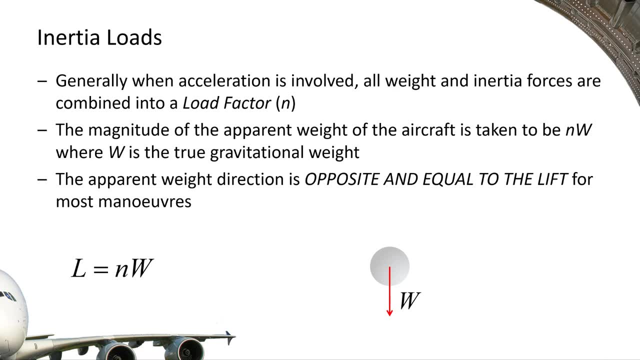 that are going to cause the aircraft to break up into pieces. And when acceleration's involved, we don't think about traditional weight. so we leave weight as it is. Weight always points towards the center of the Earth. When acceleration's involved, we think of something called an apparent weight. 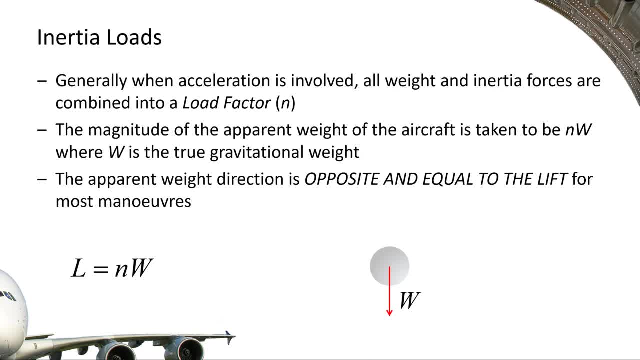 And everyone knows apparent weight, even if they don't know the terminology for it. Anyone who's been in an accelerating car or a roller coaster or a light aircraft has felt apparent weight And it's equal and opposite to. So if we've got an acceleration, 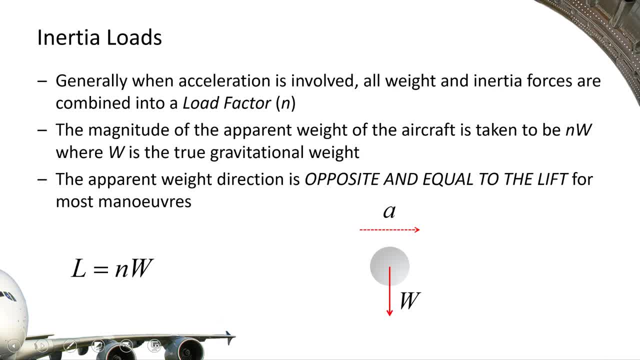 let's take this weight that's sitting there in space and we accelerate it to the right. Then we add our inertia load in, which is equivalent to our acceleration. Now the sum of these two things, in a vector way, is we call the apparent weight. 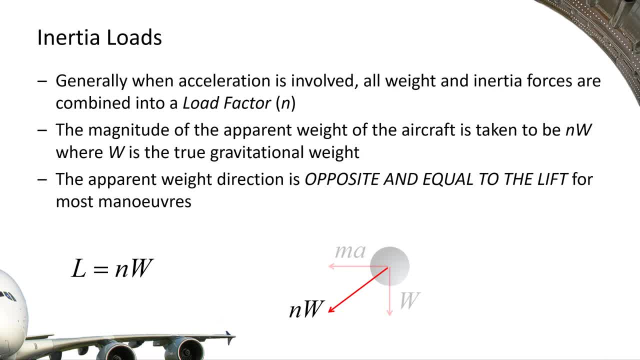 And we just give it a constant N, which is some multiple times The magnitude of it, is some multiple times the real weight, And this N is the G loading. If you've ever heard of someone talk about like the Formula One car was pulling four Gs in a turn. 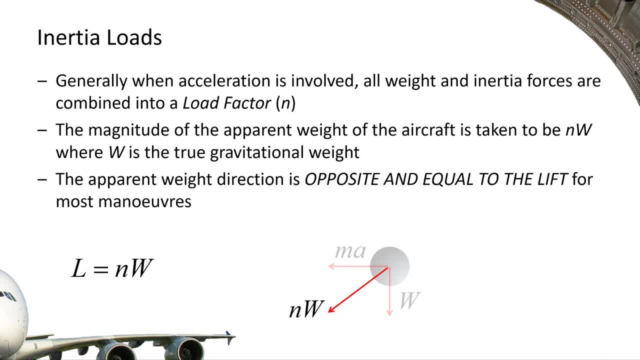 this is what they're talking about. Or if you talk about a fighter pilot pulling a certain number of Gs, that N is the load factor, we call it, And for most manoeuvres, lift is opposite this apparent weight, And we'll see that in a diagram with a turn in a second. 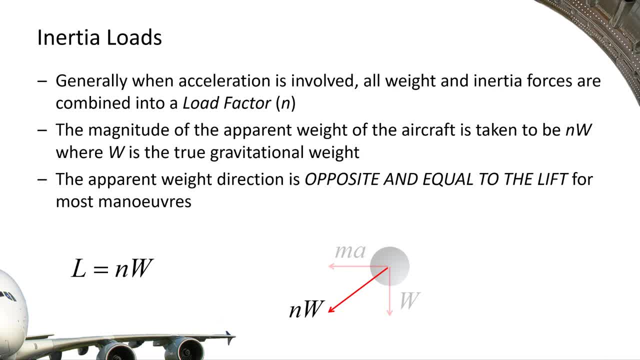 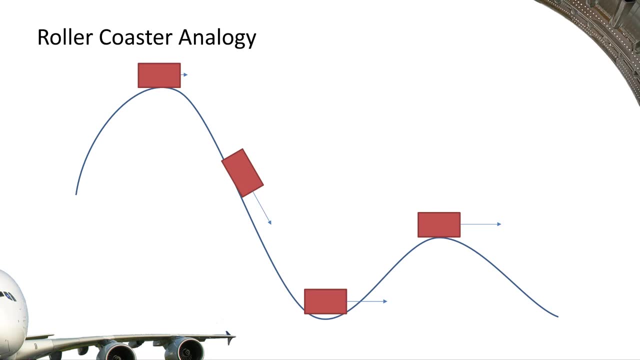 And it's equal to that, Because lift is providing the acceleration which is causing this load factor, And the easiest way. if anyone hasn't been on a roller coaster, I apologise, but I assume that most people haven't got to this point in their lives without being on a roller coaster at least once. 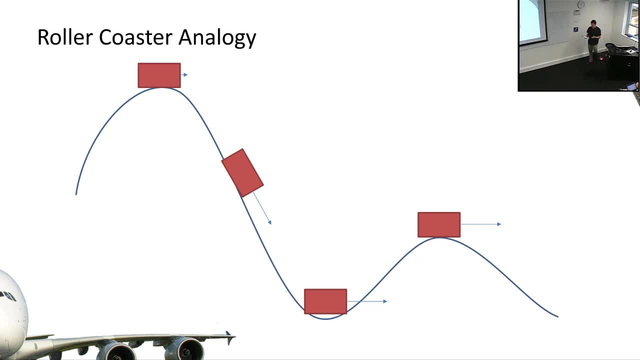 If you think about what you're feeling as you go on a roller coaster, if you go over the top of a hill, of a crest with any kind of velocity, you feel like you're leaving your seat a little bit, And if you go over fast enough, 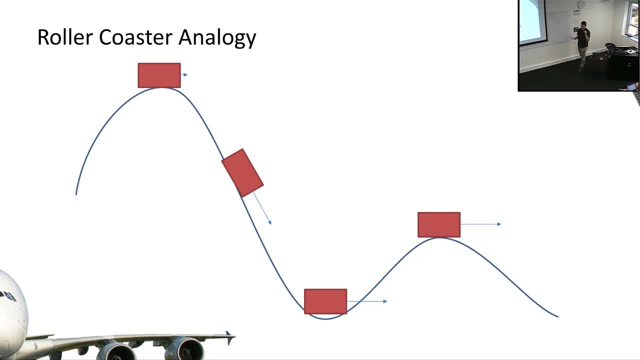 you can actually leave your seat As you're free-falling or very close to free-falling. you're not feeling much weight at all As you go through the bottom of a- Sorry, I'm taking the lapel mic- As you go through the bottom of a trough in the roller coaster. 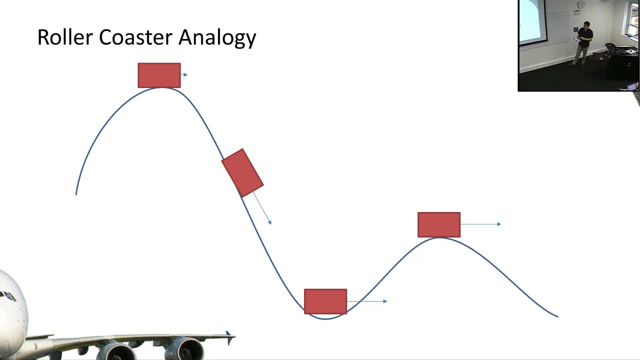 you're feeling very heavy, You're feeling more weight than usual, And And so at all times gravity is the same. We've got the same gravitational component, but what we have is different accelerations. So at the top you've got a little vertical acceleration. 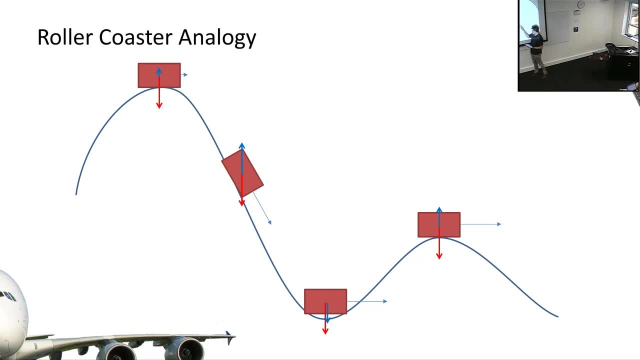 Down here you've got a fair vertical acceleration. Upwards, you've got a downwards acceleration. Oh sorry, This is the apparent component. so this is the opposite of what's really happening. So you're actually accelerating downwards here, but the inertia load is acting up. 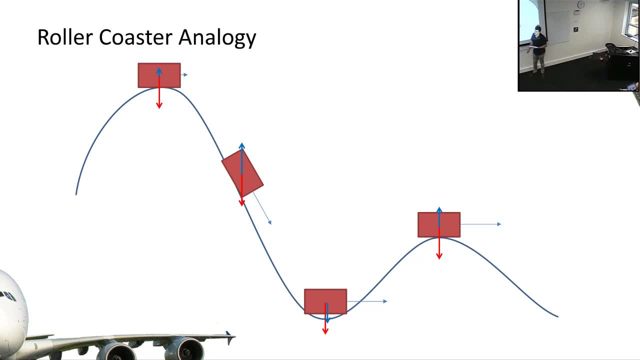 Here you're accelerating upwards, but you're Inertia, load is acting down And if you sum all those up, then you get what you're actually feeling. So in free-fall you've got an inertia load and because you're accelerating down at about the same rate as gravity, 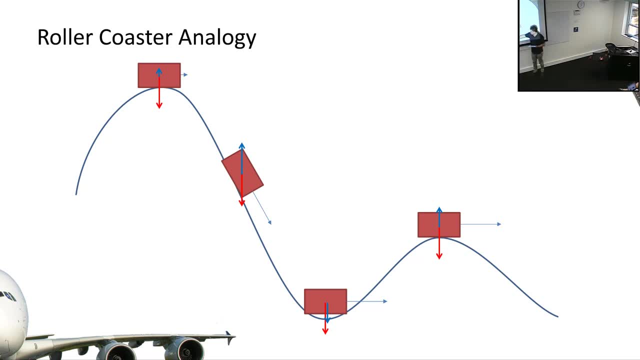 those two things balance out and you feel nothing As you're at the bottom. the two things sum up and you feel heavier. As you come over a crest at speed, you feel a lot lighter, And so that's the way that we think about. 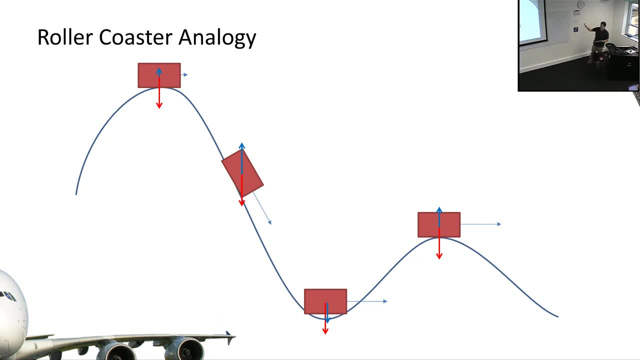 apparent weight in the aircraft, And having this kind of picture in mind when we start doing calculations with load factor is very, very helpful. Now this is the next one of those free-body diagrams that I wanted you to have a look at. Now, I'm missing some forces here, obviously. 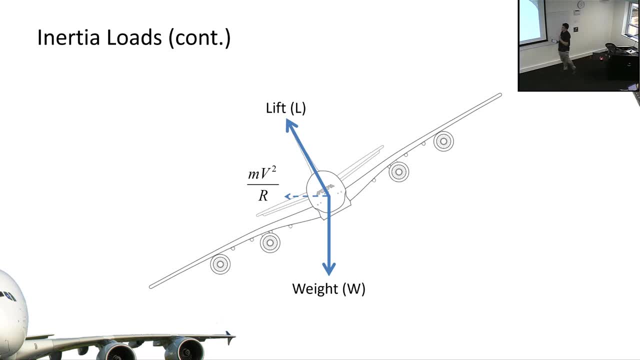 Obviously there's some drag on this aircraft and obviously there's some thrust being generated And the poor old A380 that's now being being the production line's being canned unfortunately features in a few of my diagrams. The A380 was making its first maiden flights. 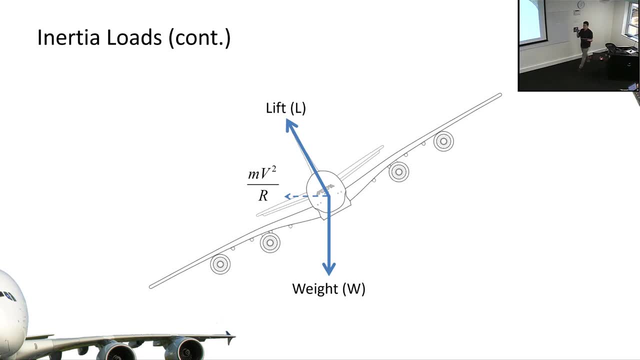 and all of its initial design and maiden flights was during my undergraduate time, And so it's got a sort of special place in my heart, as poor as it's been as a commercial aircraft. It was the aircraft that everyone I think was using, for examples, when I went through 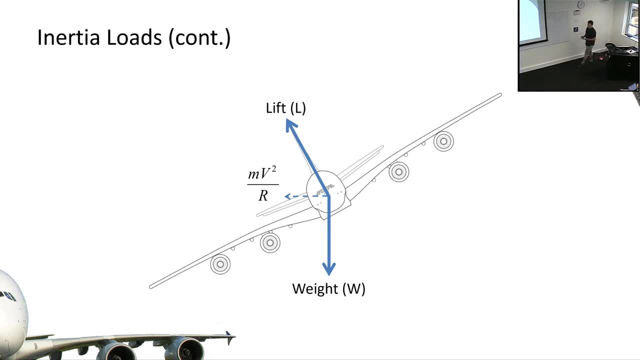 So if I need to talk about modern examples, I can pull up modern examples, but if I'm looking at loads on an aircraft then I'm going to use an A380.. The inertia loads here we haven't drawn yet, but we have our sort of traditional loads. 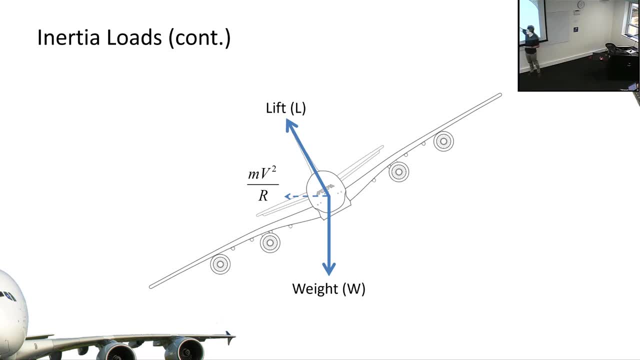 We have lift which is always drawn in aircraft coordinates. Okay, so this aircraft is banked, The weight's drawn in, The weight's drawn in global world coordinates, but the lift is drawn in aircraft coordinates, So as the aircraft moves around, 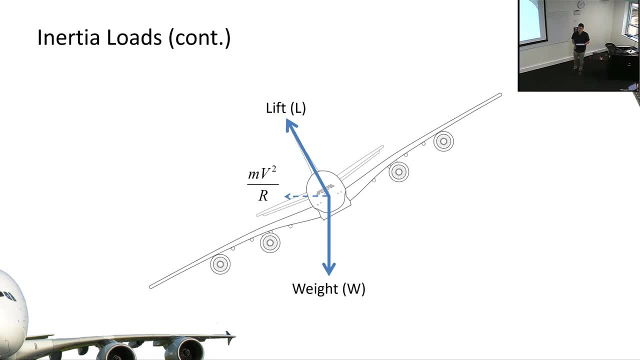 the lift is always acting in the same coordinates as the aircraft, And if this aircraft is in a level turn, it means it's not accelerating upwards or downwards, which means we have some kind of equilibrium system here we need to look into. There's an acceleration, and I've put an M here. 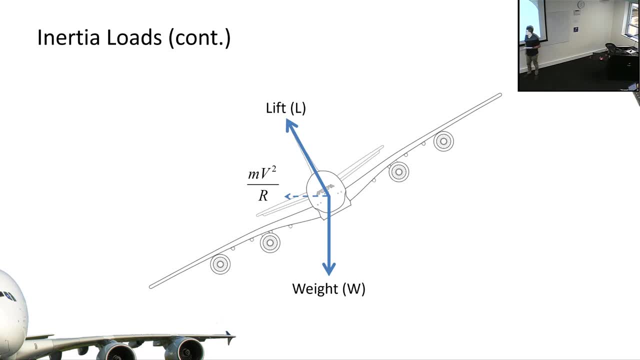 I probably should take that M out. There's an acceleration towards the centre of the bank, which I can then turn into an inertia force acting in the opposite direction, And now we have a system that we can apply our traditional equilibrium rules to. Okay. 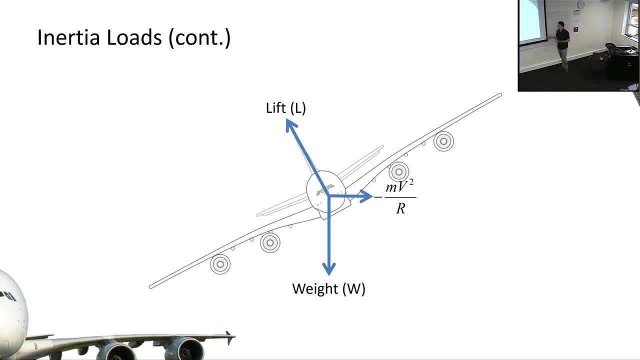 Now you can choose whatever coordinate system you like. You can choose global coordinates and say: well, the vertical component of the lift has to equal the weight and the horizontal component of the lift has to equal the inertia. or you can look in aircraft coordinates as well. 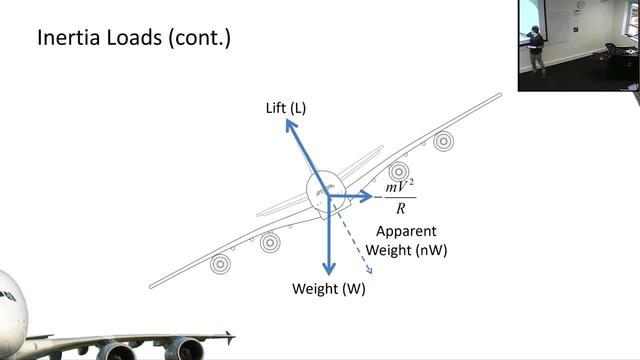 But either way, what we find is the apparent weight opposes the lift and is equal and opposite to it, So that when we do our vector sum here it's equal and opposite to the lift. Now, why are these kind of conditions important? 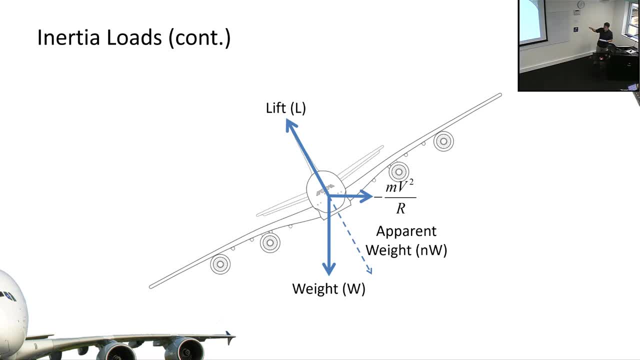 Well a turn. when this apparent weight, this load factor here N, is bigger than 1, then our aircraft, all of the aircraft structure that's generating that lift, is experiencing loads that are scaled by this load factor. So if you're generating more lift, 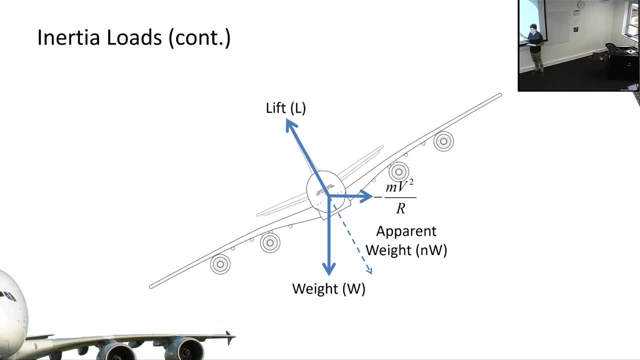 so remember here: lift is equal to N times weight. If you're generating more lift, you're generating larger stresses, you're generating more loads on your airframe that you need to account for. So this N is really like a scaling factor for how much stress we're putting our aircraft under. 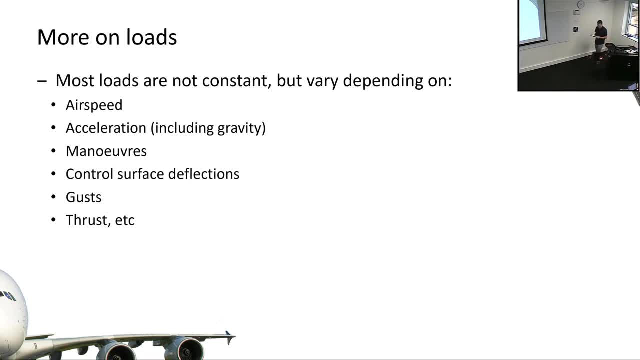 Now, everything I've said up to this point is very simplified. obviously, Most loads aren't constant. They're varying depending on airspeed, acceleration maneuvers, control, surface deflections, all sorts of things. So we won't talk about most of these variations in this course. 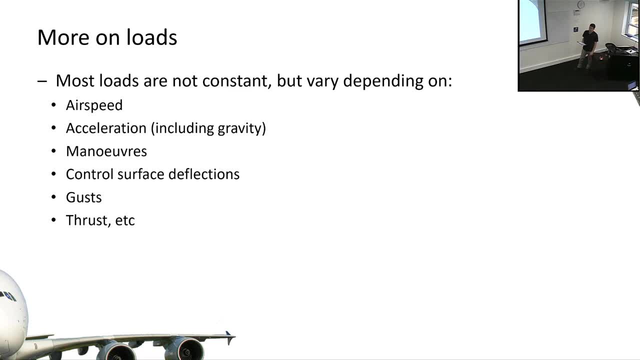 A lot of them are for other performance-related courses that you'll come across. But just be aware that when you're starting to do any kind of design calculation or you're trying to reverse engineer a structure, you're not reverse engineering it for the straight and level flight case. 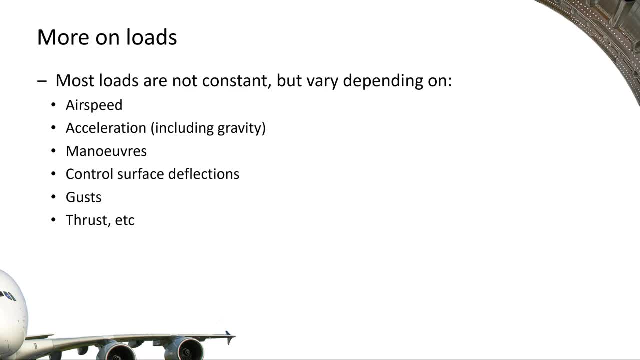 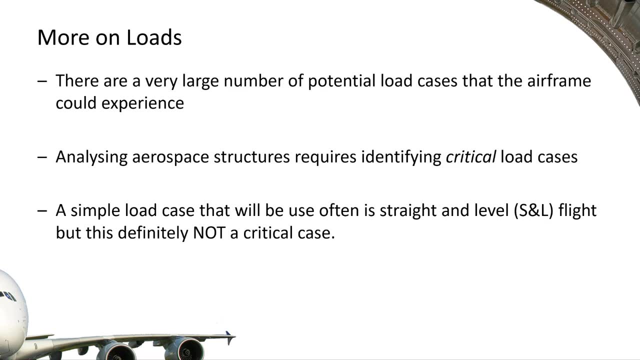 You're trying to find critical cases with which to do your calculations And those critical cases. there's a near infinite number of conditions that we could get the aircraft in while it's flying And there are a lot of rules in the regulations about identifying what we call critical load cases. 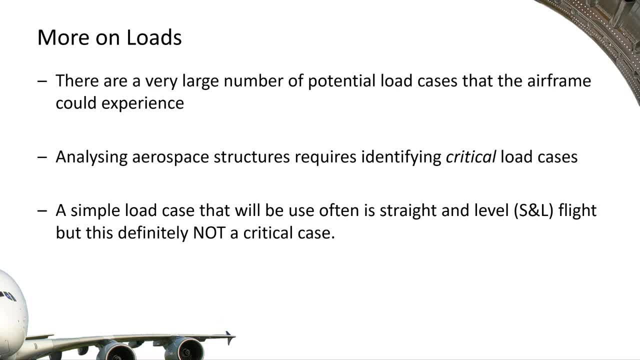 So those critical load cases are ones that are likely to induce failure, or those kinds of conditions that the aircraft may experience that are likely to induce failure, And the simplest way we can handle these critical load cases is with what we call a flight envelope. 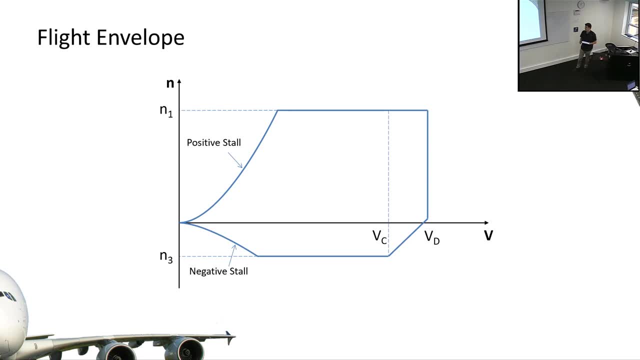 Now I won't go into too much detail in this course about a flight envelope, other than knowing that it's there. that's Sonya's job in design next semester, But just to give you a very brief overview of how it works. 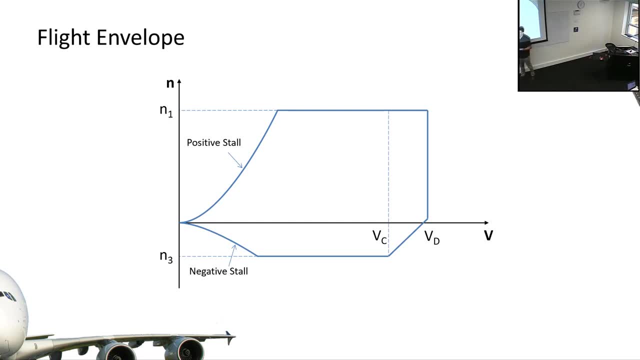 the vertical axis. here n is our load factor that we've talked about. So this is when you're feeling really heavy and this is where you're feeling really light, Or actually when you're zero, you're feeling nothing. If you're feeling negative, n. 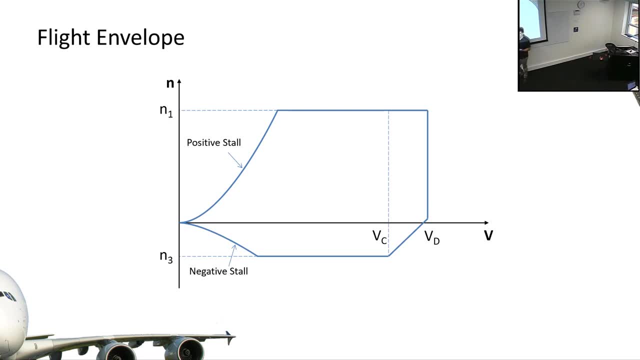 it means you're actually feeling like you want to go the opposite direction, like when you're going across the top of a crest, And v- I should probably have v? e here- as your equivalent airspeed. Now, equivalent airspeed's not your actual airspeed. 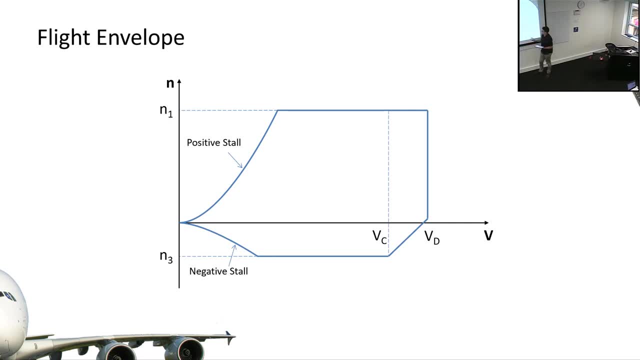 it's scaled by air density and other things that you'll learn about, But really this is saying: this is how fast the aircraft's going and this is how heavy you feel or how much load is on the structure. What we say is that the aircraft 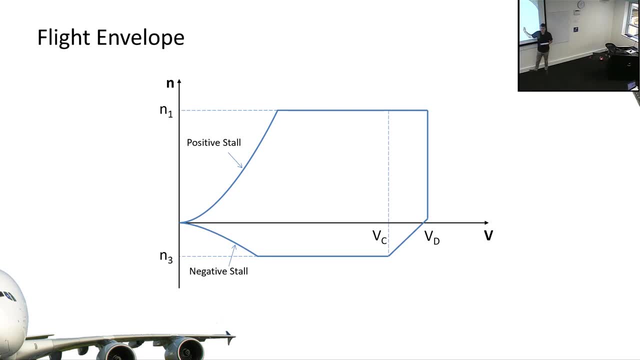 has to live inside this envelope. Otherwise, this is what we call a design envelope, because these are the conditions that we design the aircraft for, And as long as the aircraft lives its life inside here, we're okay. If the aircraft goes outside of these boxes, 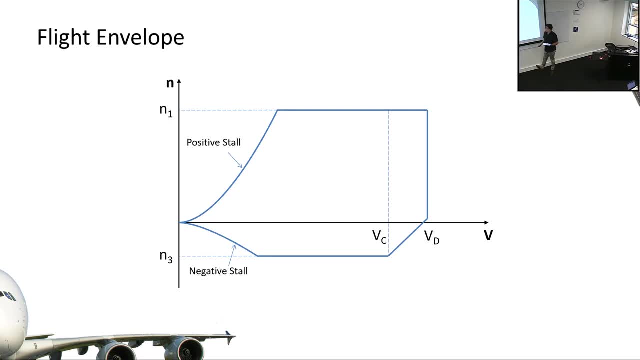 we've got a problem Now. the notation on here is the notation taken from the FAR regulations. Now you're in an interesting time because the FAR have just changed. about a year ago they massively changed how they regulate. They've changed the way that regulations work. 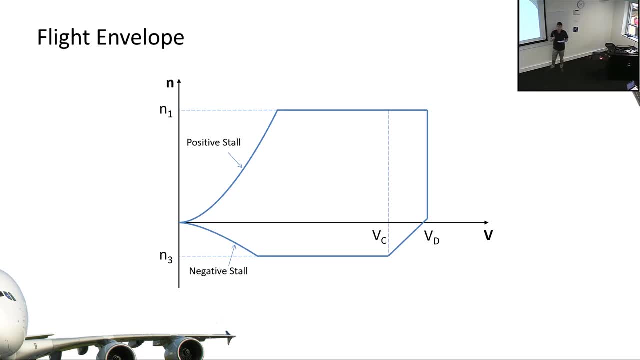 They used to have all of these diagrams and calculations and they said: this is exactly how you design an aircraft. Now all of the detail has been taken out and thrown into ASTM standards that say this is a good way to design an aircraft. 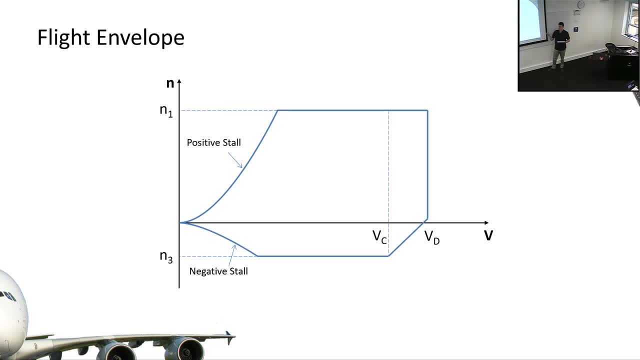 but the regulations now just say very simple statements like: it must be able to withstand the aerodynamic loads and it must be able to withstand these things. So the regulations now are very simplified, but it means you've got to go and do it. 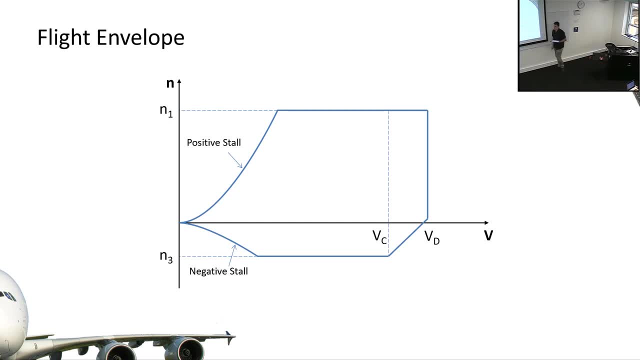 and you've got to dig for the detail of how you would do it if you wanted to do a generic aircraft design. Let's go along this axis. There are a few labels on this axis which I won't talk about because they're not relevant to this course. 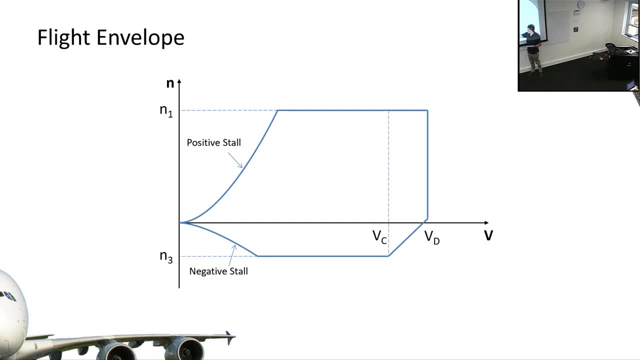 There's a VA and a VB and a VA star and other things along here. VC is our critical or our cruise velocity. Our cruise velocity is where the aircraft is spending its time in straight and level flight generally, and straight and level flight is. 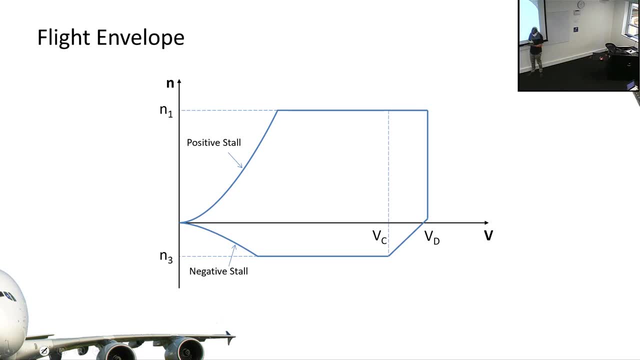 if I can bring up my pen straight and level flight lives there where we have a load factor of one, Because if you've got a load factor of one it means your lift equals your weight. you're feeling traditional 1G loads on you. 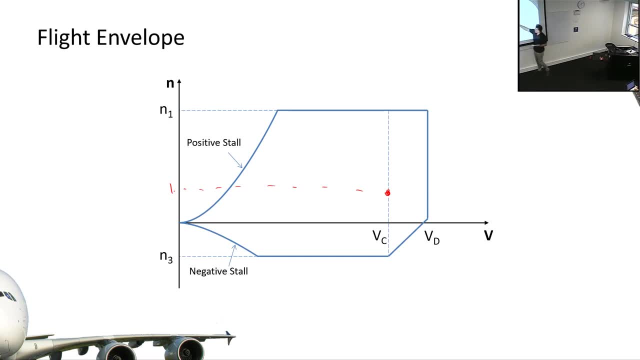 So that point is a fair way from most of the edges of the box. It's not so far away from this side, but unfortunately, in order to make our aircraft get from point A to point B in an efficient amount of time, we have to fly fairly fast. 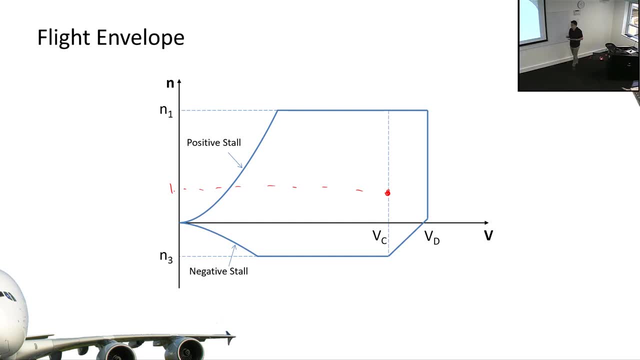 relative to the critical speed of the aircraft. Now VD is often called the design dive speed. Luckily, a lot of the critical terms also have D in them. It's also the divergent speed. It's the speed at which you're likely to break the aircraft. 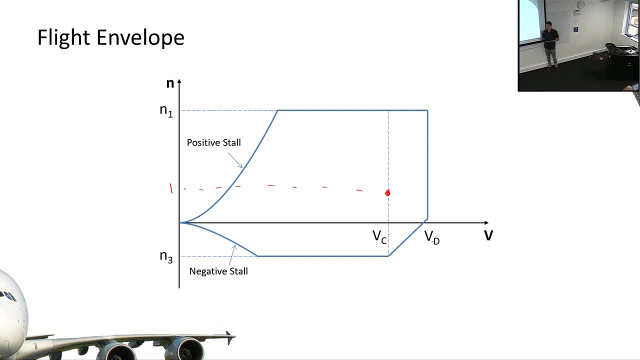 from flying it too fast. So there's a certain speed we'll find out about right at the end of the course where, if you exceed that speed, your wings will twist off and you won't have an aircraft anymore. You'll have a lying cigar temporarily. 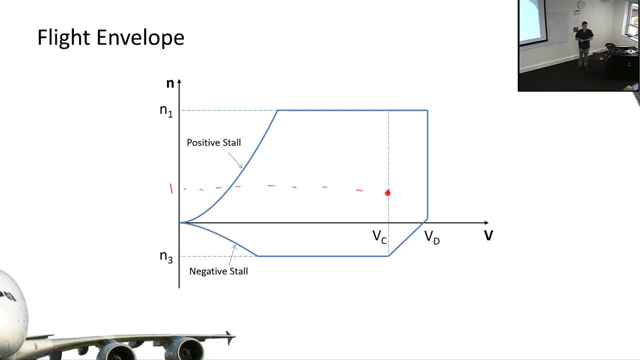 and then a falling cigar. I think you mean a flying coffin. Yeah, a coffin, yes. So this speed is something that a pilot can break our aircraft by exceeding. Engineers are never at fault here. if we do our job, It's always the pilots that are going to break things. 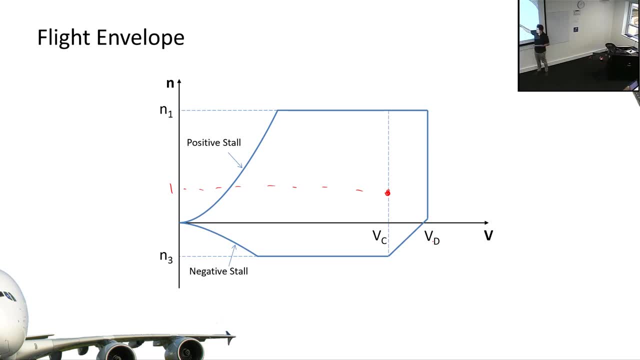 A pilot can fly the aircraft too fast and break it. And also if we go vertically here, if we go too high, which means we've pulled a manoeuvre, that's too many Gs. so if we've done something that's made the aircraft too heavy. 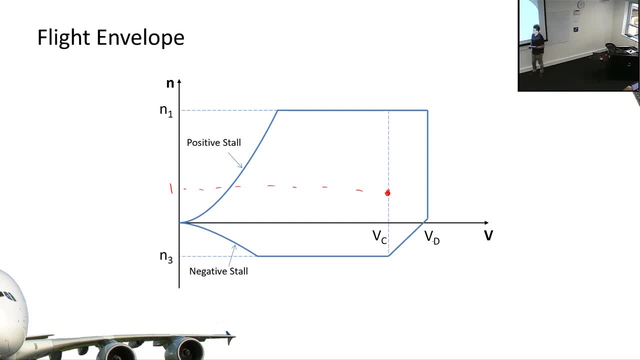 or made us too heavy. that is generally things like banking in a turn that's too tight or pulling out of a dive too quickly. You can generate positive manoeuvres that have got too high a load factor, And this number's generally about three. 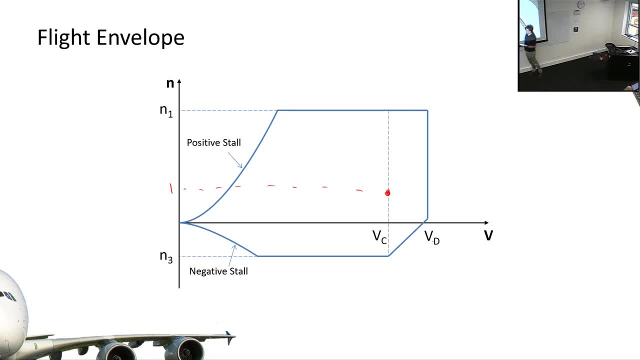 It's three plus or minus something. For acrobatic aircraft it can go up to eight or nine, And for very high performance military aircraft it can be much higher than that. But this is where, if you go above that, you'll snap the wings off your aircraft. 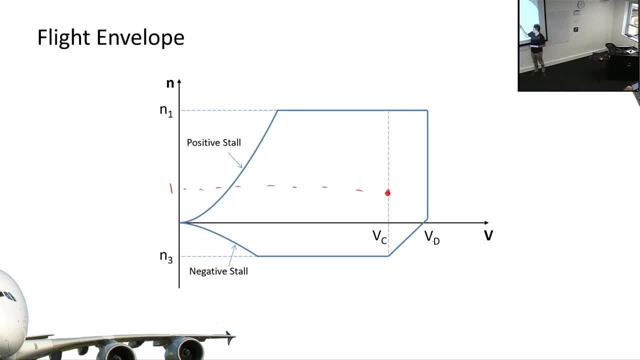 through just making it too heavy. This is where you'll snap the wings off your aircraft by flying too fast, And this is where you'll snap the wings off the aircraft by doing the opposite of making it too heavy. So if you just push down on the stick, 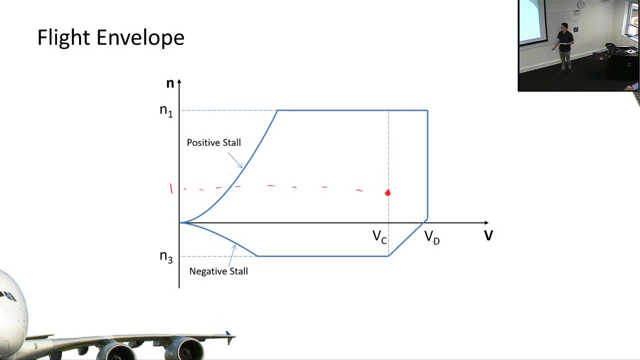 and sort of go over a crest too fast, then you're doing the opposite thing to what you normally do and you'll break it in the other direction. The only interesting part of this: that's not to do with pilots breaking the aircraft. this is just to do with physics. 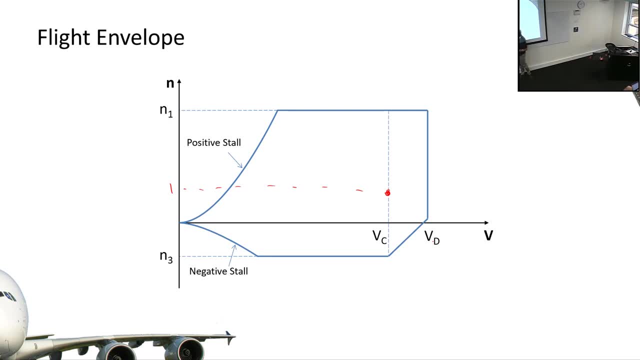 Again, the engineer's not at fault. We have here this is what we call stall lines. So if you fly faster, sorry if you fly slower than this point, this point here, if you fly slower than there, this velocity. 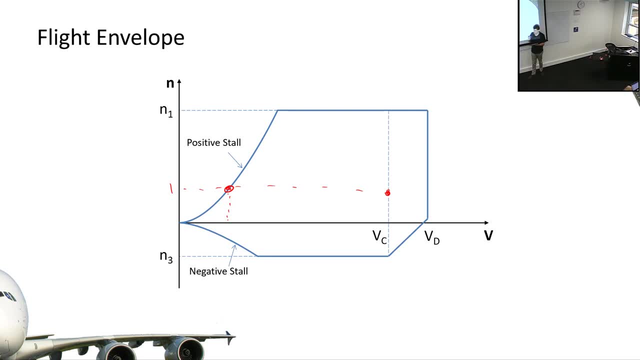 at straight and level sort of G equals one. conditions you will. the wings will stall, They just won't have enough speed over them to generate lift and they'll stall and your aircraft will start falling out of the sky, And the same in the negative condition as well. 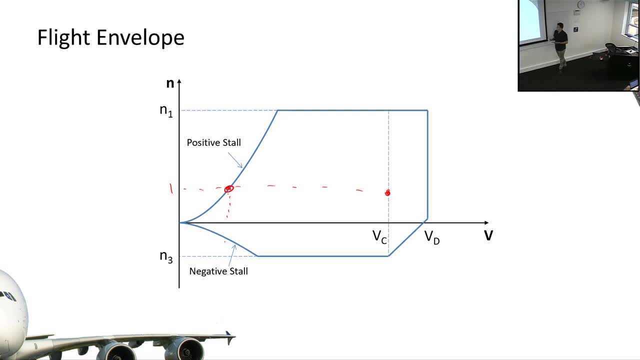 You're going to have negative stall from going the other way, Because to fly slower you've got to increase the angle of attack, you've got to generate more lift and eventually there's just no more lift to be able to, there's no more ability for the wing to be able to do that. 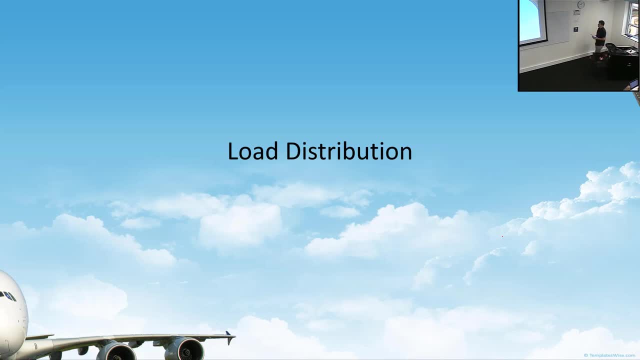 Alright, that's enough talking about what we call a V-N diagram or a flight envelope. Let's talk about distribution now. So everything we've talked to at this point is primarily treating the aircraft like a particle, like a point Now we want to think about. 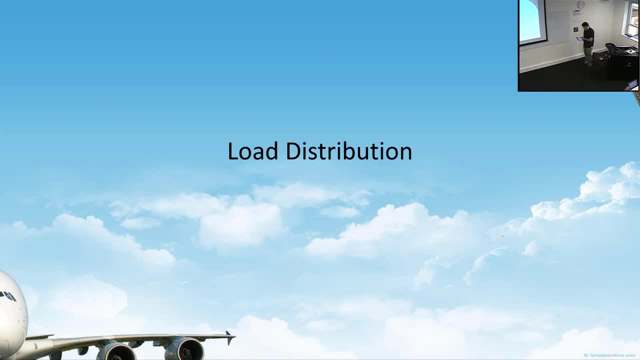 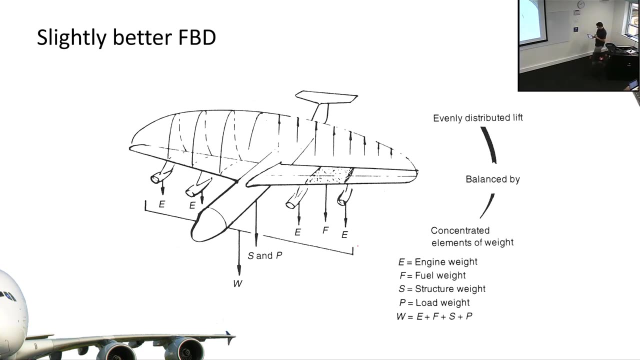 how the loads are actually distributed. Now this: I haven't actually noted where I've stolen this diagram from, but this is not my diagram. This is a good sort of first approximation for a better free-body diagram that gives us some indication of what the stresses in the aircraft are going to be. 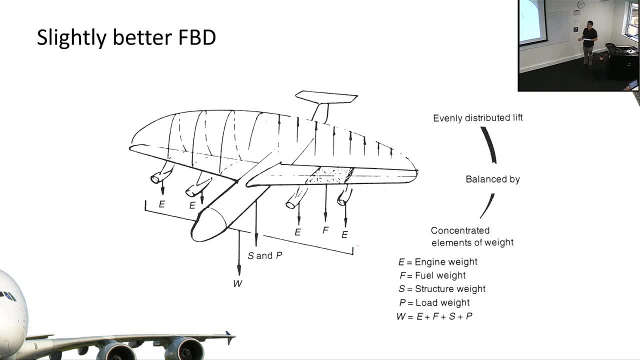 or what the loads are going to be or the moments, And this is taking loads and actually distributing them to where they're being generated. So we have some kind of lift distribution and most of the lift is being generated by the wings. There are bits of lift generated elsewhere. 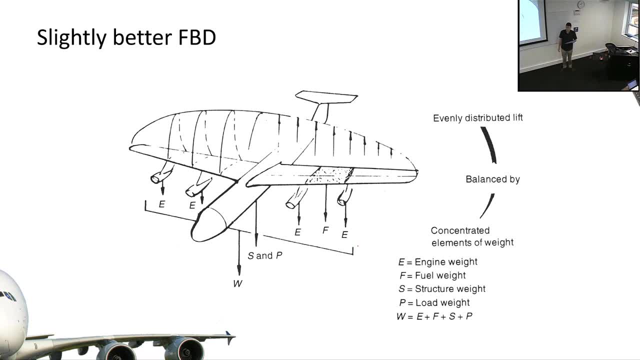 but they're secondary, So that's a distributed load and to a reasonable approximation the lift is generated in a shape like this. There's not much lift being generated out near the wingtips due to the complex aerodynamics that's happening out here. 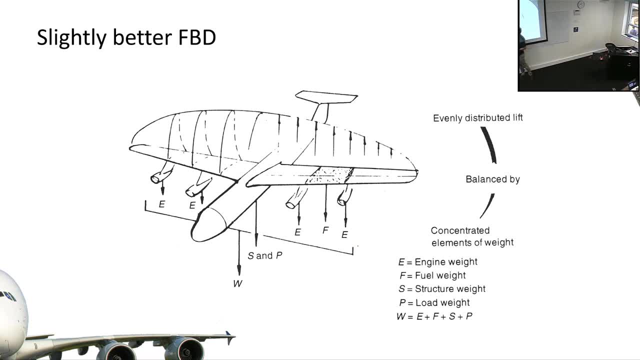 There's a lot being generated in here, Maybe a bit of a dip around where the fuselage is, and then there's not much generated at the wingtip again, And that's balancing point loads. So we have structures and payload engines, fuel and point loads. 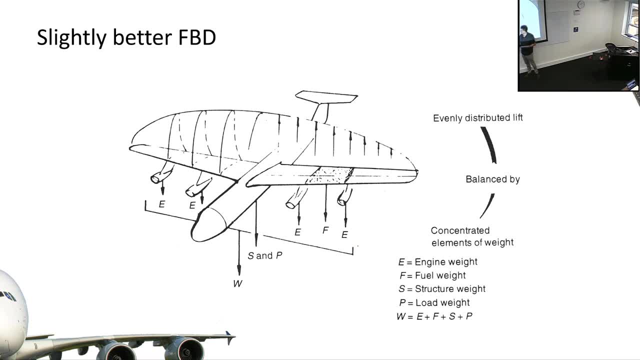 or distributed loads, but they're weights. So all of these bits at the bottom we would call our weight and the bit at the top we would call our lift. Now, that's now starting to look like something that you should be able to analyze. 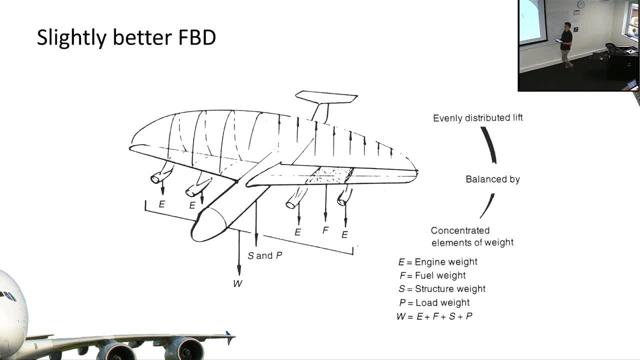 If you're thinking, if you just squint a little bit and look at it out of the side of your eye, then this looks like a beam. We have a distributed load on a beam and we have some point loads coming off that beam. 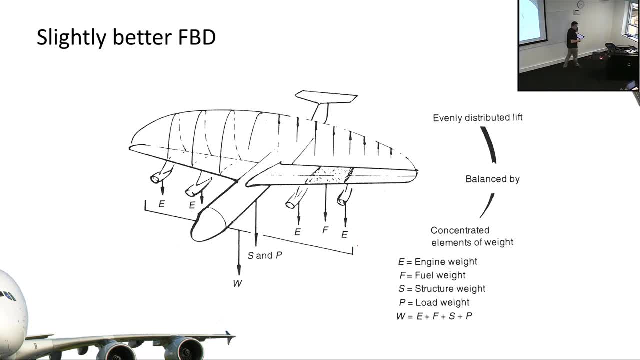 We're starting to get something that we can analyze for loads and shear forces, bending moments and things like that, And this is, in fact, the vast majority of how we're going to approach things in this course is to treat the aircraft like a bunch of beans. 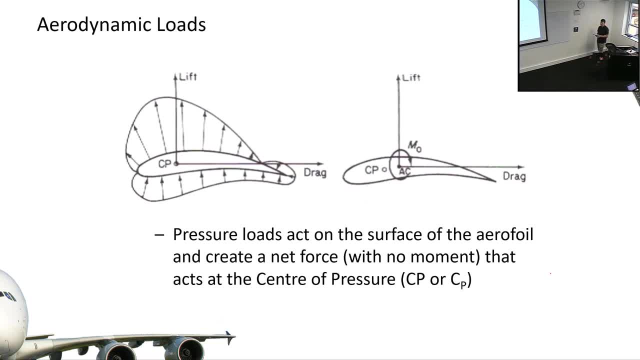 There's a few aerodynamic things that I have to introduce now, as much as it pains me. I can't stand aerodynamics and I've never been good at it. I think those two things might be correlated, But we need to talk a little bit about aerodynamics. 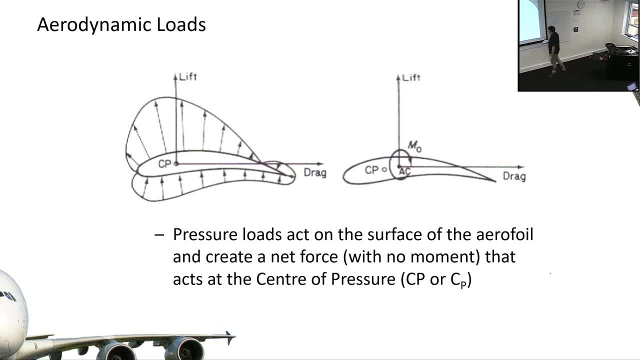 in order to understand how we're applying forces For a particular airfoil, and you'll learn a lot more about this, and so if I tell you something wrong here, just ignore me, because I'm probably wrong For a particular airfoil in a condition. 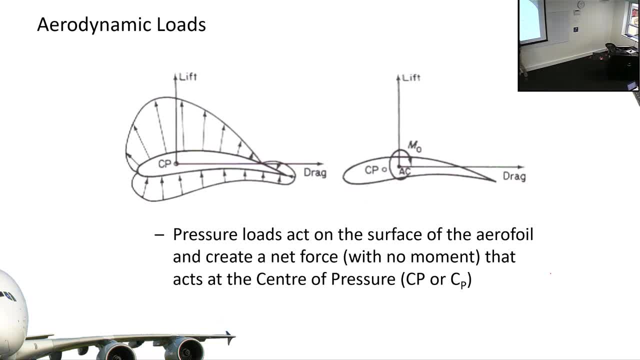 in a particular flight condition. there's a point at which all of this distributed lift and drag- I'm slicing through the airfoil here- acts, So we can take all of these forces and take a particular point and say we call this our center of pressure. 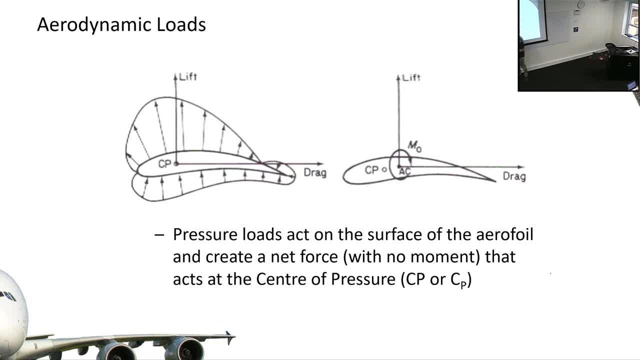 And we say: lift is the component of force that's acting vertically in the aircraft, components in coordinates, and drag is the bit that's horizontal. Now the magnitudes here are all out of whack, because if we've got a drag that's this big. 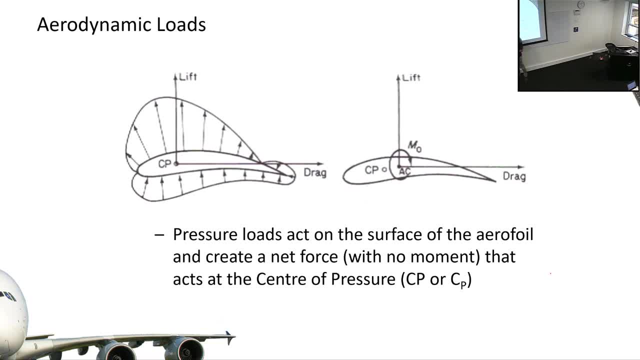 compared to our lift, we're not going anywhere today, Generally, the drag's a lot smaller than the lift. Now that's useful, but not so useful for structures- people- because as you change the angle of attack, this point moves around. 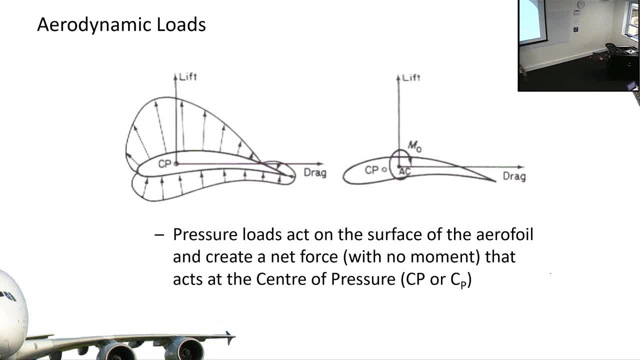 As you change the angle of attack your lift distribution is changing a bit and that point is moving. So that point becomes not so useful for us, because it's very easy for a slight change in conditions of the aircraft to move our reference point. 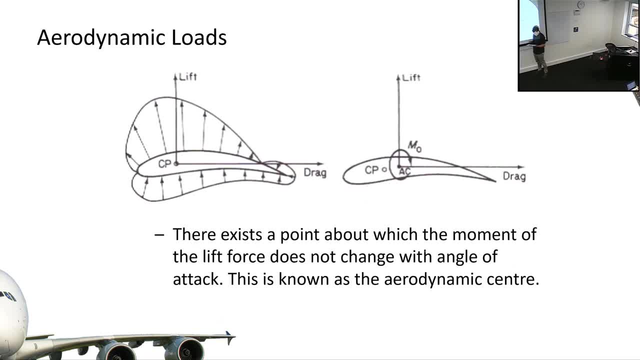 So what we tend to use is a thing called the aerodynamic center, which is drawn over here, And the aerodynamic center's not at the center of pressure. The aerodynamic center is a point about which the moments so remember, because we've moved our reference point. 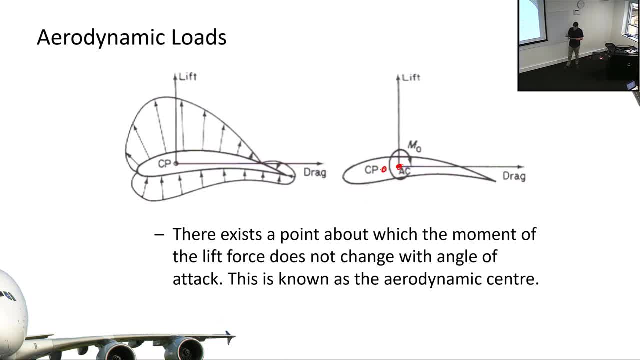 we also need a moment now. It's the point about which our moments don't change with angle of attack. There exists a point- We could pick any point. We could pick a point here, we could pick a point there. There exists a point at which 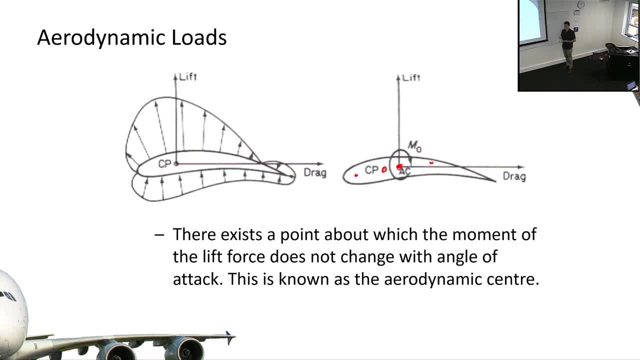 if we resolve our forces and moments at that point, those moments don't change with angle of attack, so that we can simplify the moment calculation and take it out of the expression and then just worry about how our lift and drag varies. So we tend to do most of our calculations. 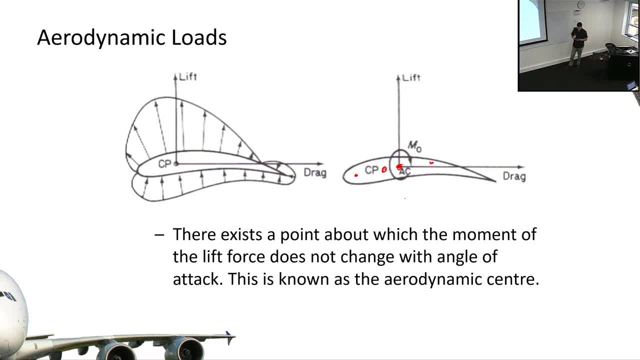 at a point which we call the aerodynamic center, And the aerodynamic center to a reasonable first approximation for most airfoils is about a quarter of the way from the front to the back of the airfoil which we call the cord. 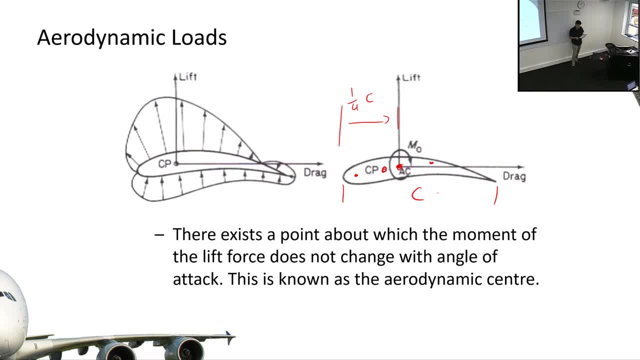 It's a quarter of the cord from the leading edge to the aerodynamic center. for the vast majority of airfoils that we use, except delta wings and all sorts of strange aerodynamic surfaces For traditional airfoils, that's a pretty good approximation. 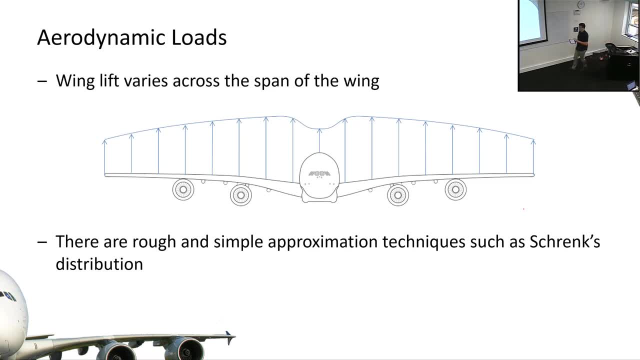 Now, when we start treating our aircraft like beams and trying to do calculations based on those beams, we need to have an understanding of how lift is distributed, And I don't know why my line drawing of my A380 doesn't have wing fences. 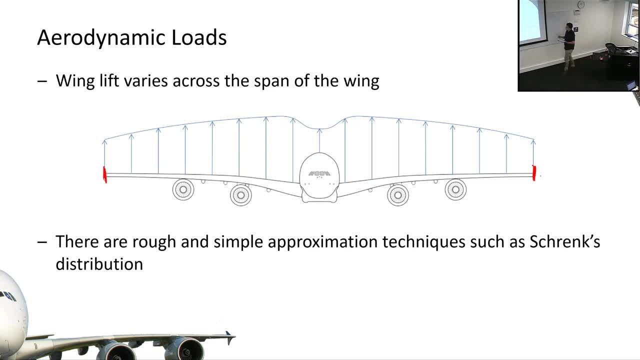 That's a bit of an annoyance, But the lift distribution, for want of a better approximation, looks a bit like this: We can approximate that with a number of different methods. There are semi-analytical methods called lifting line theory, and there are other aerodynamic tricks. 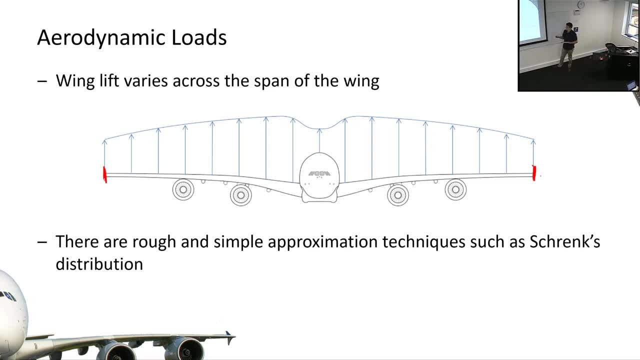 to work out what it's doing. There's a really rough one called strength distribution, which you can look up. I think I have some notes for it in the notebook, But it's an approximation, where you sum up an ellipse. So if you draw an ellipse on here, 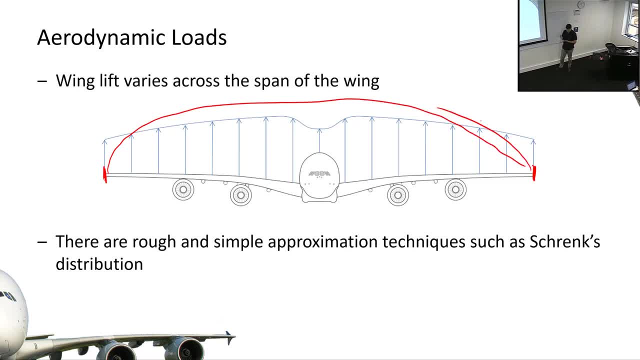 you sum up an ellipse- Now, I'm not good at drawing ellipses, I've just shown myself- And then you sum up another shape, that's the shape of the airfoil plan form, which in this case probably looks something like this: 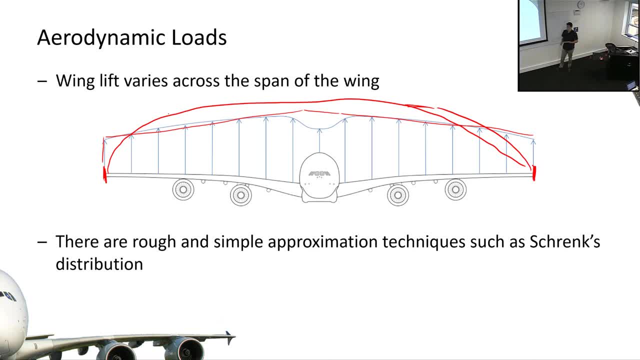 If you sum those two things up, you end up with something that pretty closely approximates the lift distribution. Now I'll leave that for you to have a look at on your own time. It's not so critical for the calculations that we do. 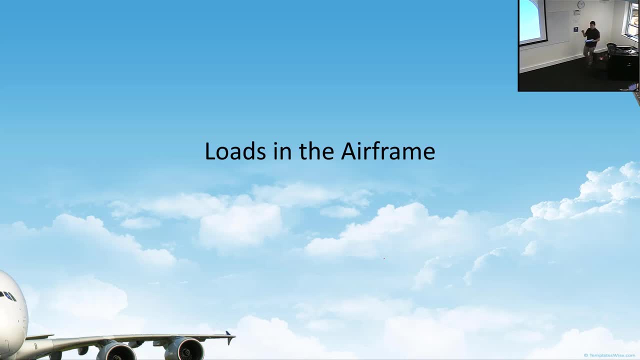 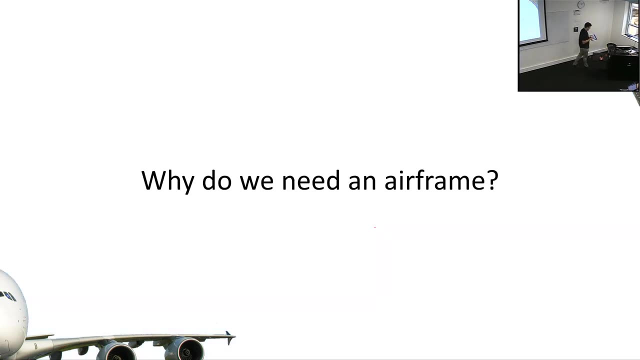 OK, so loads in the airframe. So we've talked a lot about loads on the airframe. Now we're going to talk about loads in the airframe. But I want to ask a fairly strange question: Why do we need an airframe? 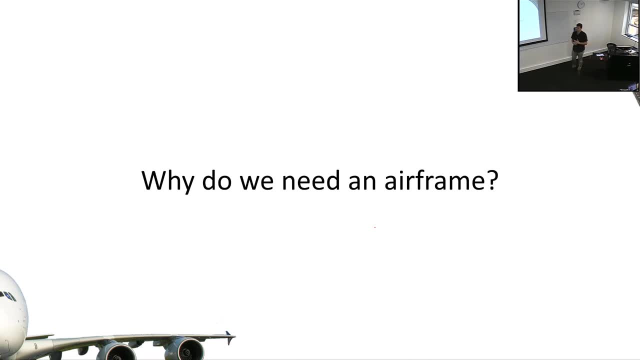 What is an airframe actually doing for us? Yeah, so we need a structure. So, obviously, if we're flying along at a few hundred kilometres an hour with airflow hitting us in the face, it wouldn't be particularly pleasant. So the first job, obviously, is environmental protection. 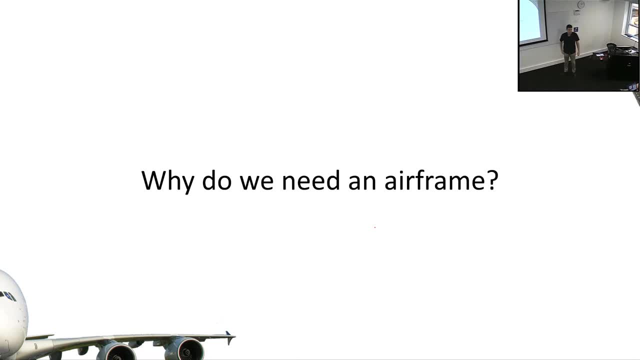 It's giving us something to be inside. But if we had to think abstractly about what the structure of the airframe is doing, what's its primary structural role? Why do we have all the bits of the aircraft the way we currently have bits of the aircraft? 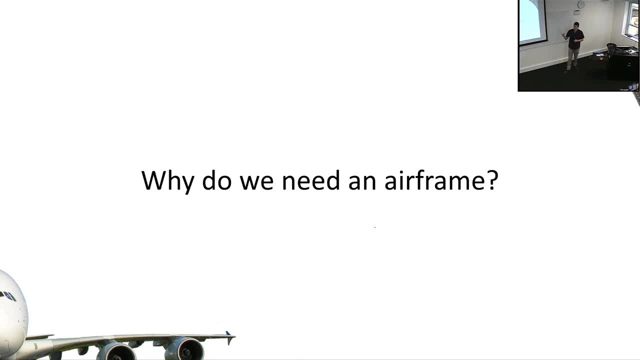 Yeah, so it's withstanding load, but where is the load coming from? We're generating lift in one part of the airframe and we have weight in another part of the airframe. Yeah, so we've got air pressure on the fuselage and on the wings. 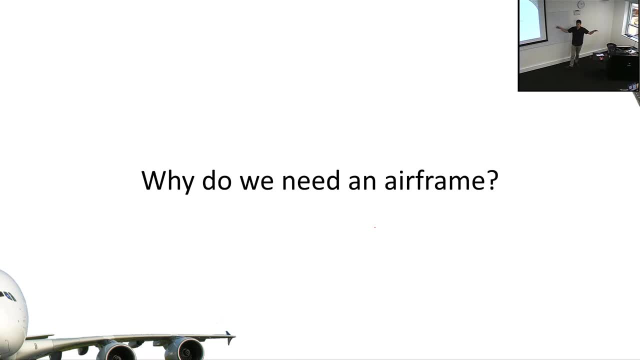 which is generating our lifts And the airframe moves those loads to where the weight is. That's really what the airframe is doing. So we can't generate lift where the weight is unless we've got some crazy flying wing configuration. With our current airframe configurations, 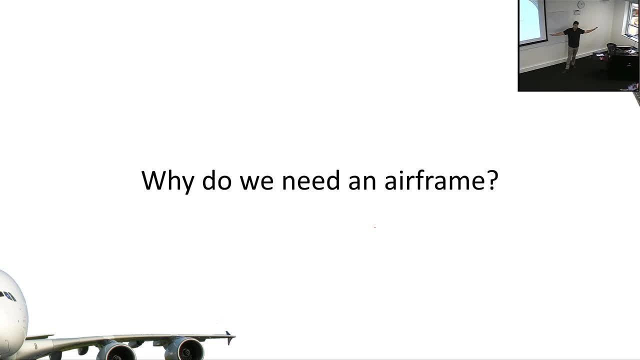 the lift is generated in a place I'm going to flap my arms a lot in this course. It's generated in a place that's not where the core mass of the airframe is, So the payload and all the things that we want to get up there. 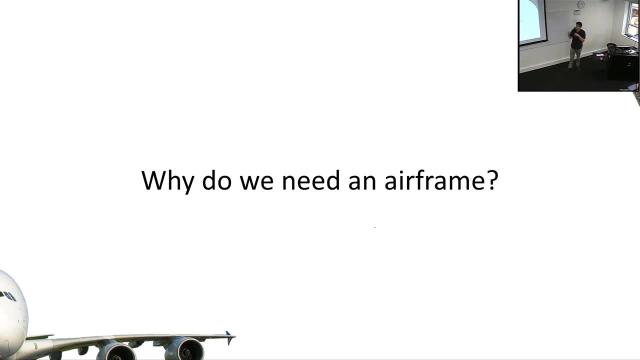 are in the fuselage, and all the bits that are doing the job for us are out in the wings, and the airframe is translating the loads generated in the wings to the payload, And so its primary structural role is to literally move that load from one place to another. 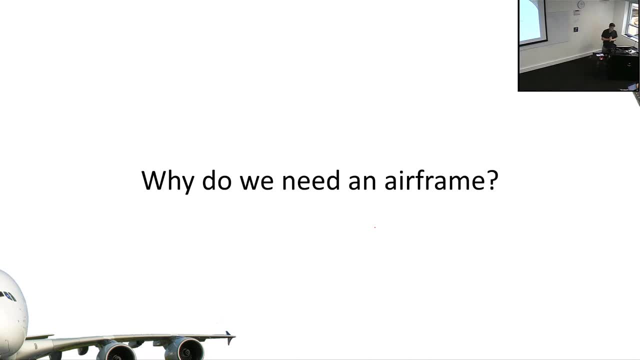 And so we work out all of the loads that are required, the amount of material that's required and the type of material that's required, and its layout in order to do that job. And that's the primary job of the airframe. 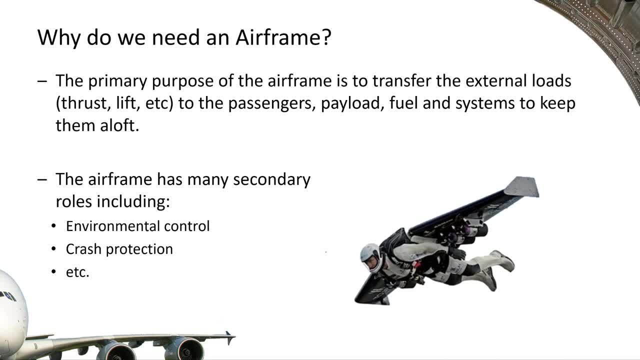 So to move all the external loads, thrust, lift to the passengers and payload. We don't want a jet engine strapped to our to us when we're flying along, unless we're this crazy guy And if you haven't seen those Red Bull videos. 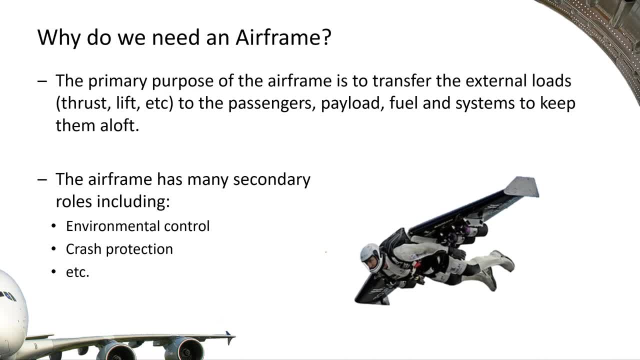 it's well worth a watch, But the you've got all of these loads being generated on the aircraft, where the thing when we sit in a seat, where the thing that we're paying the money, where the payload we need to be moved from one place to another safely. 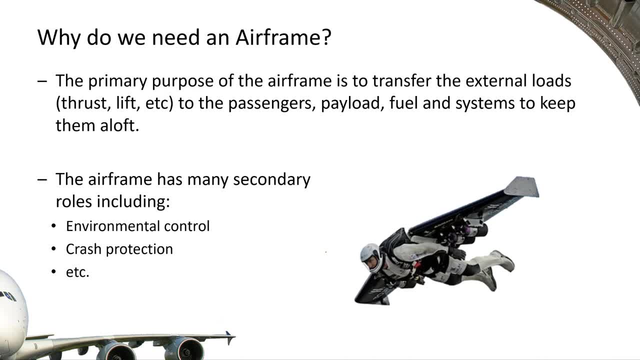 So the airframe is transporting the loads from where they're being generated to where they're being used, which is to keep all of the things inside a loft. Now there are a lot of secondary roles. It's very simplistic to say it only carries load. 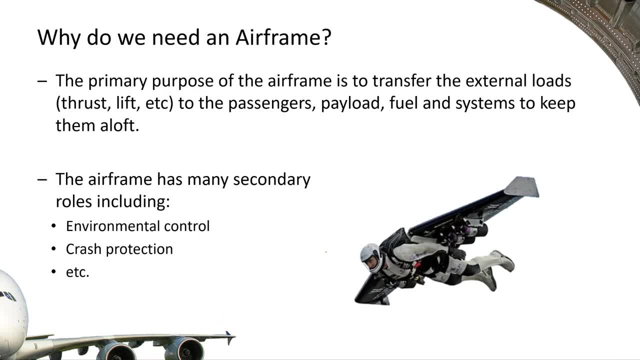 Obviously environmental control, keeping pressures, temperatures, everything reasonable for human existence, Crash protection. so there's a lot of structure underneath the floor in an aircraft that's designed to dissipate energy if it crashes. And there are other roles as well, But the biggest one that concerns us in this course 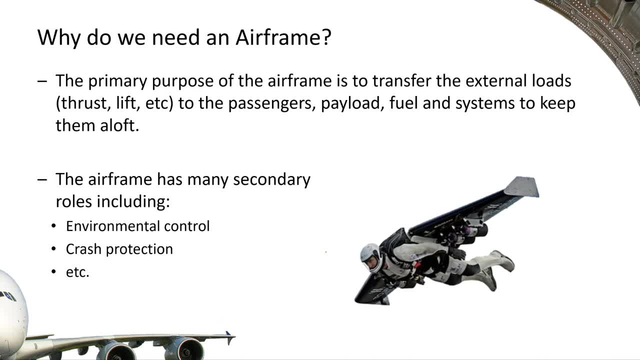 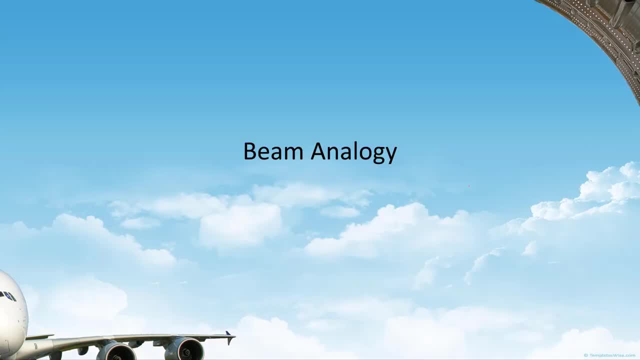 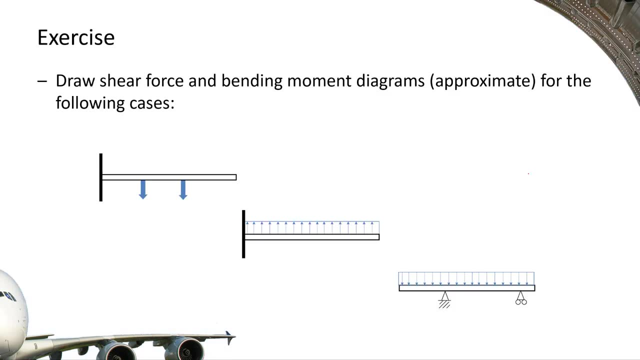 is this structural role? Sorry, my little cursor's not going the right way. Now again, let's do some free body diagrams, But this time we'll start with a free body diagram and we'll look at shear forces and bending moments. 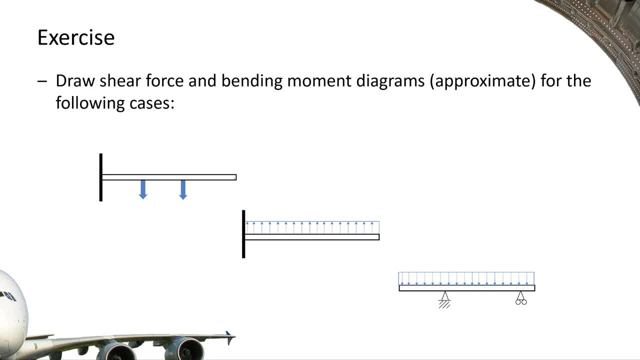 I'm not going to worry about sign convention, but if I have a shear force diagram, it's going to look something like this: Oh, my pen doesn't flip out on me. Okay, Where the point loads are going to create steps in the shear force diagram. 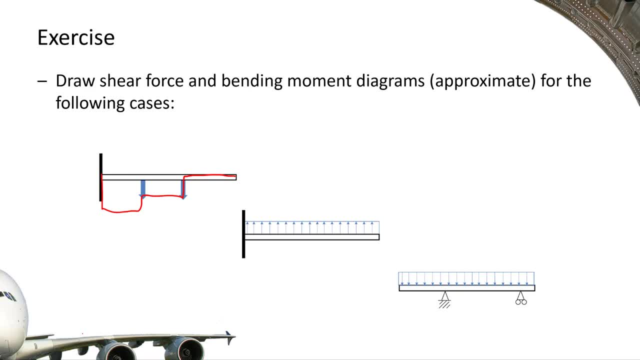 And if I choose a different colour for my bending moment diagram, the bending moments are going to increase linearly and then they're going to increase at a different slope And there'll be zero out here. Now my shear force diagram for this case is going to start at zero. 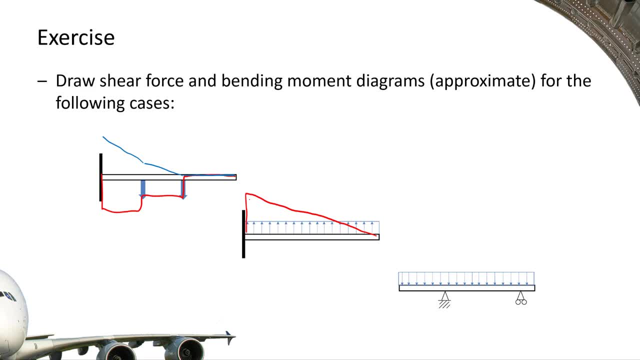 and increase and come down. Okay, Whether it comes down or not is kind of immaterial, because there's always a bit of structure that's experiencing the full load there. And just to be consistent with my sign convention, I'll draw my moment diagram the other way around. 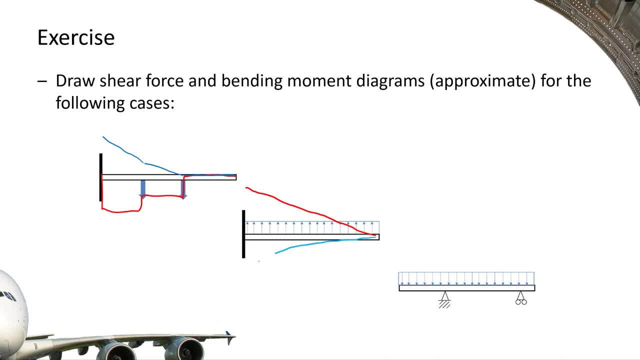 So the moment diagram is doing something like this: Okay, Where it's parabolic, If I've got a linear increase in shear force, I've got a parabolic increase in bending moments. Now, any concerns yet? No, Okay. 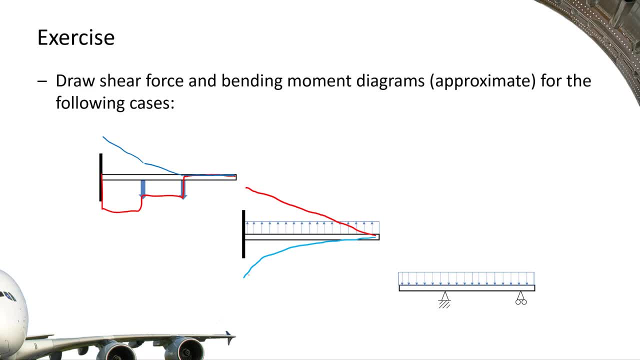 So now for this last case. I'd need to think a little bit about the magnitudes of the distances and the forces involved, but I can do a pretty good first-pass guess of what this is going to look like. I can decrease linearly. 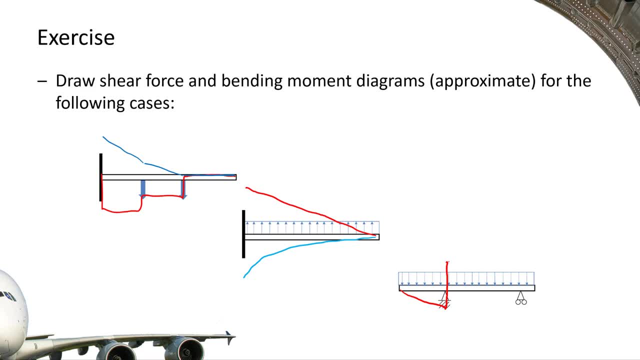 increase where my reaction force is, decrease linearly, increase where my reaction force is and decrease to zero. Now you note, with all of these cases, I've started at a free end. I've started somewhere where I had a pretty good understanding. 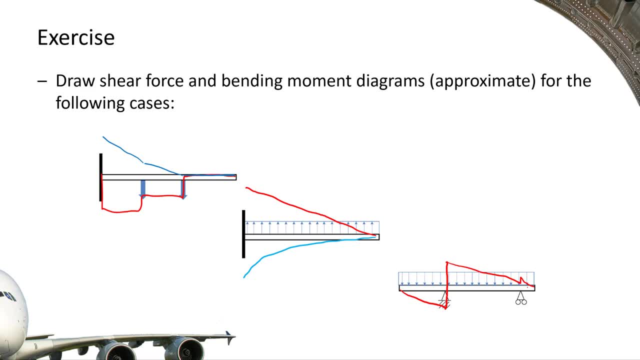 of what the shear force and bending moments are going to be. They're going to be zero at any free tip because there's nothing there that's going to generate forces or moments. Now bending moment diagram for this case is a little bit trickier. 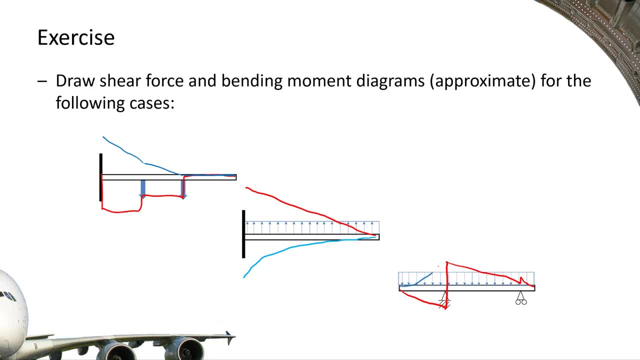 It's going to do something like zero up to a maxima and then Now I haven't done my slopes very well here, but it's going to keep increasing, I think Let me just If I'd drawn my shear force diagram better. 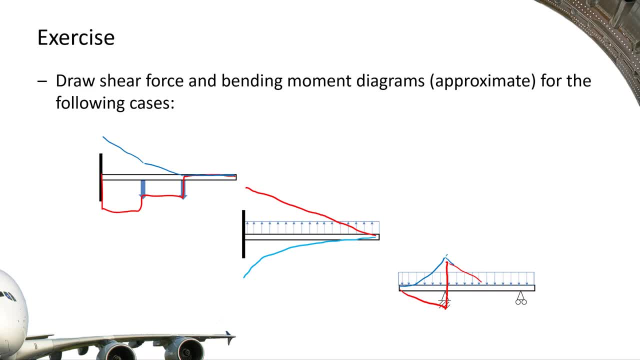 I would have had a better opportunity to do this. Let me just do that. Okay Now, the points at which the bending moment diagram is going to go to zero are ones where we have a summation on the left and a summation on the right that are the same. 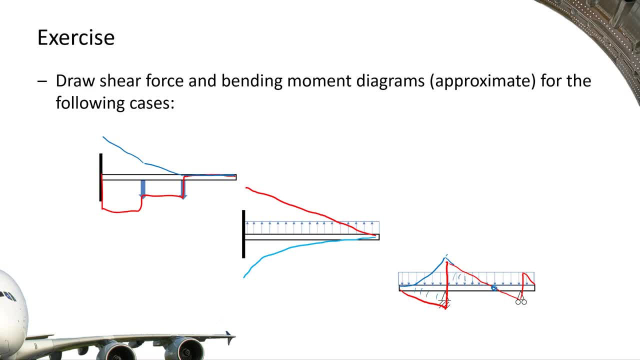 So, assuming that this area here and this area here are the same, then the bending moment's going to come back to zero There, Then it's going to increase again and then go back to zero there. Now that one. There could be mistakes in that. 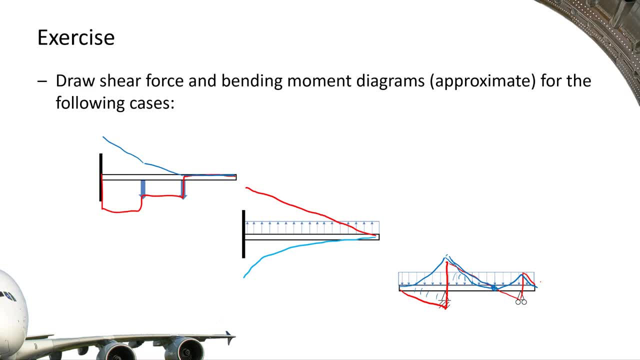 I'm not. The magnitudes and the positions matter a little bit for that one. but you can see, in principle we can very quickly draw some shear force and bending moment diagrams for any configuration and we should know what to expect Now. 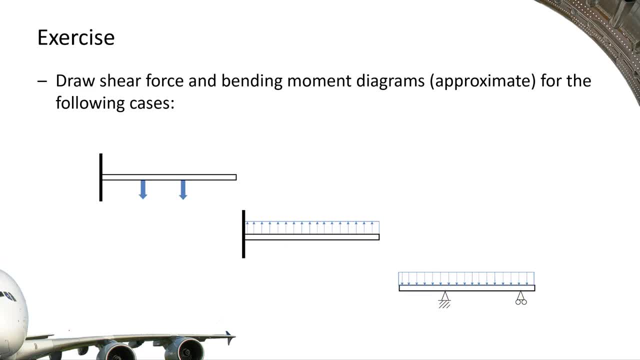 I'll just erase the ink and show you why we would do this. These are just simplified cases of what we might be wanting to analyze, for So the weight of engines hanging off a wing, the distributed lift on a wing and generating lift while it's still sitting on the ground. 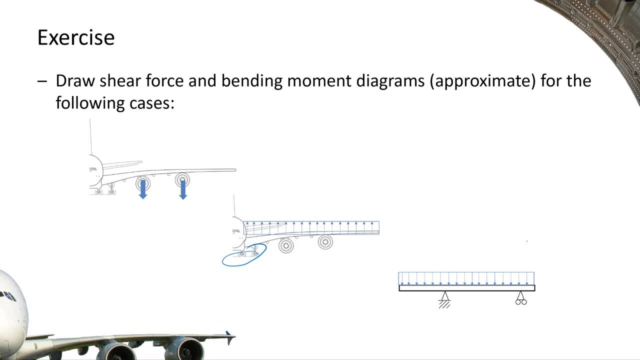 That's a bit of an awkward situation. but Or the wings, The distributed loads on a fuselage, So the wings essentially pick the fuselage up. so you can think of the wings as simple supports for the fuselage. Okay, so those three diagrams we just drew give us 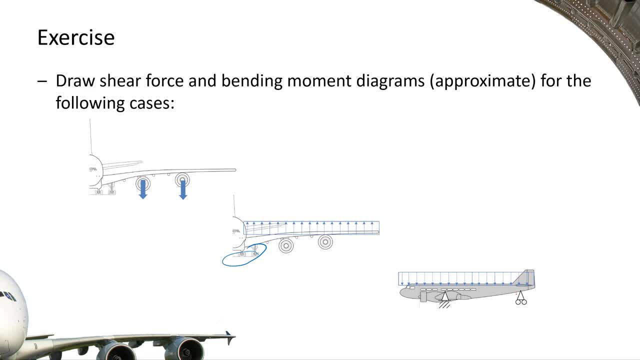 If we treat the fuselage and the wings like beams, they give us an indication of how we might want to generate shear force and bending moment diagrams for those beams, And with those shear force and bending moment diagrams then we can calculate stresses, as long as we can translate between shear force and stress. 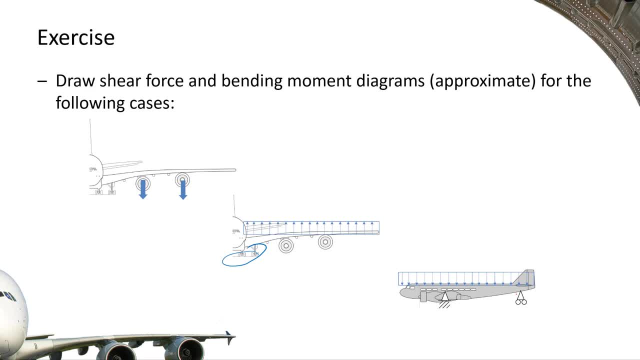 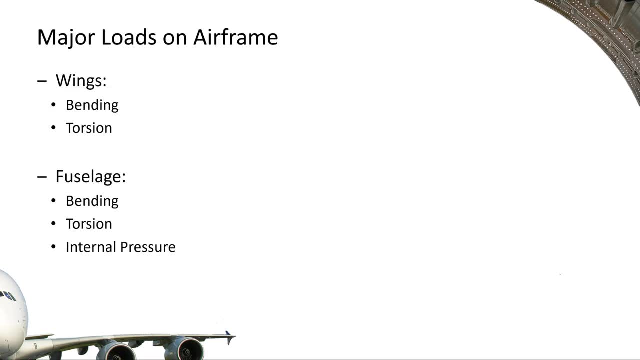 and between bending moment and stress, which is what, in a few lectures' time, we will start to do. Okay, so The primary loads. Now I want to talk about major loads, The things that are generally likely to cause us problems. 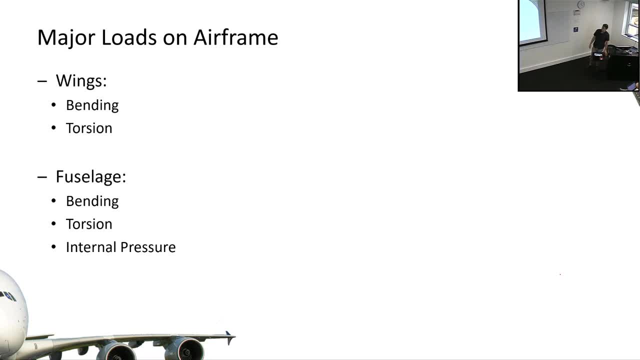 and the things that we have to analyse. for For most aircraft the wings are the critical piece of structure and they take in the most material. So the critical load case for wings is bending. So they're generally very slender and they have to be slender for aerodynamic reasons. 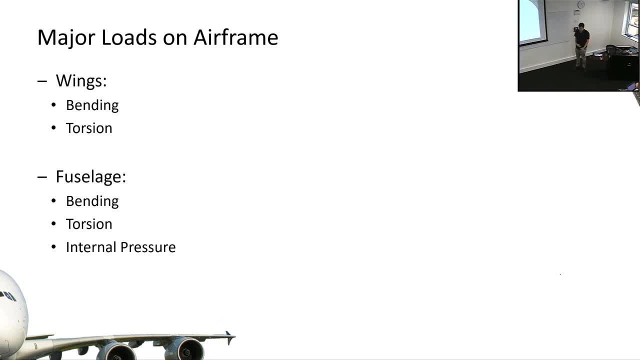 And so the aerodynamicists tell us: this is the shape of your wing and the structures. people say that's really painful, don't give us such a thin wing. And the aerodynamicists say, too bad, make a thin wing. 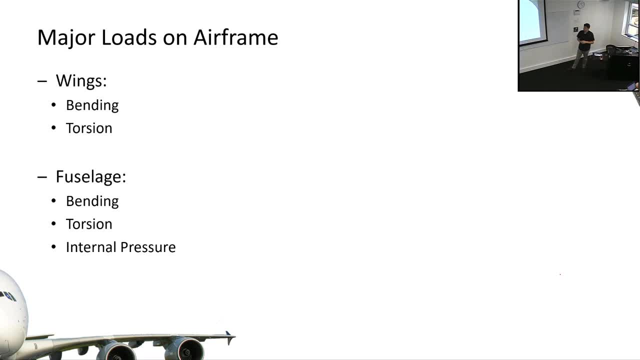 And so your job as a structural engineer is to get enough material in there to make it withstand the loads. But if you think about this really long, slender set of wings or flapping arms, the lift is being generated at a distance from the fuselage. 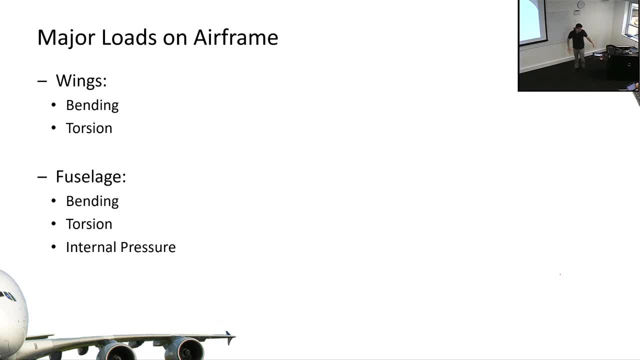 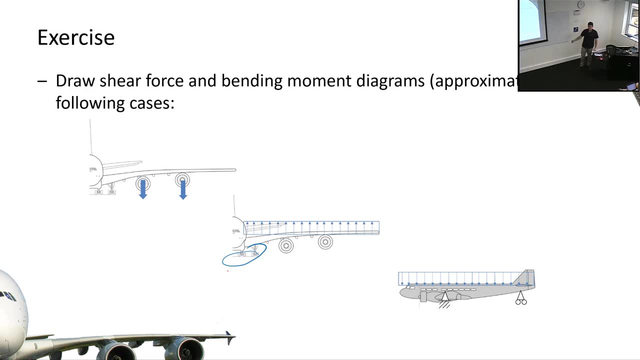 That means that it's generating a bending moment. So if we go back to our bending moment diagram, this one in the middle here, there was quite a large moment at the wing root. So at the root, the inboard part of the wing- 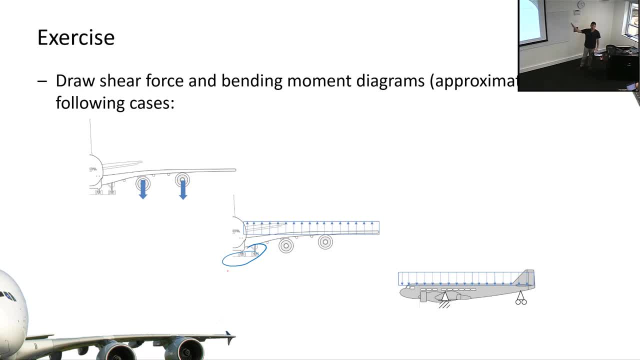 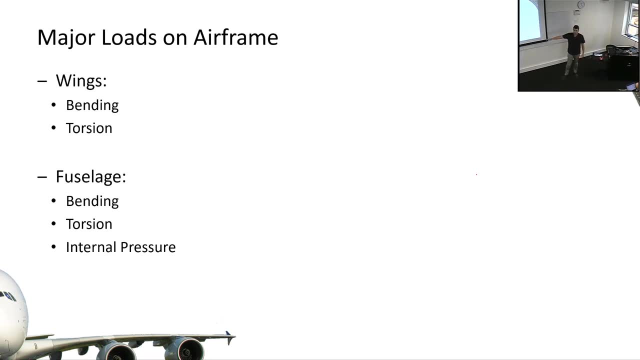 there was quite a large moment. That is the primary load that we have to worry about on wings when we're analysing them. Also torsion. So, as we talked about when we talked about the aerodynamic centre, the airflow generates a moment. 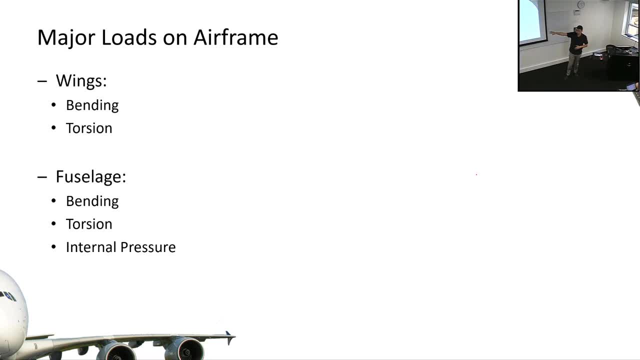 And as you go along, the wing is because it's slender, it's got a fairly low torsional rigidity And so that torsion being generated by the airflow is actually another critical case as well. For the fuselage, bending and torsion are a matter. 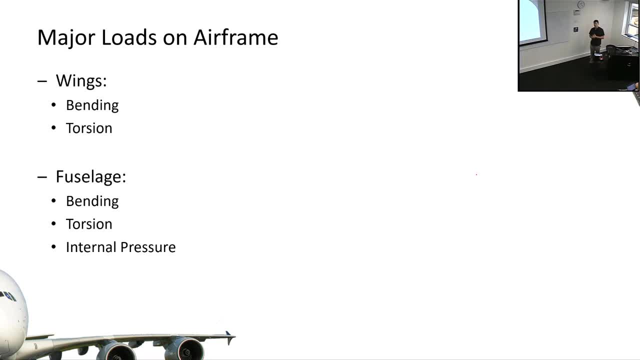 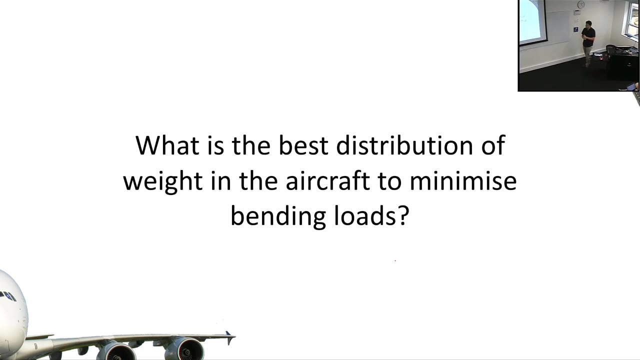 but also internal pressure. So for pressurised fuselages, the fact that we pump it up and are trying to burst it is another critical thing to consider. Now, if we- this is a sort of abstract question that may not be easy for you to answer- 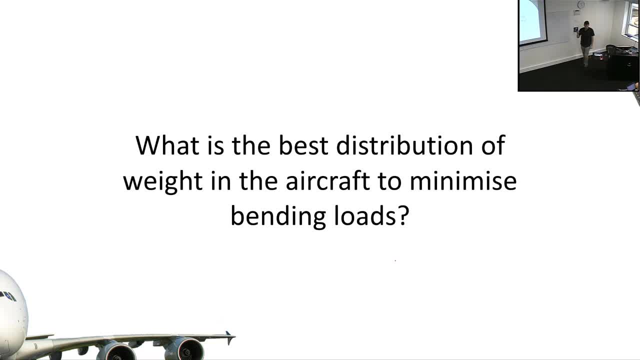 but if we want to minimise bending loads, where do we want to put our weight? So if we had an aircraft and the aim was to minimise bending moments, or even a beam- if we just think about a beam- if we wanted to minimise bending moments, 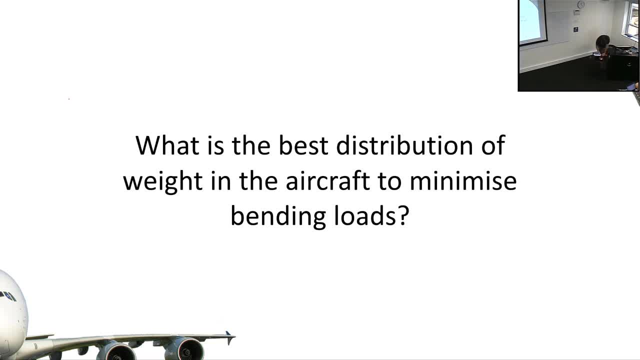 OK, let me just draw a little picture. Let's have a wing here, It's got an engine hanging off it, OK, and it's got some lift distribution And a point load for where the engine is. Now, if we wanted to add, 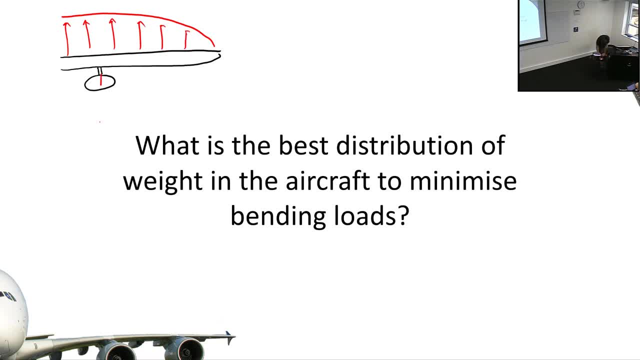 say we had some discretion about where our fuel was going to go. where do we want to put the weight? to keep the bending moment as low as possible? Further out The wing, Yeah, So we're really trying to put our weights where the lift is being generated. 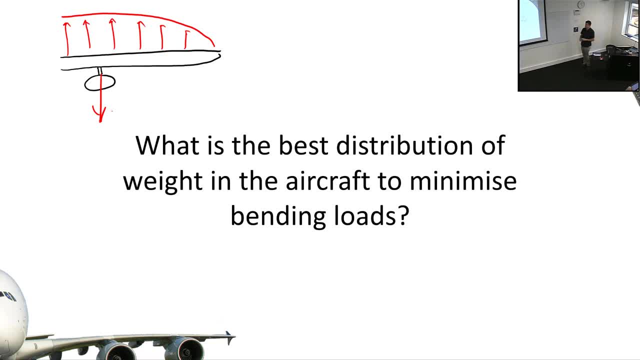 So to be able to put the weight where the lift is being generated. So we're really trying to put our weights where the lift is being generated So to balance it out like immediately. So the further out we can get the weight. 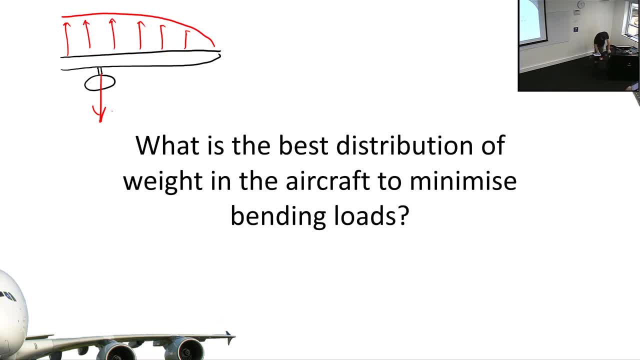 the lower we can keep the moments. So if we think about this in its current configuration, there's going to be quite a sizeable bending moment near the root. but if we put a bunch of distributed weight in for the fuel then we can offset a large amount of that bending moment. 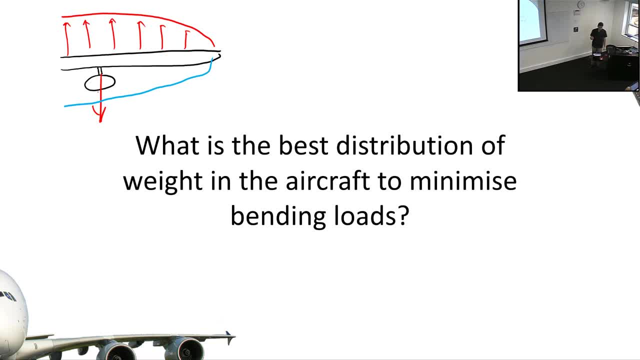 And this is what we call wing relief, and we'll talk about this a little bit more in this lecture. But anything we can do, where we can get weight out, where the lift is being generated, the moments come down. The big problem with aircraft: 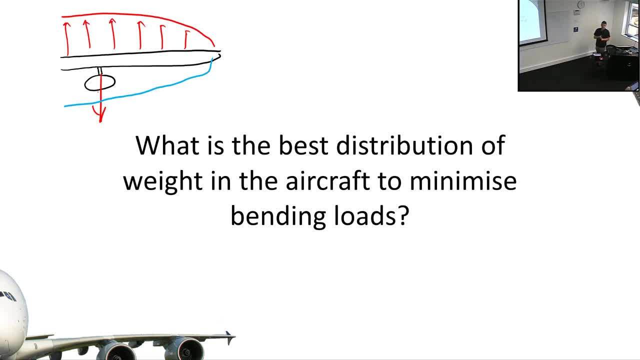 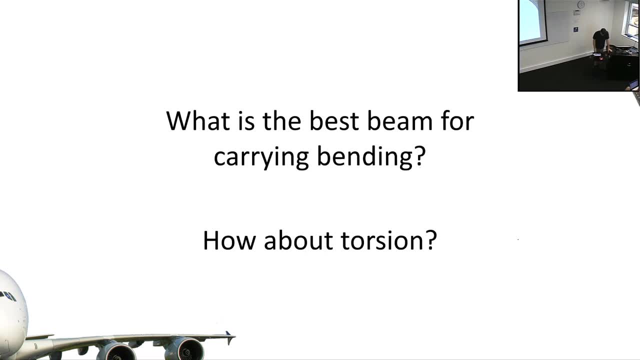 is that the lift is being generated at a distance from where the weight is, and that generates large moments. So getting rid of those is really important. Now here's a question that you would have come across in. Well, the first question, at least in second-year mechanics. 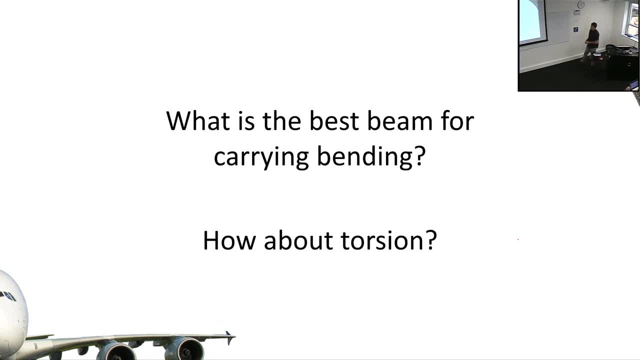 What's the best beam configuration for carrying bending moments? I-beam- yes, Everyone's heard of an I-beam. I may have just given away the answer to the second one. What about torsion? What about a beam that's being loaded in torque? 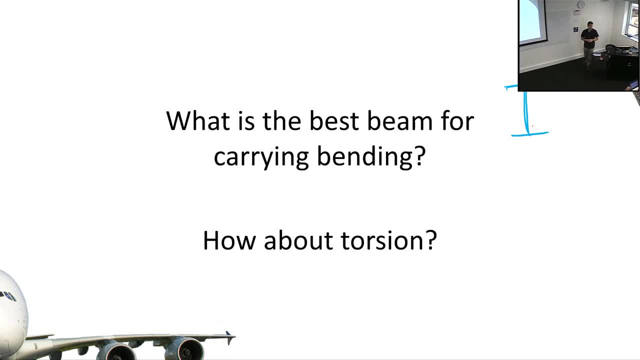 which we probably should call a shaft. What do we want to do with a shaft Circular? Is there anything particular about A hollow circle or a solid circle Hollow? yeah, So we want a thin-walled hollow tube, which I'm not used to actually drawing wall thicknesses. 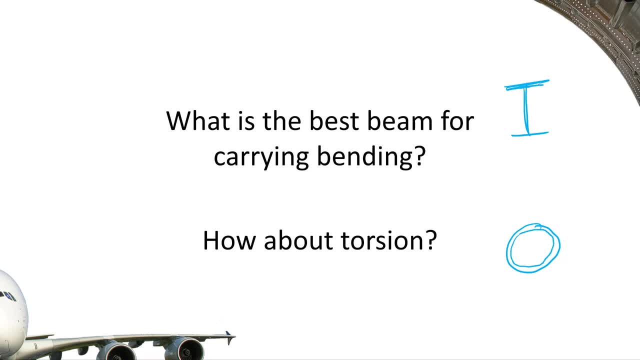 As we'll see through this course, there's no real reason to draw wall thicknesses for most of what we do. When we think about beams and shafts, we're going to try to abstract our aircraft into these kind of classic engineering cases. 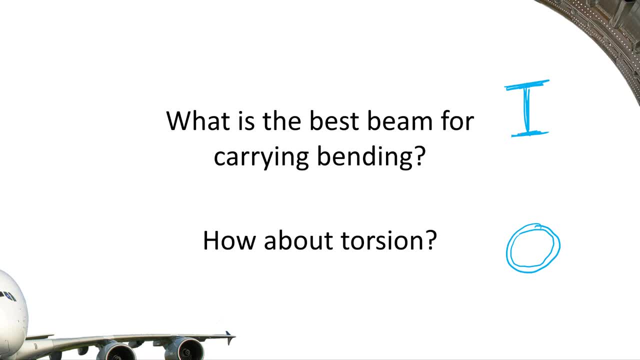 We want to think about our aircraft as beams and shafts as much as possible, because then it gives us the tools that we need to do the analysis. So if we wanted something to carry bending, we want an I-beam. If we want something to carry torque or torsion, 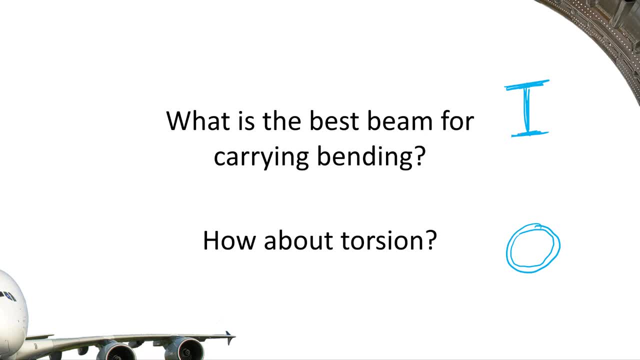 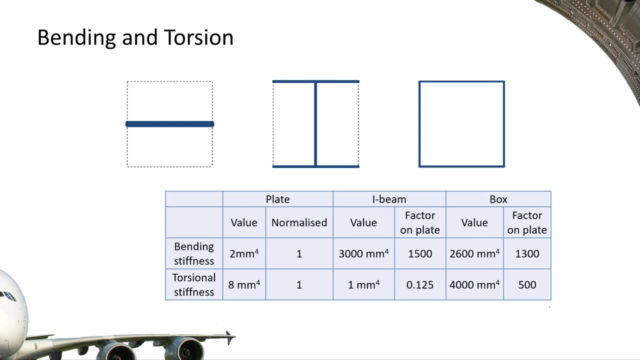 we want a tube. Let's do a bit of of a back-of-the-envelope calculation, So this analysis takes the same amount of material. So there's a box that I'm putting that material inside which is dashed, And then I have considered a flat plate. 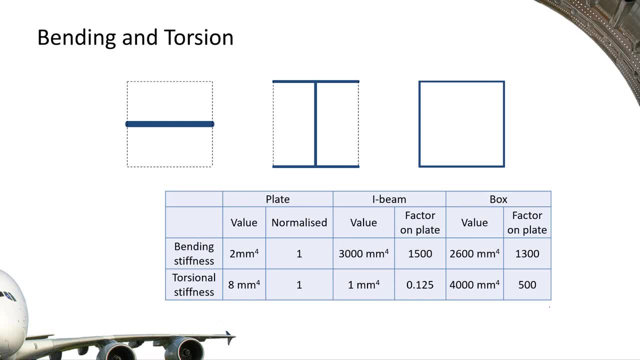 an I-beam and a square box And the amount of material is constant. So this thickness here T-plate is, And if we call this T-box, T-plate equals 4 times T-box. So I've distributed the same amount of area. 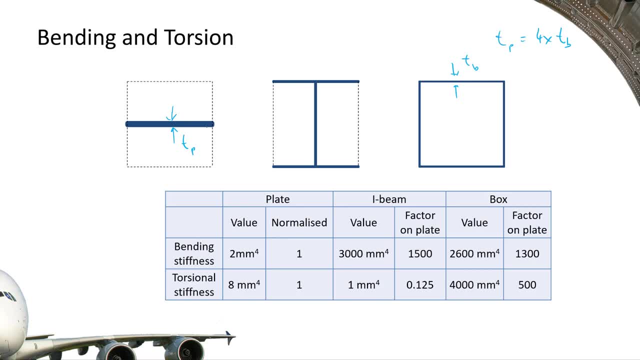 to these sections. So this one's a bit thicker, The plate's a bit thicker and the box is a bit thinner. So they weigh the same, essentially The bending stiffness of the. We normalize the bending stiffness and we can do that through I-X-X. 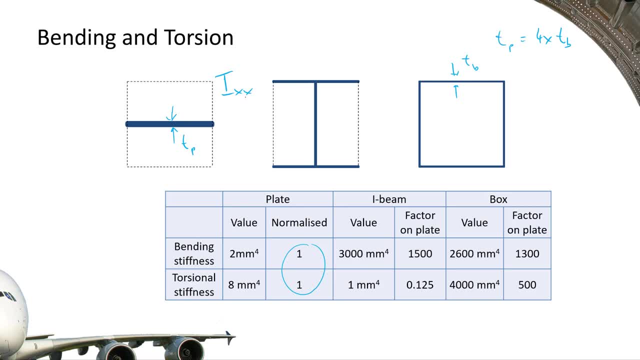 I-X-X is a measure of our bending stiffness Then the I-beam is 1,500 times stiffer in bending than the plate, But the box is also 1,300 times stiffer, So it's still pretty good. 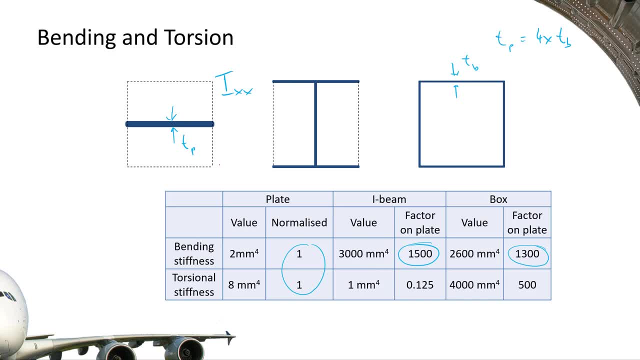 If we look at the torsional stiffness which we can do with our polar moment of inertia, the polar moment of inertia for the Oh sorry. polar moment of area for the I-beam is actually less. It's an eighth of the flat plate. 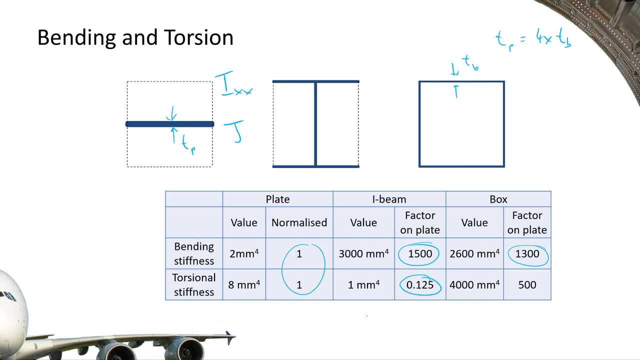 So the I-beam has got a lower torsional rigidity than the flat plate does, But the box has got 500 times the torsional rigidity of the flat plate. Okay, So what we can see if we've got structures that are loaded. 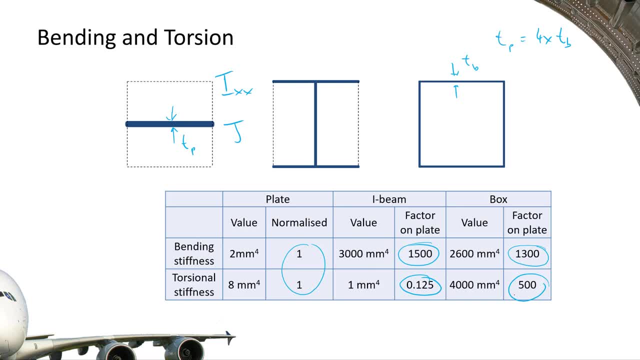 in both bending and torsion, which wings and fuselages are. we want hollow, thin-walled sections. We want stuff that's got a lot of space in the middle, lots of material out near the edge, and that gives us the best case. 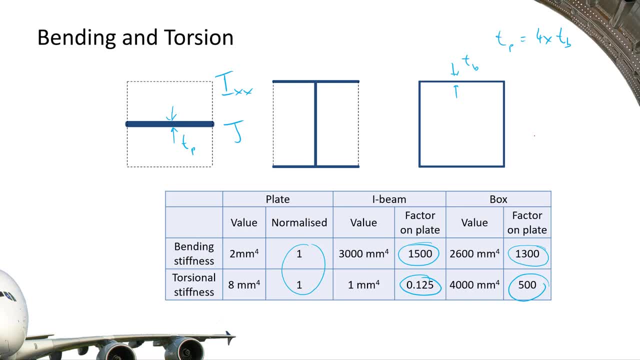 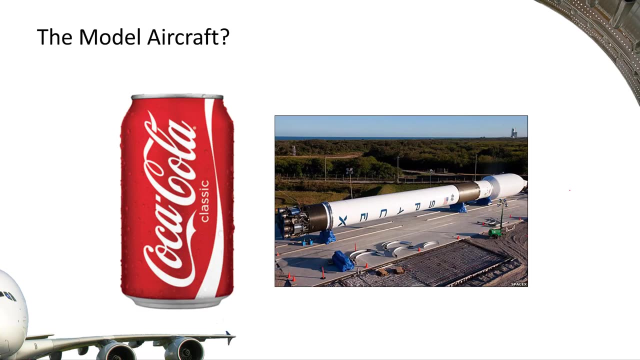 for carrying bending and torque. And if you look inside most aircraft that's exactly what you've got. You've got a lot of material in the skin that's carrying loads and not much in the middle. So a classic aircraft, the one that would give us 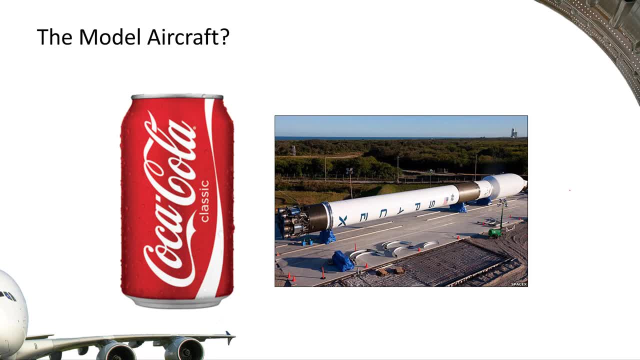 the most efficient possible structure. I mean it's a Coke can, really something that's a thin-walled structure with maximum distribution of material to the outside. It's the best balance of torque and bending and direct load carrying that we can have. 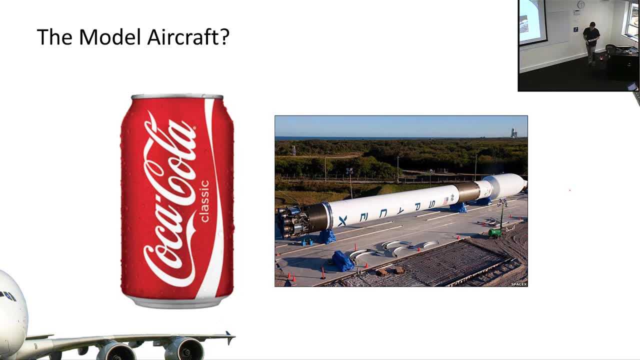 And the engineering that goes into a Coke can is pretty insane, But the we can't use those kinds of structures in many applications. Even this rocket, which looks like it'd be a perfect application for a thin-walled structure, has got lots of internal reinforcement. 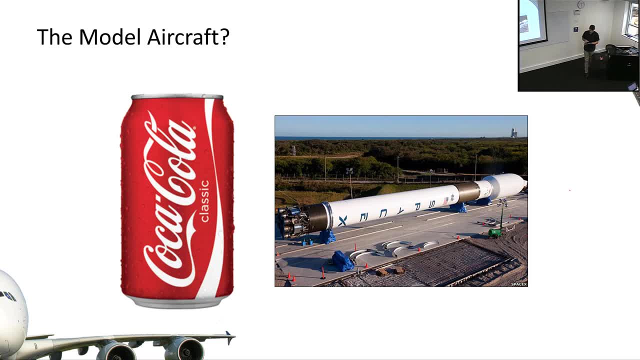 And we'll talk about why that is in just a second. But has anyone seen that thing that people do as kids, where you can stand on a Coke can and it can pretty much take your entire weight, except as soon as you put the slightest little defect in it? 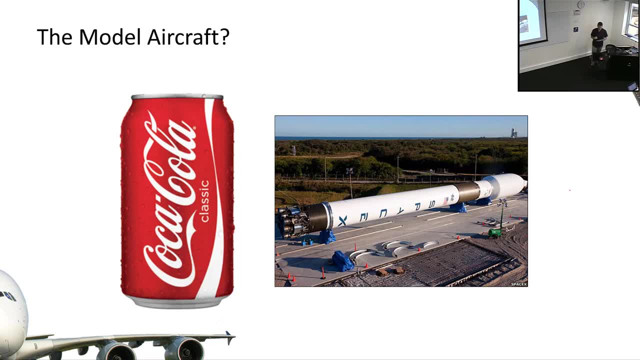 it collapses to nothing. If you've got a pure Coke can, it'll easily carry 100 kilos empty and probably like 300 kilos full. But as soon as you put a little defect in the wall, that drops to next to nothing. 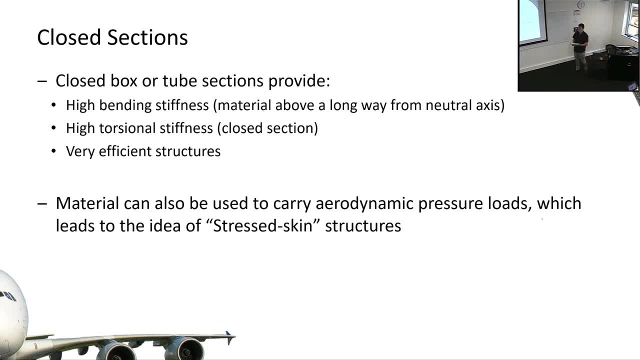 So these closed box sections or tube sections have very high bending stiffness, very high torsional stiffness and they're very efficient. And they're also very good at carrying pressure loads. So aerodynamic pressure loads, Because the skin on the outside is the same thing that's carrying the pressure loads. 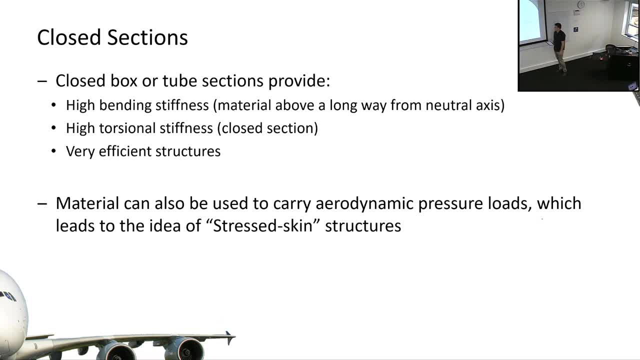 and it's also carrying the structural load. So this concept of putting the skin of the material being the load-bearing part of the structure is what we call stress skin design. So we don't have a frame and then a parasitic facade on the outside. 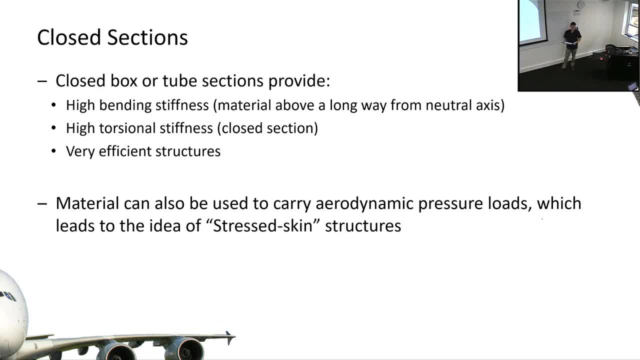 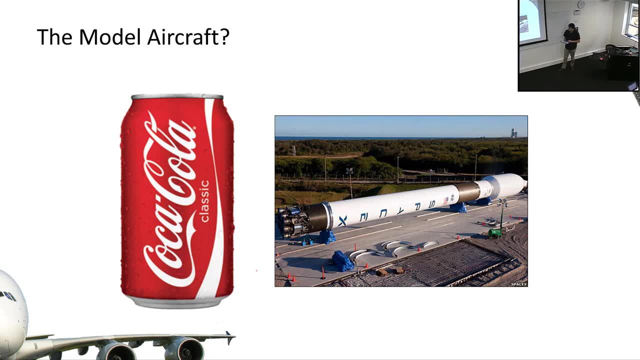 The skin of the aircraft is actually carrying the loads, So that's what we call a stress skin design. Now, just as a little point of interest, a Coke can. if you scale a Coke can up to the size of a 747,. 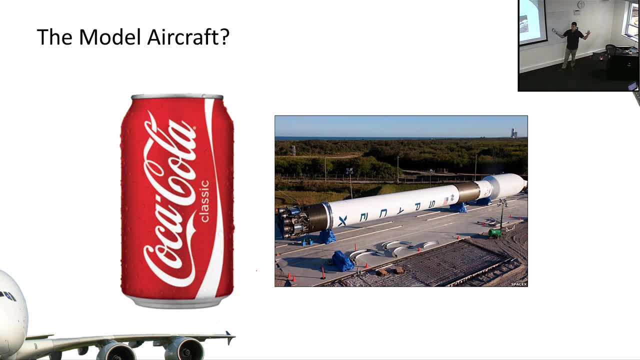 so you just took the aluminium can and made it as big as a 747, which a 747 is really an aluminium can as well. the wall thickness of the Coke can is thicker than a 747.. So think about the relative wall thickness of an aluminium can to its diameter. 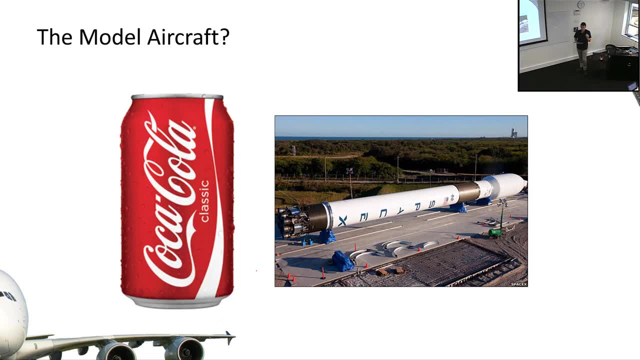 A 747 and other aluminium aircraft have thinner walls than that. relative to their diameter They're very, very thin. There's probably only for most of the fuselage. there's only about 4mm of aluminium between you and the outside wall. 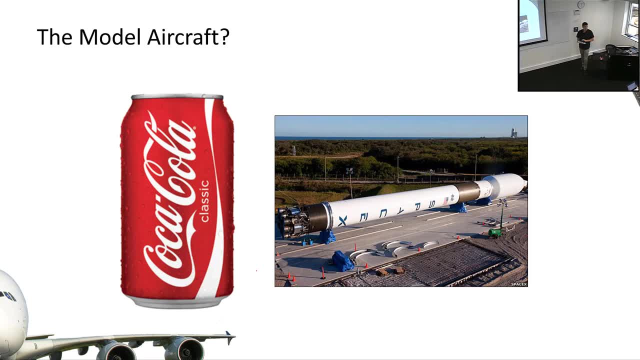 There's not much there at all. There's other reinforcement which we'll talk about, But in terms of carrying pressure loads and like if you really wanted to get something and stab a hole through it, then there's not much material there. 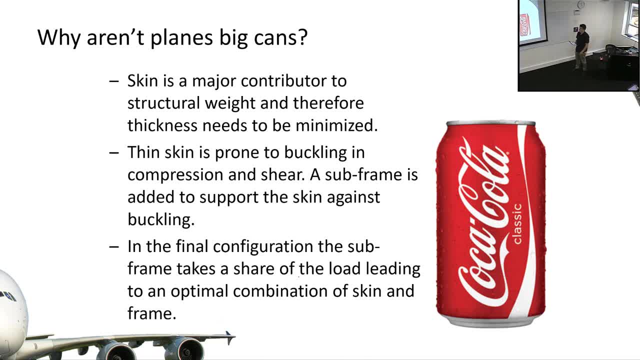 So this sort of logically takes us to the point: well, why don't we have aircraft that are just big cans? Why do we have this internal structure that you will see inside some aircraft? Well, the driving force to make them like aluminium cans. 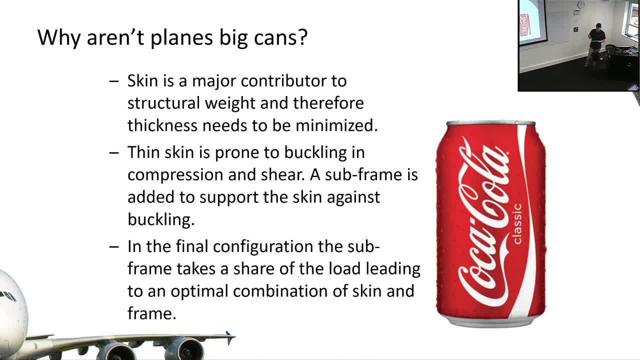 is that the thickness needs to be minimised. It's a big contributor to structural weight, But as it thins out it gets more and more prone to buckling, And buckling is something we won't talk about until late in the semester. 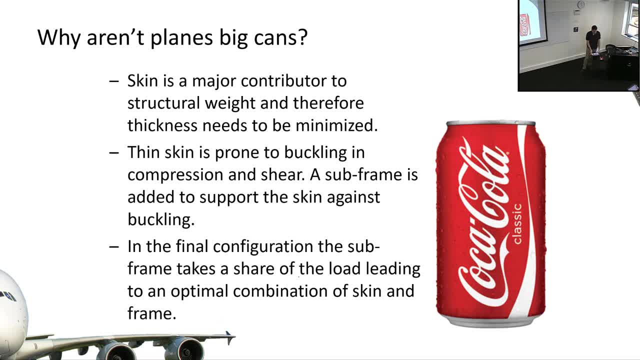 but it's an instability. So if you take a bit of paper in your exercise book or a plastic ruler or something that's fairly thin in tension, it's actually surprisingly strong, Like a piece of paper is really strong. A piece of paper is really quite strong in tension. 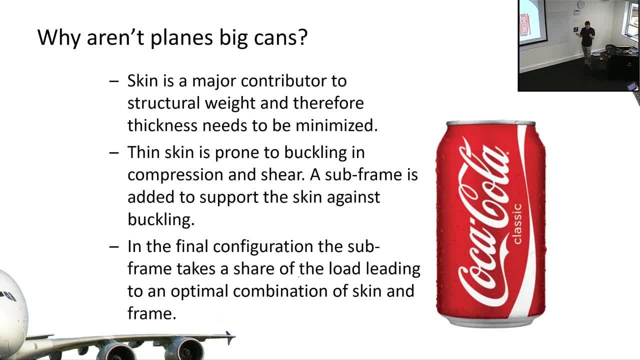 and it's really quite strong in shear. But the second that you apply any compression to it it doesn't fail. The material doesn't break, but it's got no stability. So if you take your exercise book and just collapse it like that, 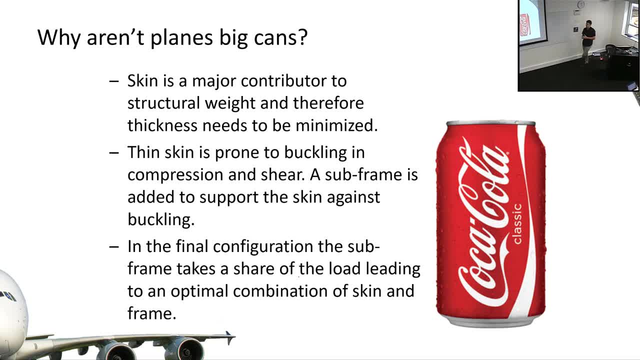 it'll just buckle. The material's not breaking, but it's just got no ability to withstand any load. And this is exactly the same as what happens with aircraft structure: As we make them thinner and bigger, they become very, very susceptible to buckling. 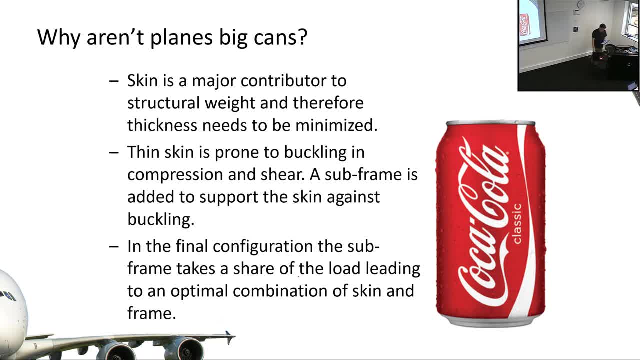 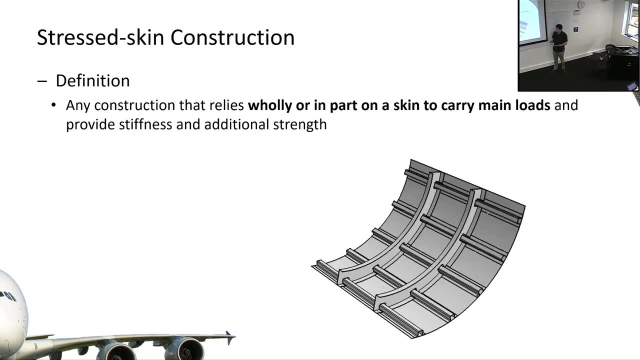 and also other failure modes through buckling, which we call crippling. So what we end up doing is putting an internal structure in to support against buckling and we find the optimal combination of skin and frame, And this is what we end up with. 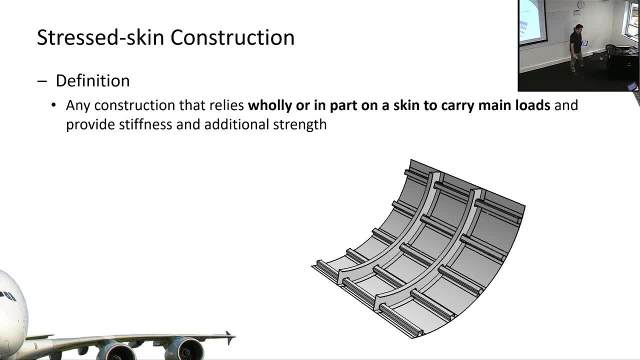 is something we call a stressed skin construction, And this is not how aircraft are always made, and there's still a lot of aircraft that don't use this design paradigm, but most of them do. Most big aircraft do So. the definition of this term. 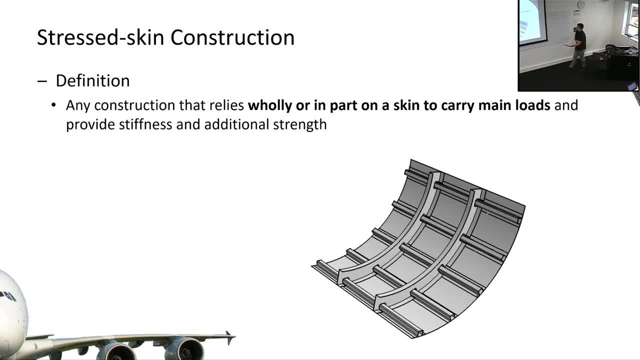 is that any construction that relies wholly or in part on the skin to carry the main loads and provides stiffness and additional strength. That's what we call a stressed skin design. So this is a cutaway part of a fuselage You'll have longer ons. 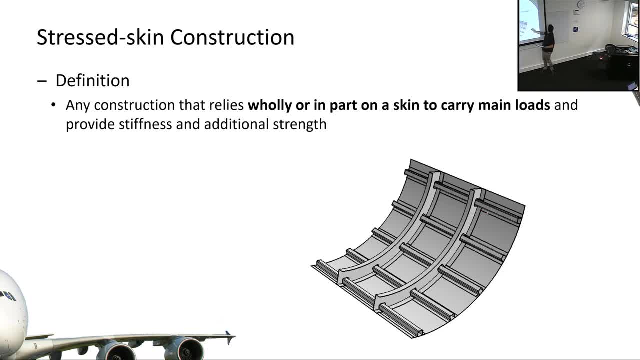 skin and frames. and don't worry about these names, We'll talk about them in a bit, about what they all mean. But the combination of area: there's roughly as much area in all of these longitudinal stiffening members as there is in the skin. 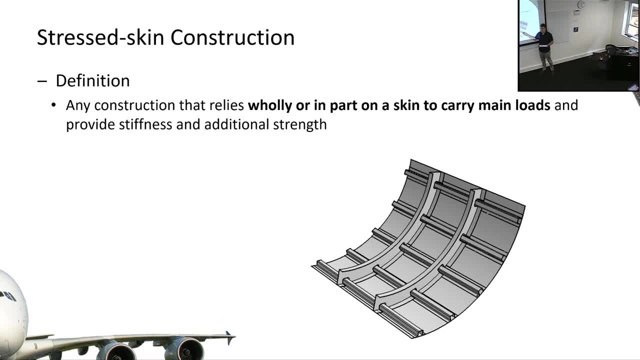 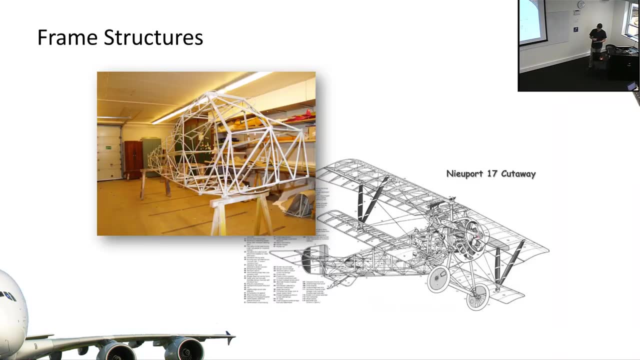 So it's about a 50-50 mix of material in the subframe and in the skin, and they're both sharing the loads, And it's that combination that ends up with the best configuration for us. So historically, aircraft weren't always built that way. 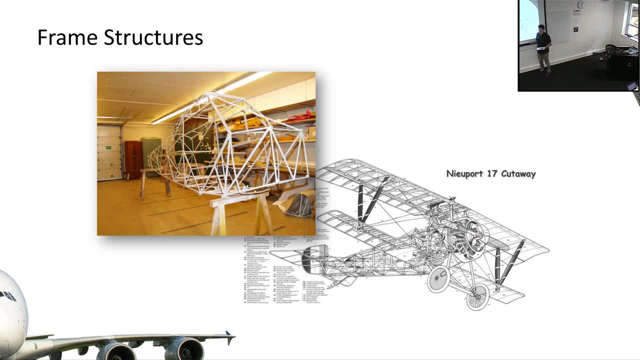 And even to this day there are still quite a few frame-type structures inside light aircraft. The original aircraft came from bicycle manufacturers. So the Wright brothers were bicycle repair people. They thought like bicycle people. they built bicycle frames and they put skin around them and made an aircraft. 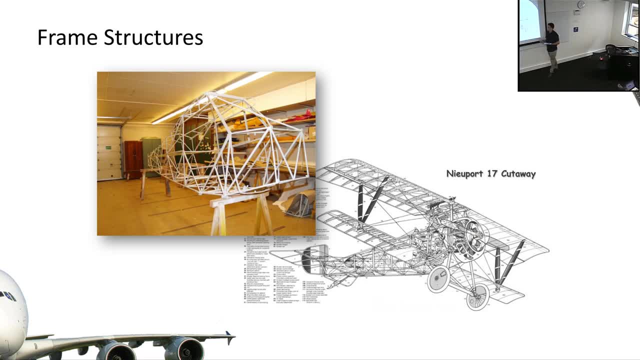 So they had these space frame kind of configurations And the load in these space frames is carried as direct forces. So it's either tension or compression in a member And the skin on the outside was just parasitic. All it was doing was either providing a surface, 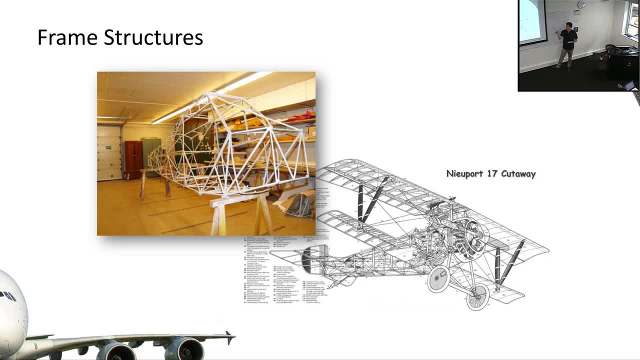 so that it minimized drag or providing a surface to take the aerodynamic pressure and put it into the frame And, as a result, all of the weight of the skin is just subtracting from the performance of the aircraft. On the plus side, it's easier to make more damage-tolerant structures like this. 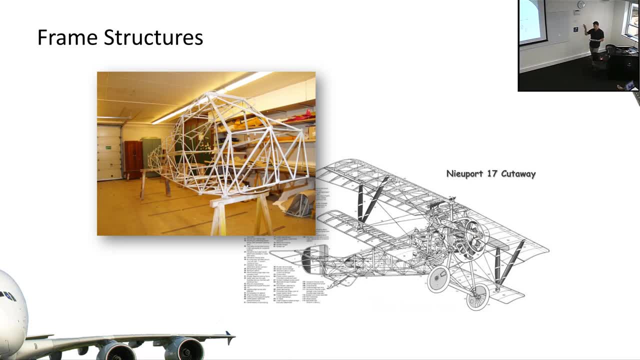 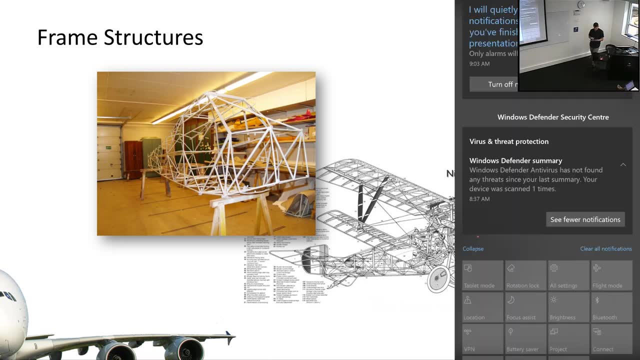 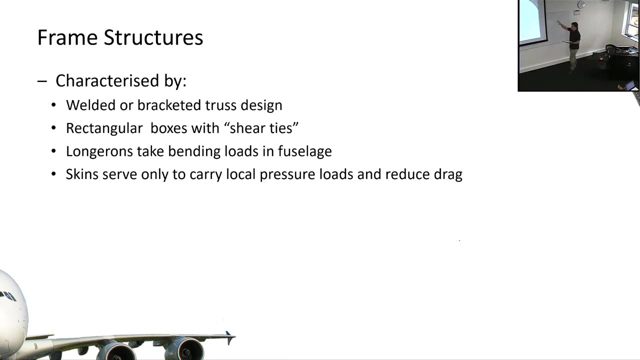 You can make a redundant truss that if you poke holes in your skin, you're not really degrading the performance of the airframe very much. Now, the characteristics of these type of aircraft is that they're generally welded or bracketed trusses. 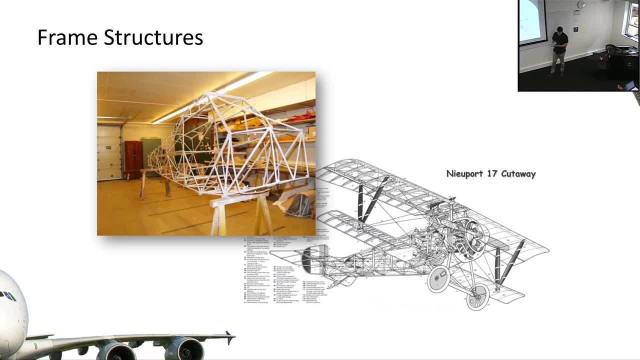 They'll have regular box shapes. So if you look along here, my pen has gone AWOL. No, it hasn't. They're a regular box structures. You'll see these repeating boxes And then they'll have shear ties. So here you can see them as well. 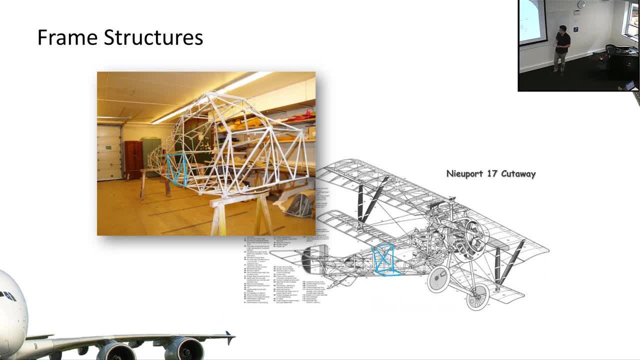 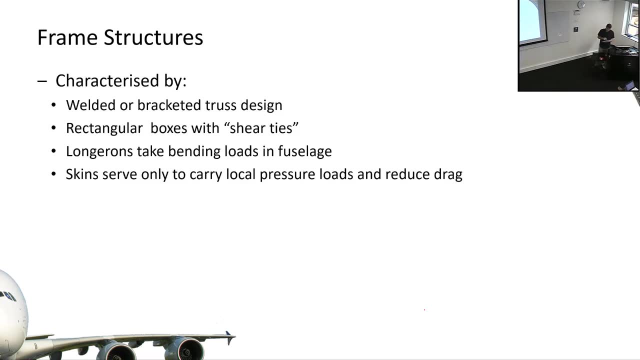 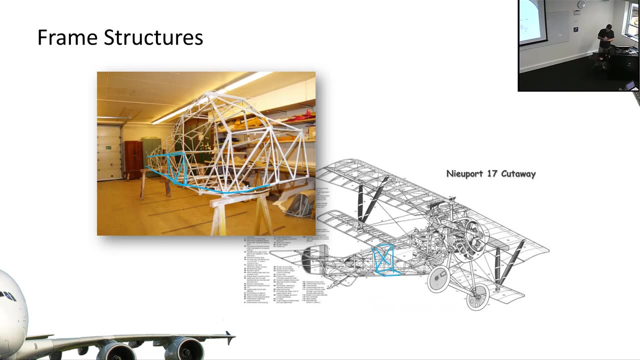 There are box structures here And then they'll have shear ties in them to withstand the shear loads And the longer ones take bending into the fuselage. So if you see, here there are these longitudinal members that are taking most of the bending moments. 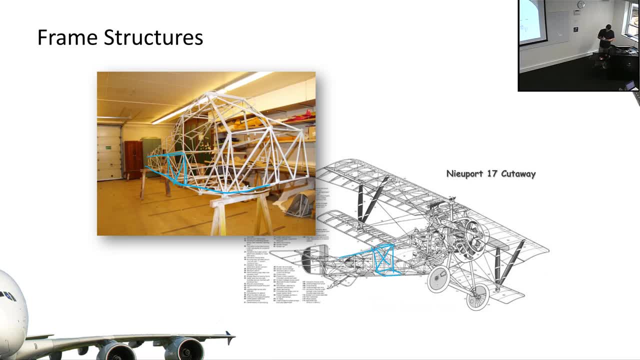 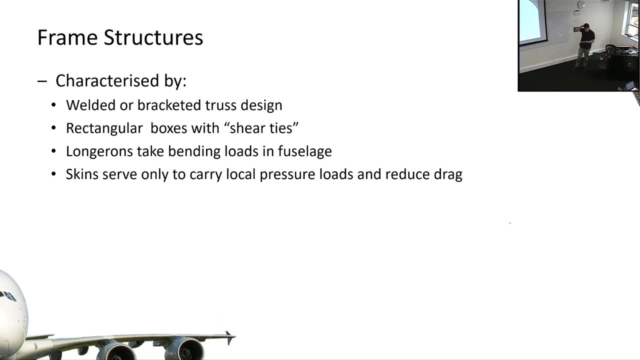 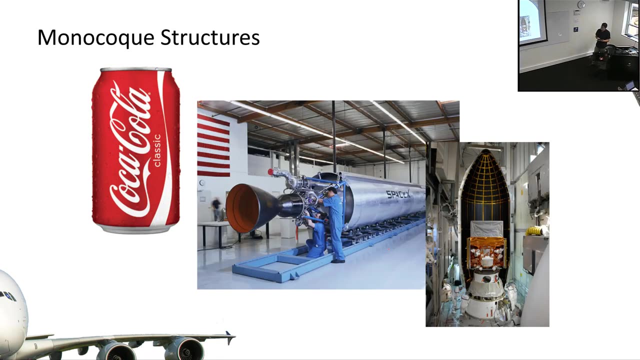 in the airframe And here longitudinal members taking the bending moments, And the skins are parasitic and they're only carrying local loads. Now the exact opposite end of the spectrum are monocoque structures, And monocoque is a pretend French word. 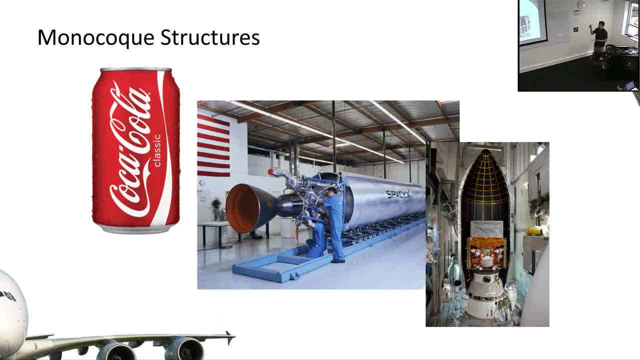 I don't remember who coined it, but they thought they were making up a French-sounding word. It essentially means single shell, So balloons, for instance, are monocoque structures because all of the load is being carried in the shell. 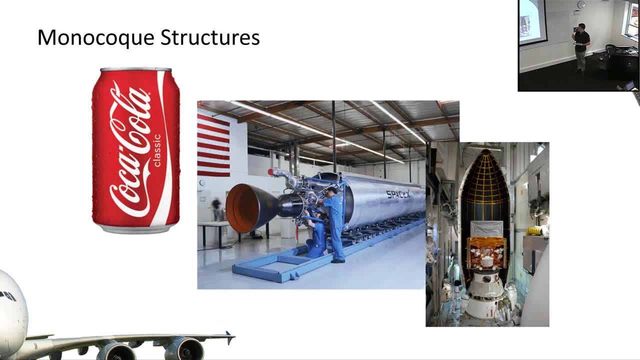 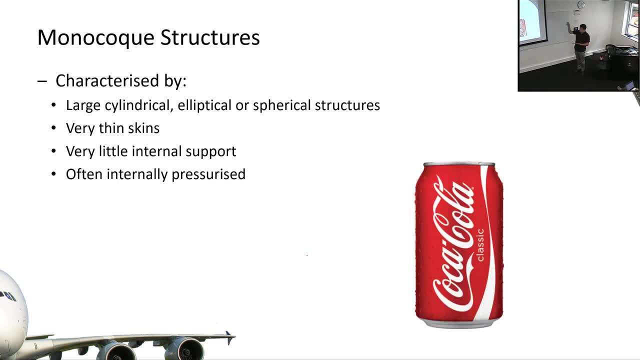 A Coke can is a monocoque structure. Some space components- rocket components- are monocoque structures, But they're characterized by large cylindrical, elliptical or spherical structures with very thin skins And very little internal support, And normally they're internally pressurized. 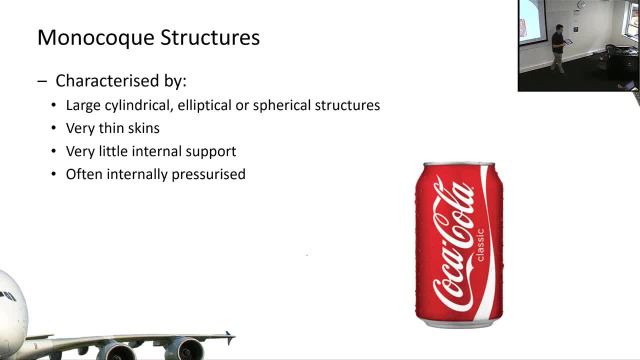 Most of the strength of a Coke can in transport comes from the fact that it's internally pressurized. They're extremely efficient, but any cutout, any hole in the can or any change in geometry needs to be heavily reinforced. So if you look at the top of the can, for instance, 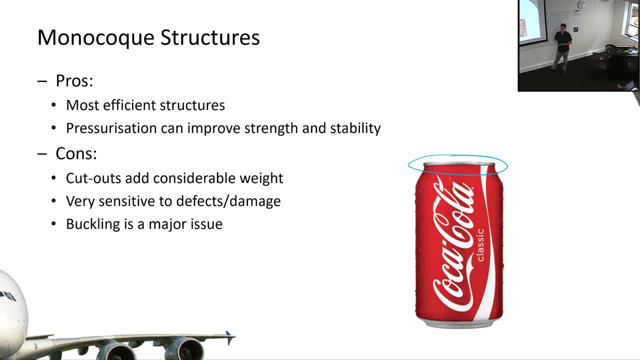 where the opening is. there's a lot of extra material and extra reinforcement where that opening is in order to carry the loads, And at the base, where the geometry changes again, it's much, much heavier. The walls of the can are significantly lighter. 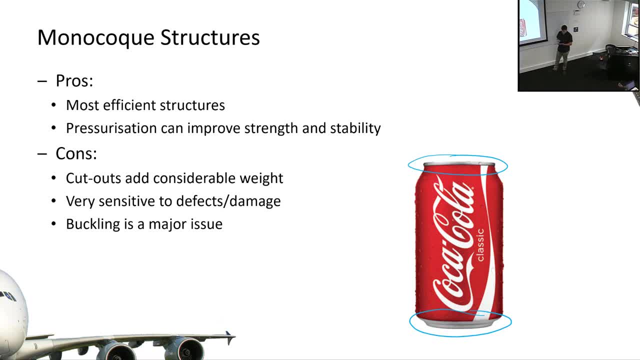 than the top and the bottom put together, And so anywhere we need an opening and unfortunately aircraft need a lot of openings. you have to have lots and lots of reinforcement, So it degrades the benefits of having thin monocoque structures And buckling is a big issue. 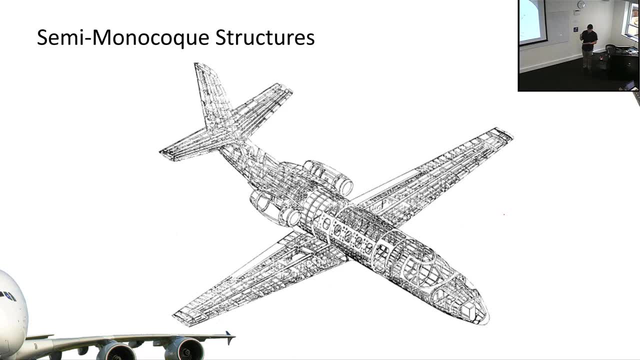 Any defect and you lose strength massively. So the compromise and what you'll see in nearly every aircraft out there at the moment that's of a reasonable size- light aircraft maybe not- are semi-monocoque structures, And semi-monocoque is just semi-single-shelled. 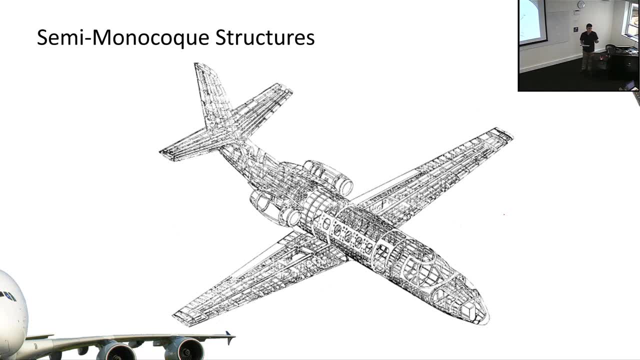 where we have a subframe and a skin and they're both carrying loads together. They're give or take. for a structural component like a wing, about half the weight will be in the subframe and about half the weight will be in the skin. 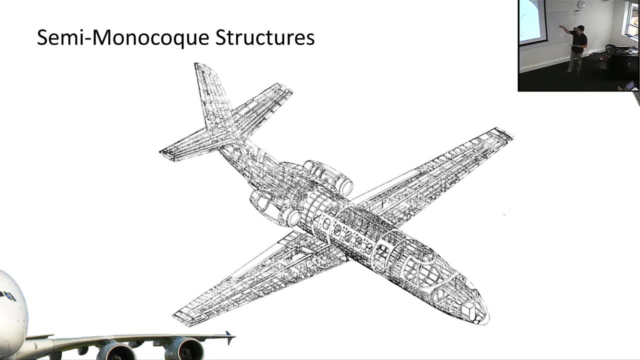 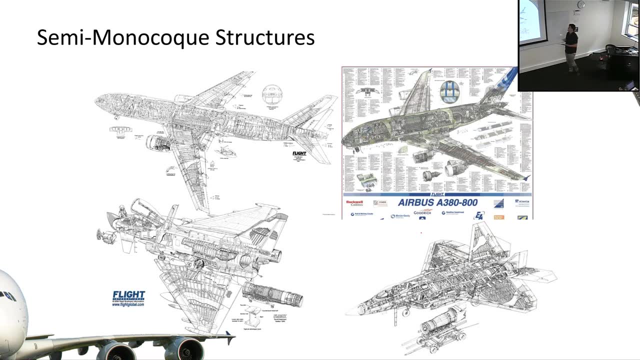 So a bit more in the subframe because there's other things that it's doing. If you look up any aircraft cutaway and you can find these, there's sort of Flight International, Flight Global. you can just Google aircraft cutaways. 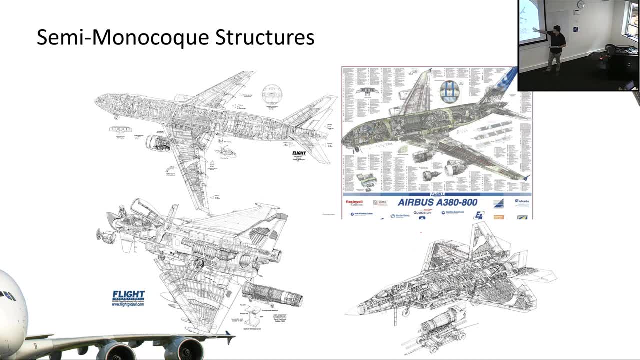 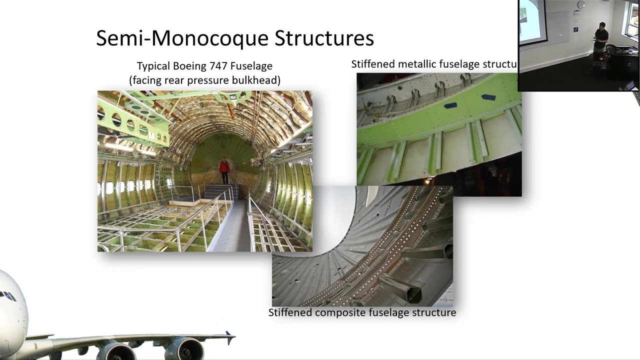 you'll see the same setup. You'll see subframe with a skin on top. So these are some examples. This is the inside of what a 787 looks like. This is the inside of a 747. And I don't know what that one is. 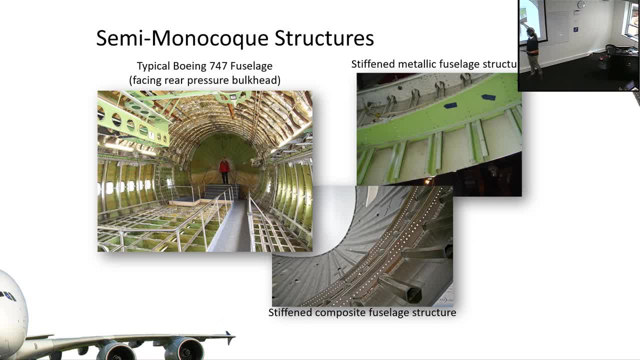 I think that's a picture I took. I didn't take that picture. I have no idea what that aircraft is, But you can see if you look closely. here there's longitudinal stiffening members running the length of the aircraft, frames running around the diameter. 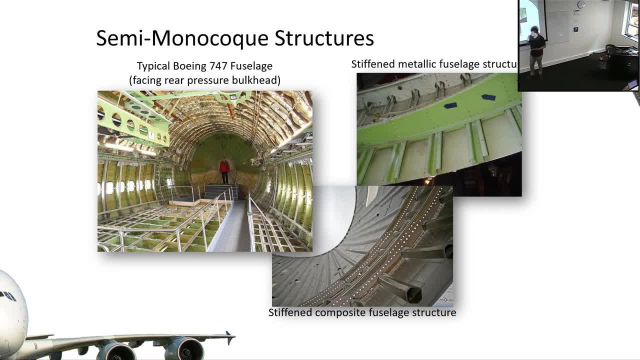 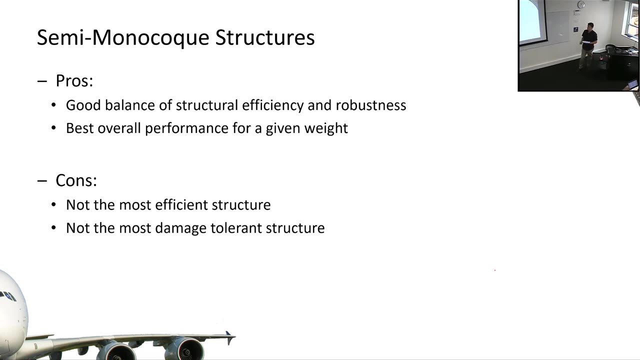 Again here longitudinal stiffening and frames and a skin And all of those are acting together to carry the flight loads. They give us the best balance of structural efficiency and robustness and the best overall performance for a given weight. The negative is it's not quite the most efficient structure. 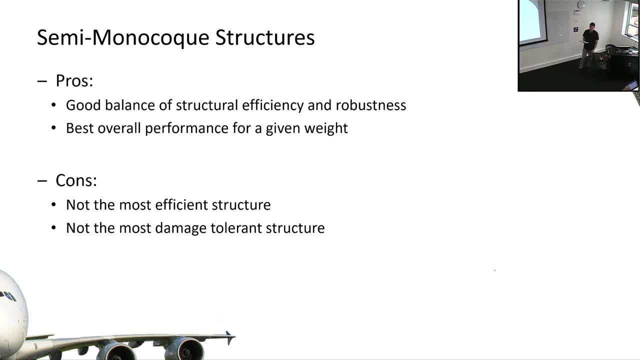 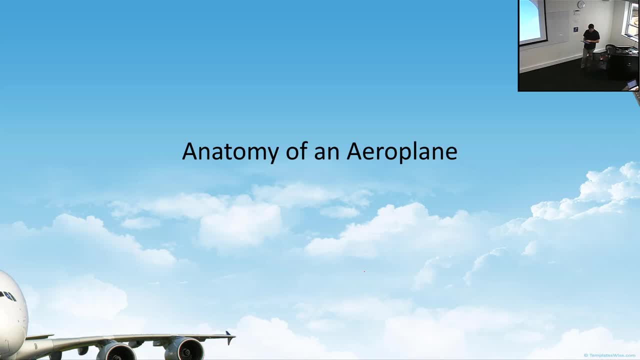 It's not quite the most damage-tolerant structure, But it's the best combination. All right, another little activity, because I know for most of you- unless you've been a plane nerd your entire life, and I wasn't when I came into aerospace engineering- 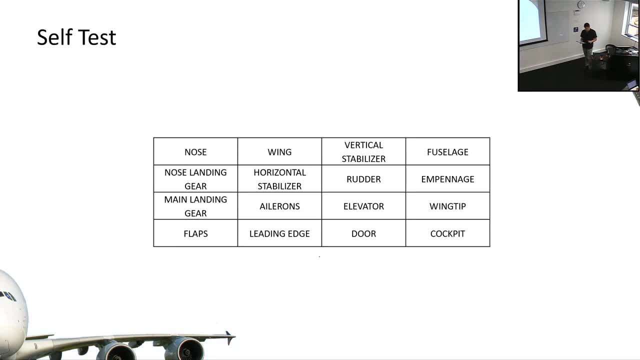 you may not be familiar with some of the terminology. So if you've got the notebook, copy this out of the notebook. Otherwise, just take down these 16 labels. Now there's going to be some ridiculous ones in there, like door. 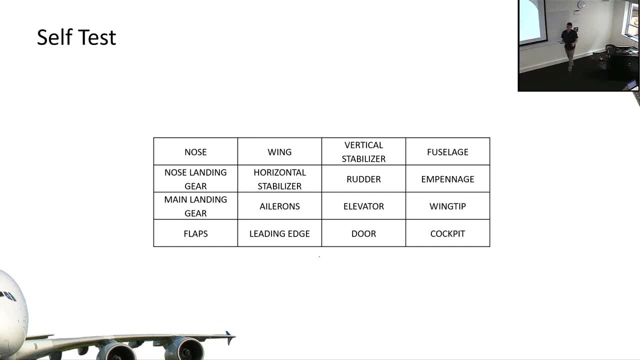 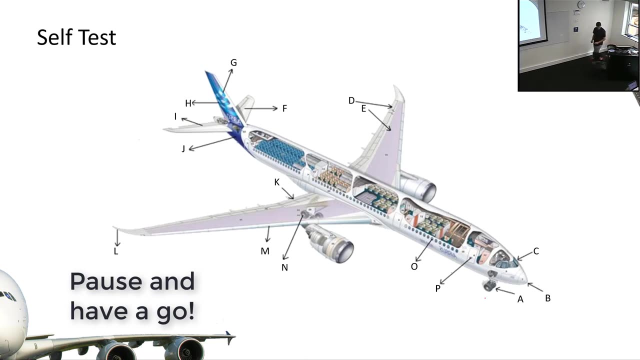 But I needed 16 to make a nice grid. So take down the labels. In a minute I'm going to show a picture of the aircraft And then you can start sticking the labels on the aircraft. Here's your picture of the aircraft. 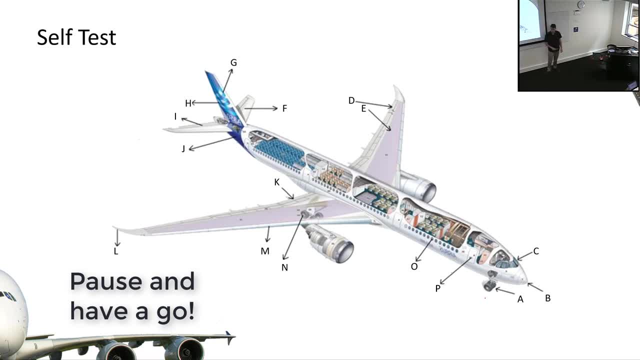 Put an ABCD or whatever next to all of those things that you've taken down. So hopefully I don't expect you to know all of these, but hopefully you know by now that the pointy end at the front we call the nose. 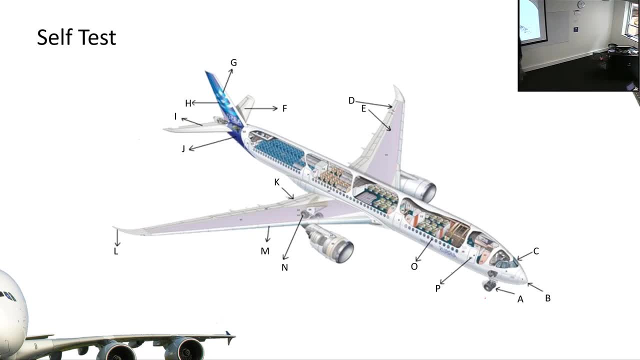 and the bit at the back we call the tail, And we have a couple of wings here and a couple of engines hanging off those wings, so I haven't really bothered too much with those kind of labels. We have landing gear underneath which we can have some labels for in a minute. 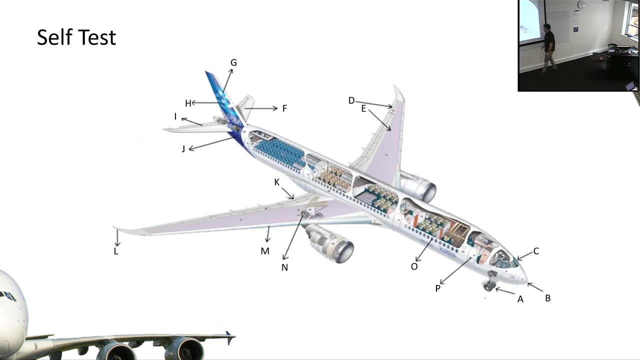 But then it gets a little bit more nuanced about what everything else is called. So let's go through A. Anyone want to volunteer their answer? Nose landing gear. yes, It's the landing gear that's in the nose, which is good. 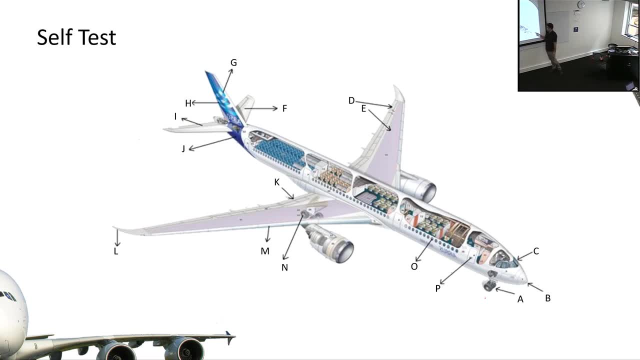 B- This one's easy Nose. yes, The pointy bit at the front. C- Cockpit- yes, It's where the people who break our aircraft sit. D- Ailerons- yes, So ailerons, control what. 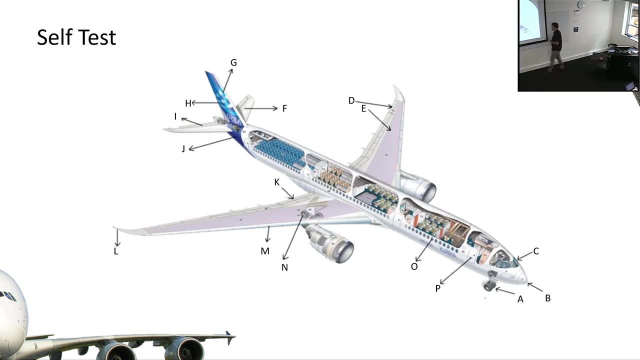 The role of the aircraft. yes, So we'll talk a bit about coordinates in a minute. but we have different attitudes and different control of those attitudes in the aircraft. Generally we treat the aircraft as an orthogonal system where we have a vector that's pointing forward. 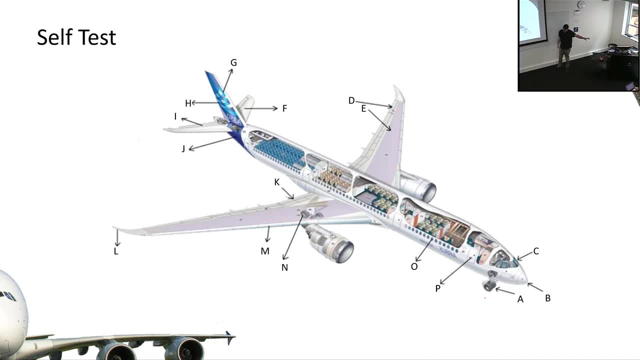 a vector that's pointing out one wing and a vector that's pointing down And we say fore-aft is going sort of forwards to backwards and then we have inboard and outboard is going sideways and I can't remember the vertical up and down. 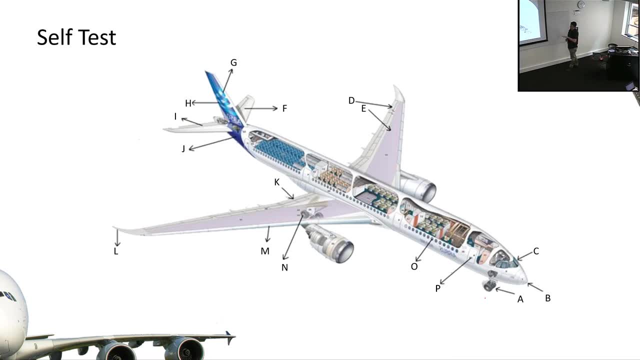 because we don't use it very often, But changes in attitude relative to those coordinates. if we roll about the longitudinal axis, we pitch about the transverse axis and we yaw about the vertical axis. So ailerons control roll. Now E wing, it's nice and easy. 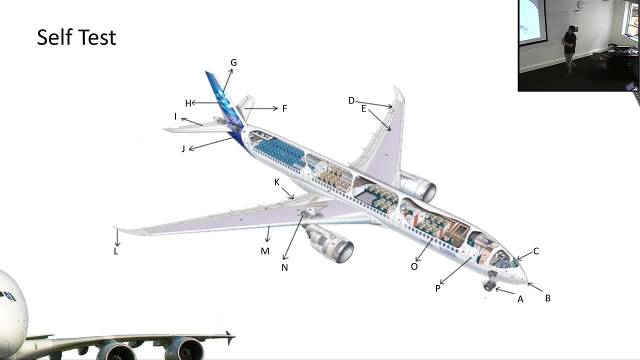 F. okay, we've got a couple of, So it's a horizontal stabilizer. We'll get to elevator in a minute. Horizontal tail horizontal stabilizer: they're both the same meaning They provide stability, which is in the name. 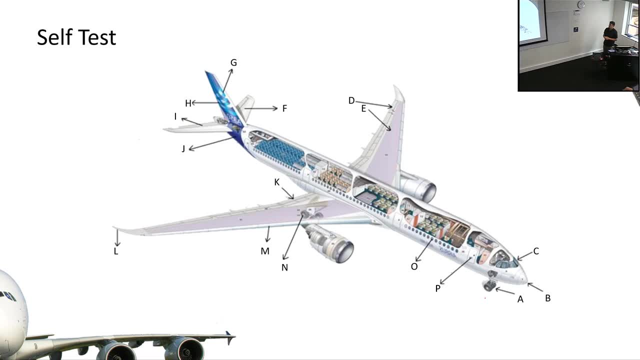 stabilizer. They stabilize the pitch of the aircraft. Okay, so if you tried to deviate from the pitch that you have, they would restore and stabilize. They don't control pitch, but they stabilize pitch. G- Vertical stabilizer- Vertical stabilizer and the vertical stabilizer controls yaw. 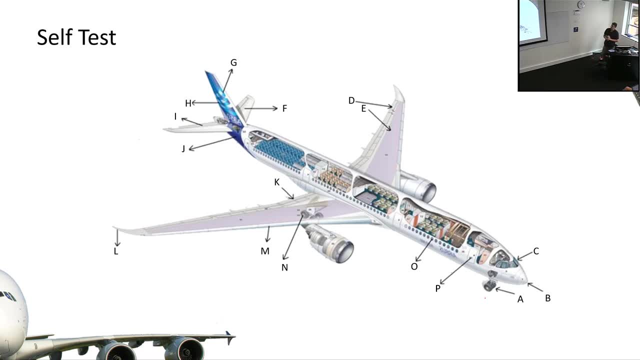 Sorry, stabilizes yaw H Rudder. Rudder Now the rudder controls yaw Now, as you'll find out in the course as you go along, it's not that simplistic Once you put the rudder on or any of the controls. 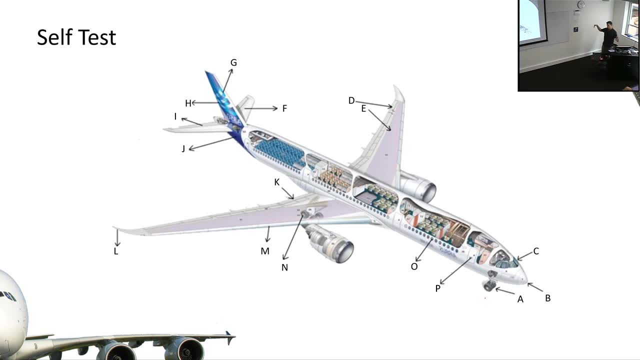 you get extra reactions. So if you put the ailerons down, you don't just roll, you also yaw at the same time, because you generate drag. So there's complex interactions here. but to the first pass, the rudder controls yaw. 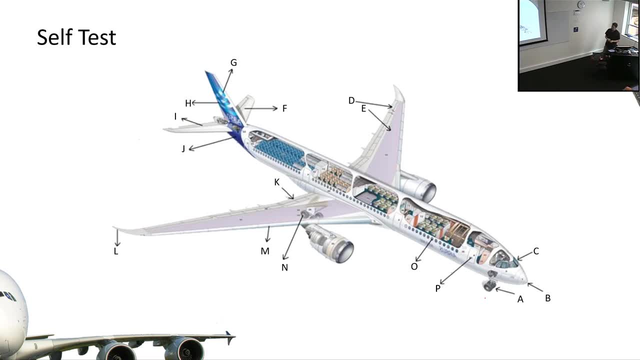 I Elevator, Elevator. It controls pitch, sort of. Actually it doesn't really control pitch, It primarily controls your airspeed. but that's not my course's job to teach you about that, J Empennage. 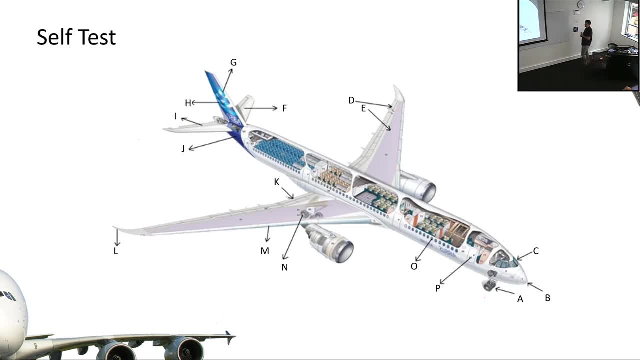 Empennage. yes, It's one that sort of people get to the end and go. what the hell is that? It's the only one left. The empennage is pretty much- it's another French-sounding word- for anything- rear of the rear pressure bulkhead. 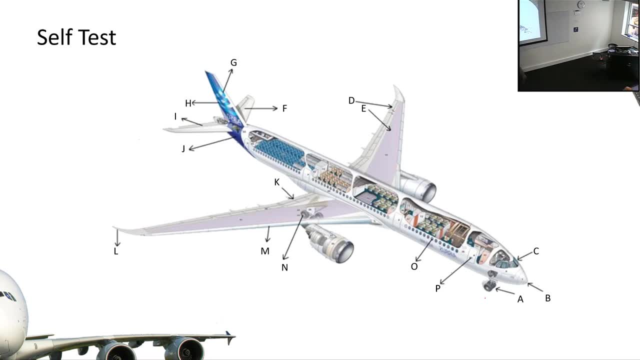 So lots of aircraft have these tapering tails. So anything in what we would call the tail structure, we call the empennage K Flaps, Flaps, yeah. So high-lift devices generally live inboard. 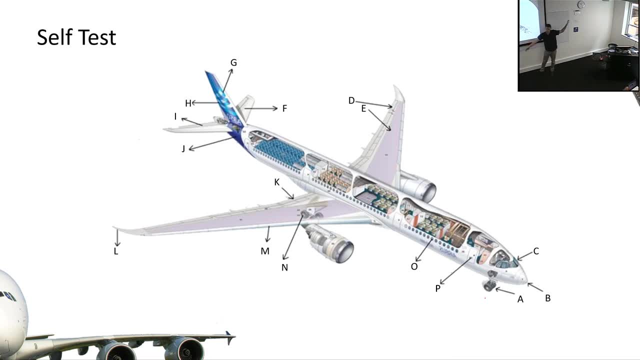 So ailerons live outboard generally so that you can control the aircraft. You need a lot of moment so that you can actually provide that control. Flaps and high-lift devices generally live inboard, because then it generates less moment on the wings. 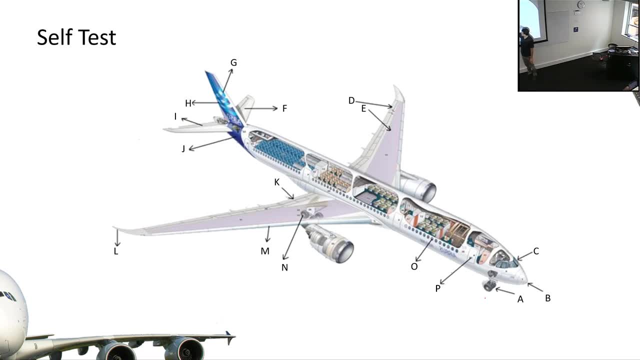 This is depending on the aircraft. Some aircraft have what are called flapperons, which are actually flaps and ailerons together, so you can have the surfaces do both. Generally flaps are deployed downwards together to generate more lift, but if they also have independent control, 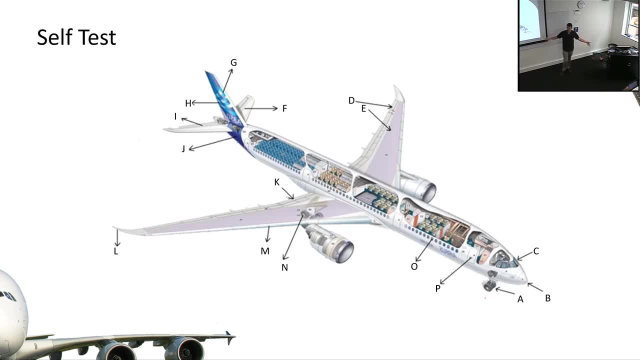 they can be deployed downwards and differentially applied, which gives us the ability to control roll. So if they're both just down together, they're generating just lift. If you can then differentially control them, you can roll them as well. 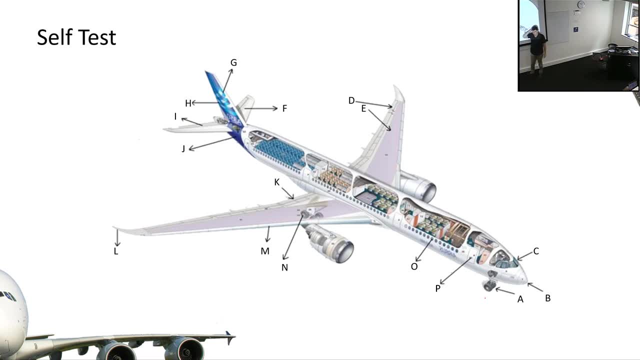 Most high-speed aircraft, so things travelling close to sort of Mach 0.8, 0.9,, which is most of our airliners, will have outboard ailerons out here and they'll also have flapperons inboard. 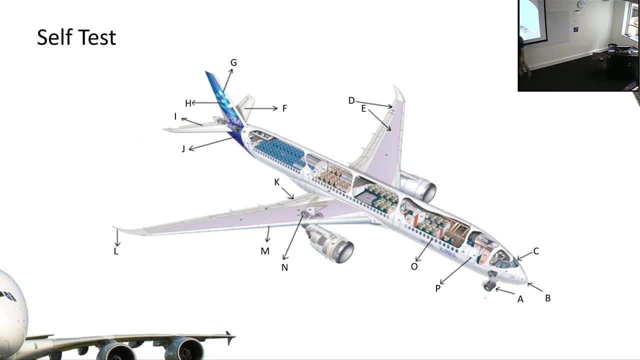 So at high speed you lock these out so they can't move and all of your roll control is done with the inboard, Because, just like if you're flying down the freeway at 150 kilometres an hour and you very quickly turn your steering wheel, 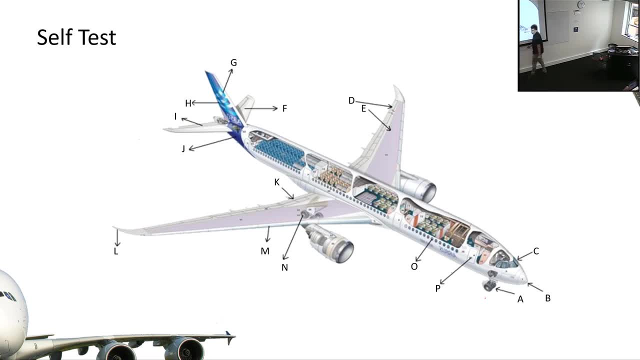 it wouldn't be a very easy vehicle to control. you need precise control at speed, which is why they have inboard ailerons and at low speeds they'll have outboard ailerons. Where are we up to L? 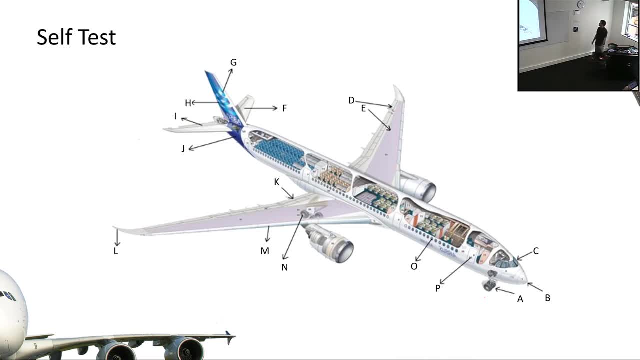 Wing tip. yes, So we talk about the wing tip and then we talk about the ailerons And the wing root. So the root is where it attaches to the fuselage and the tip is where it points out into space. 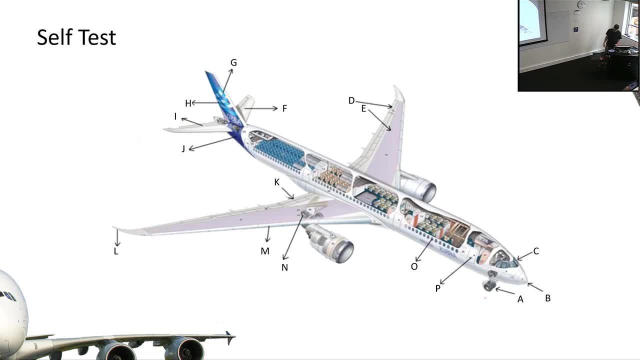 M Leading edge. So leading edge is at the front, trailing edge is at the back, N Main landing gear, O, Fuselage And P. we finish on a high note Door, yes, Cabin door, Of which there are generally a few. 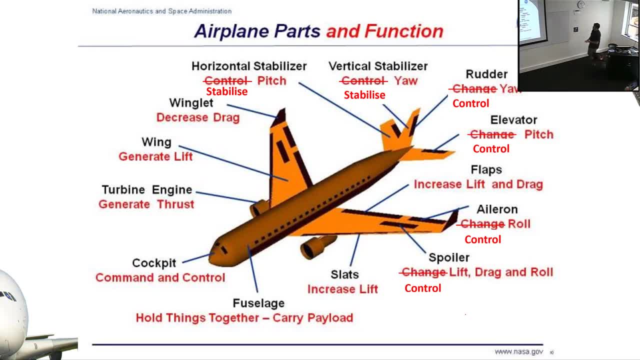 All right, Now this diagram I'll leave you to review, because there's a lot of text on it And this is a NASA diagram, but I disagree with NASA completely on some of these, so I've crossed them out So, because they're just flat out wrong. 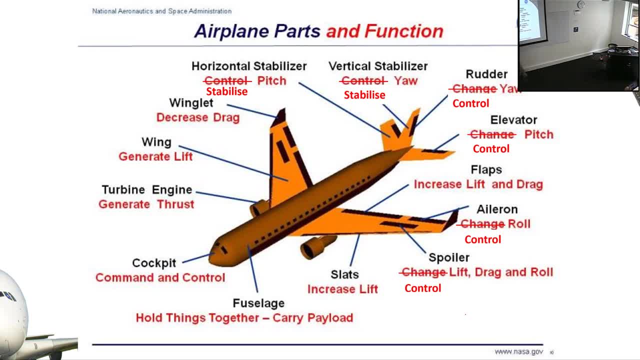 The horizontal stabilizer, as it says in the name, stabilizes pitch and the rudder controls your. so they've just used the wrong verbs, But other than that they're pretty good. But I'll leave you to review that by yourself. 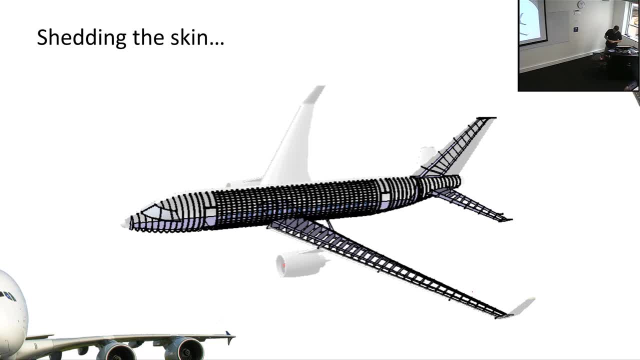 Once you take the skin off, you can get these cutaway diagrams. This is something that you can by the end of your aero degree. here, your aero design groups will be generating something like this. This is actually a CATIA drawing. 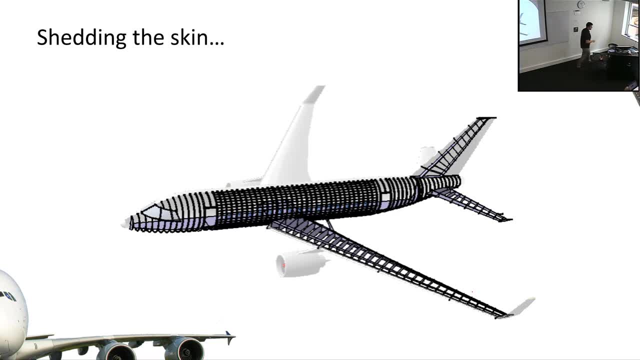 from my aerospace design project here. It's in fourth year. I didn't build this, someone else in the team did, But we need to get to the point, from now until two years from here, where you're skilled enough as engineers to be generating these kind of layout diagrams. 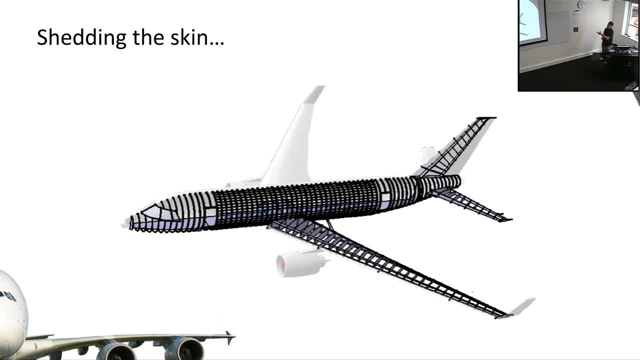 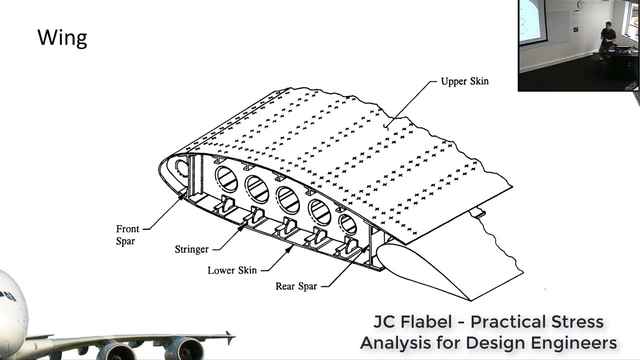 for an aircraft and knowing not necessarily the details of the size and shape of every component, but how to lay it out and why it's laid out in that configuration. A bit of terminology. We're really quickly running out of time. But inside a wing we have our skins. on the outside, 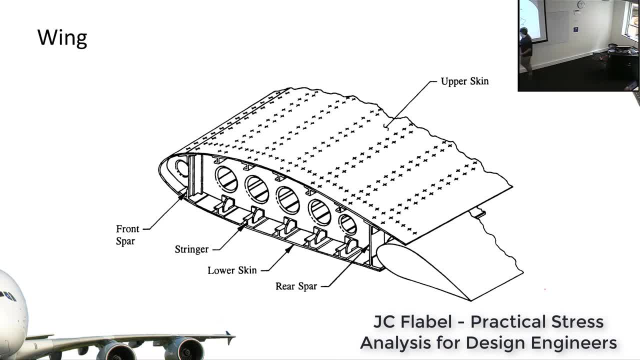 We have control surfaces on the back ailerons. Stringers are the longitudinal stiffening members. We have spars of these vertical members inside that are carrying bending moments. We have a rear spar and a front spar. Generally we'll have two. 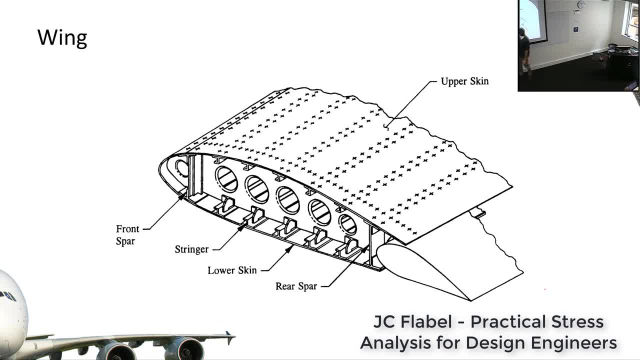 Sometimes we'll have more, And we have spar webs, which are the vertical parts here, and spar caps, which are the tops and bottoms, Primarily all the skin at the top and bottom and the stiffening members is what's carrying the bending moments.